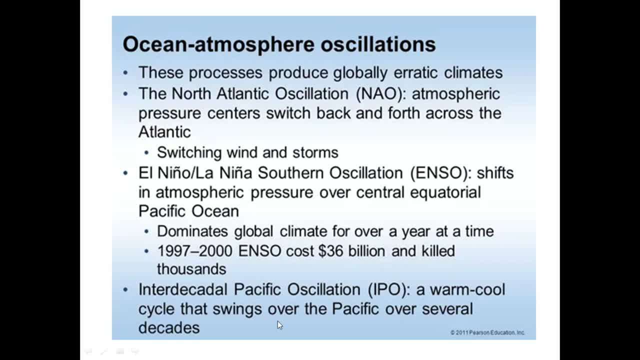 considered the IPO to be kind of like a $100,000.. And then there may be other ones, like the Arctic Oscillation, which tends to work closely with the North Atlantic Oscillation, And then there's the Atlantic Multi-Decadal Oscillation. 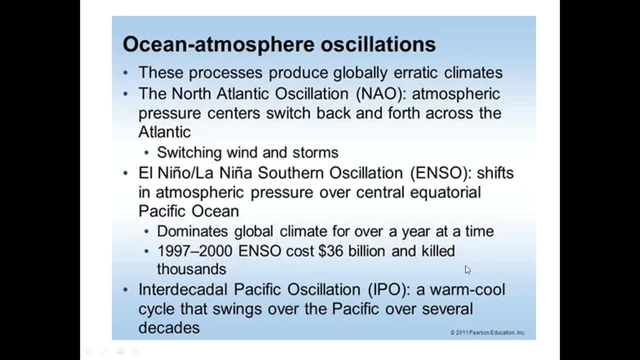 the AMO, And again, that's sort of like the answer to ENSO, but on the Atlantic continent. And we have another one as well: the Arctic Oscillation, which tends to work closely with the North Atlantic Oscillation, And then there's also the Atlantic Multi-Decadal Oscillation, and 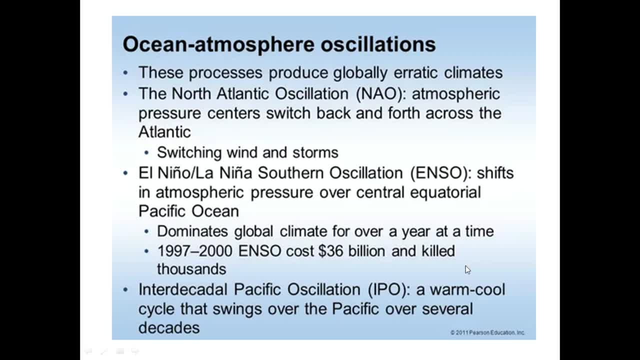 Atlantic side, and there's two more recently identified cycles, one called the Indian Ocean Dipole, another one called the Arctic Dipole, and over the course of several videos, I'm going to be discussing every single one of these. This video will be dedicated to discussing ENSO. 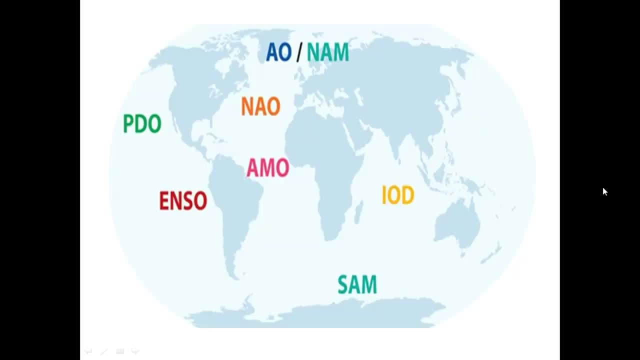 So here we have. this is the Arctic Oscillation, something called the NAM, and then there's a counterpoint, the SAM down in the around Antarctica. I will not be discussing SAM. Here is the North Atlantic Oscillation, the Atlantic Multi-Decadal ENSO, the PDO, and then here's the IOD Over the Arctic Oscillation, the Arctic Multi-Decadal ENSO, the PDO, and then here's the IOD Over the Arctic Oscillation, the Atlantic Multi-Decadal ENSO, the PDO, and then here's the IOD. 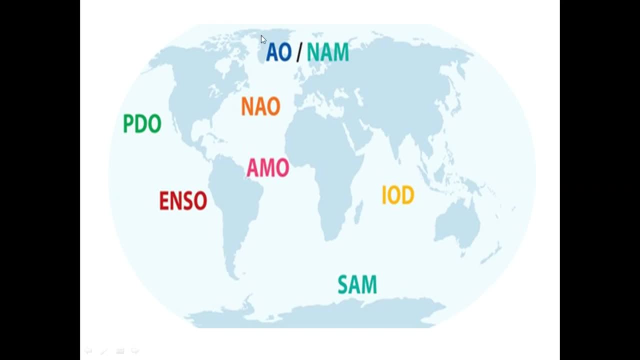 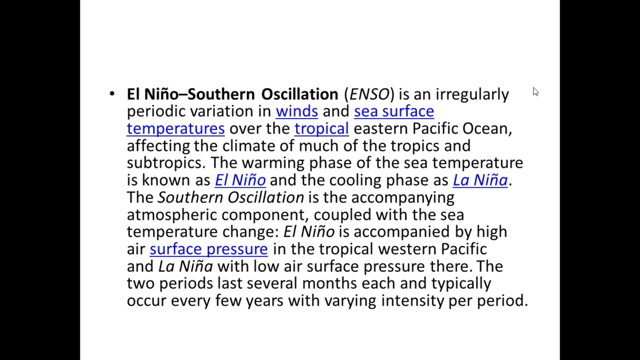 Over here about going to the Russia side. it would be the Arctic Dipole. I'm going to be discussing each one of these over the next several videos. Okay, so let's get going. ENSO El Nino, Southern Oscillation, and it's a little description. some background information. 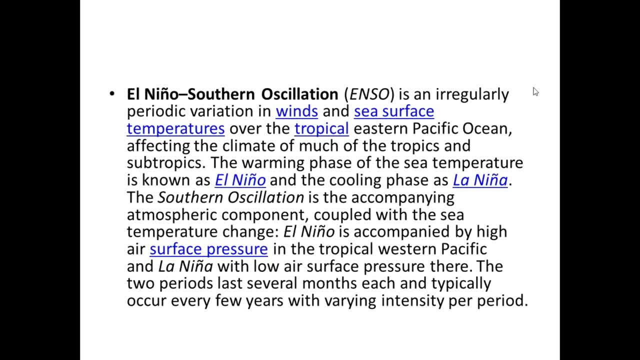 It's a regularly periodic variation in winds and sea surface temperature over the tropical Eastern Pacific Ocean affecting the climate. It's a regularly periodic variation in winds and sea surface temperature over the tropical Eastern Pacific Ocean affecting the climate. It's a regularly periodic variation in winds and sea surface temperature over the tropical 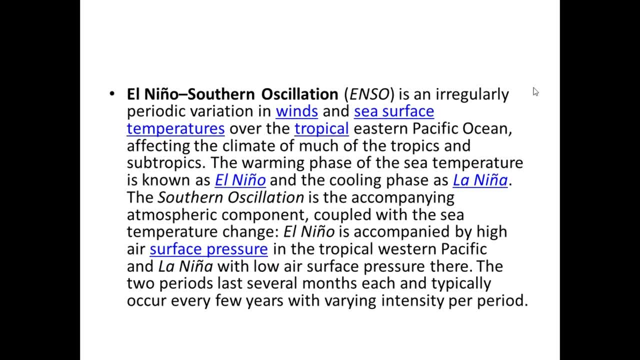 Eastern Pacific Ocean, affecting the climate Much of the tropics and subtropics. the warming phase of the sea temperature is known as El Nino. The cooling phase is La Nina. Now, the reason why it was called El Nino is that off the coast of South America, the 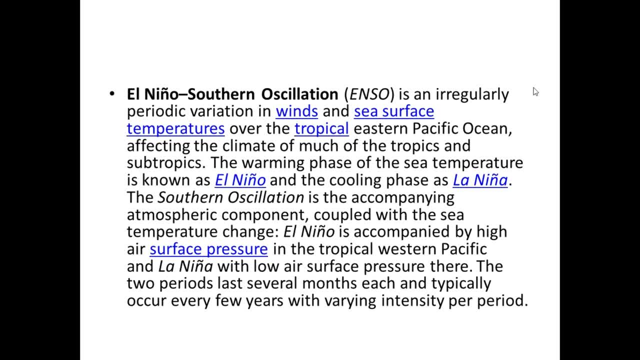 western coast of South America, which would be the eastern side of the Pacific Ocean. Peruvian farmers would notice that every seven or so years, plus or minus, their anchovy catch, how much anchovies they caught and fished fish would drop, And this seemed to occur around the time of Christmas. That's why they call it. 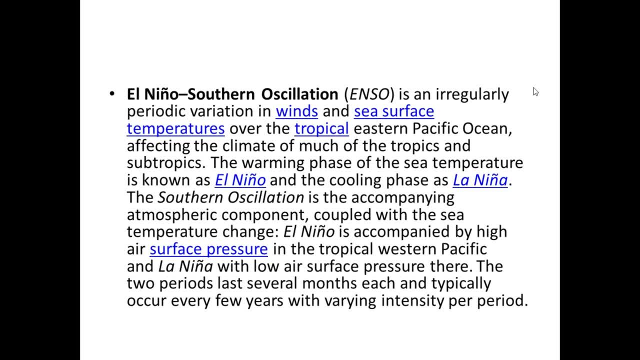 El Nino referring to, because El Nino is the boy or the boy child, And so it was a reference to the fact that this phenomenon seemed to occur around Christmas, almost like once a decade, plus or minus a little less. So that's where, that's how the name came about. 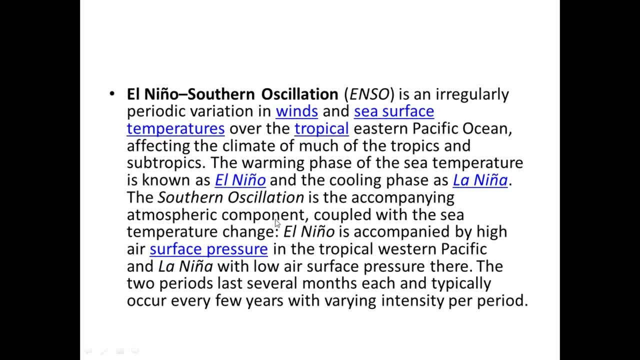 The Southern Oscillation is an accompanying atmospheric component, So El Nino, La Nina, refer to sea temperature, sea surface temperatures to be a little more accurate, And Southern Oscillation refers to what's happening, to the high and low pressure systems in the atmosphere. 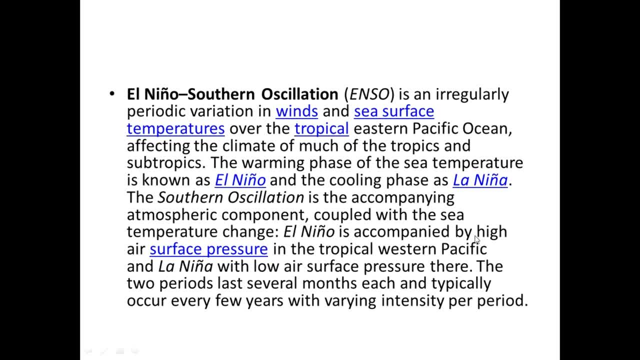 And then that couples with the sea temperature change. El Nino is accompanied by high air surface pressure in the tropical western Pacific, La Nina with low air surface pressure at the same level. The two periods last several months each and typically occur every few years, with varying 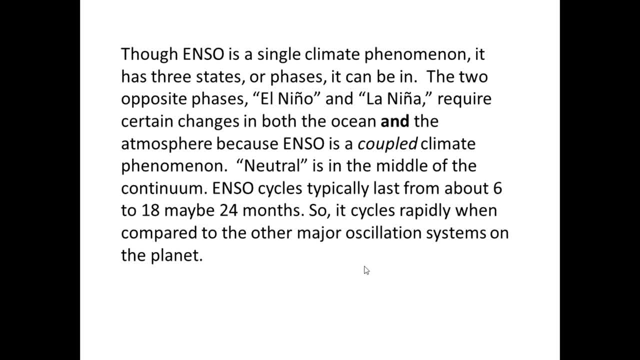 intensity. It's actually in three states. It's commonly thought of as a single state climate phenomenon. It's actually in three states. You've got the opposite phases of El Nino: La Nina, which requires certain changes in the ocean and the atmosphere because it is a couple climate. 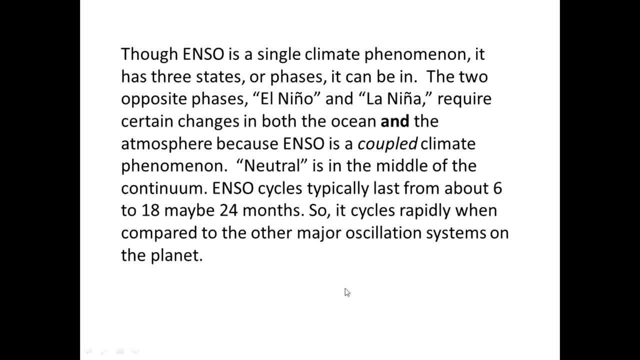 phenomena, And the neutral is basically what you get in between. So when it goes from El Nino to La Nina, it goes through a neutral phase And then, on the way back from La Nina to El Nino, again goes through a neutral phase, And so cycles typically last from about six. 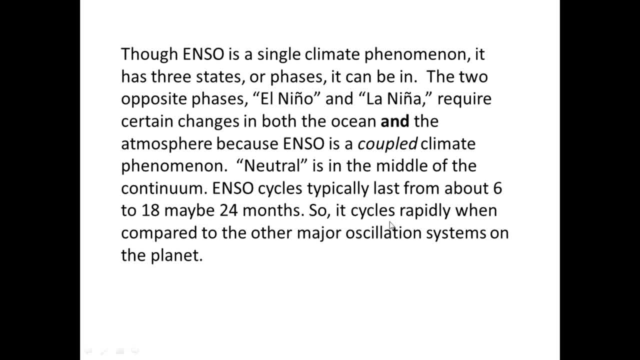 to maybe 24 months, But the cycle varies rapidly when compared to other oscillating systems on the planet. Now it cycles on that route, But when you get the strong El Nino or the strong La Nina, that's when you start getting the strong El Nino And that's when you start. 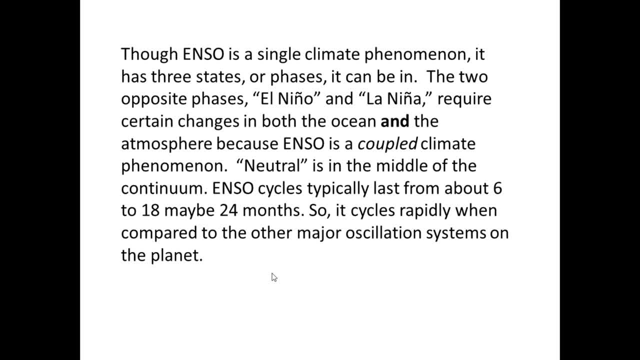 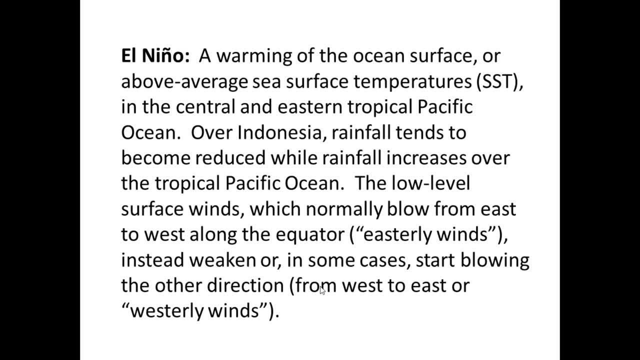 getting into about the five to 10-year cycle. Okay, El Nino is the warming of the ocean surface or above average sea surface temperatures, hence referred to as SST, in the central and eastern tropical Pacific Ocean. Over Indonesia, rainfall tends to become reduced, while rainfall increases over the tropical Pacific Ocean. 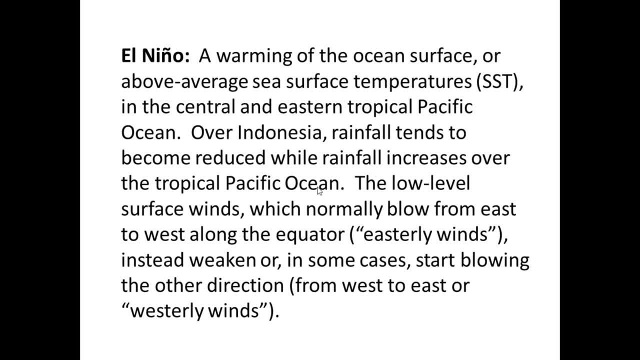 The low-level surface winds which normally blow from east to west along the equator. easterly winds weaken or, in some cases, actually blow from west to east, become westerlies And when you have wind blowing, the wind is also pushing on. 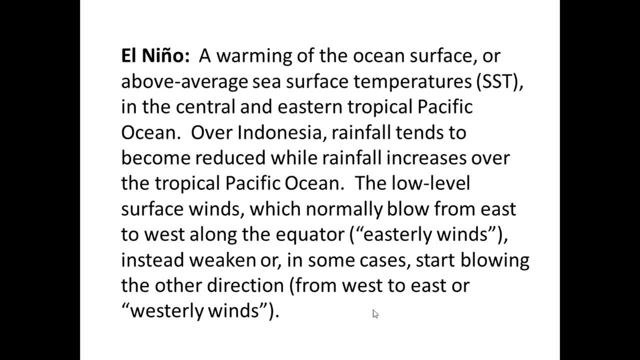 the ocean surface. We call that wind stress, And as it pushes on the wind, it's going to cause the water to pile up at the end of where the wind stops blowing. That is a critical component of what happens with ENSO. 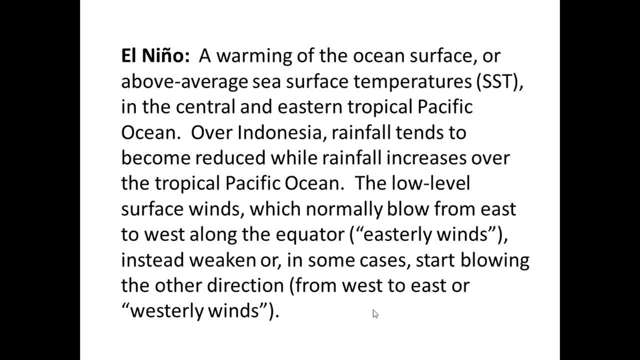 In fact, for many years, oceanographers did their things, atmospheric scientists did their thing, and it wasn't until in the last several decades that I said: hmm, it's really a couple system and we need to start collaborating more. so Because, no matter how you look at it, 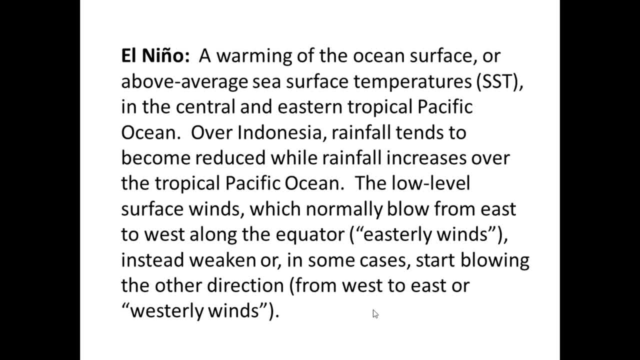 whether it's the atmosphere or the ocean, they're both considered to be fluids. Now, I say fluids, not liquids, So they behave like fluids, the difference being the internal viscosity and density. Viscosity is a little bit different, but it's a little bit different. 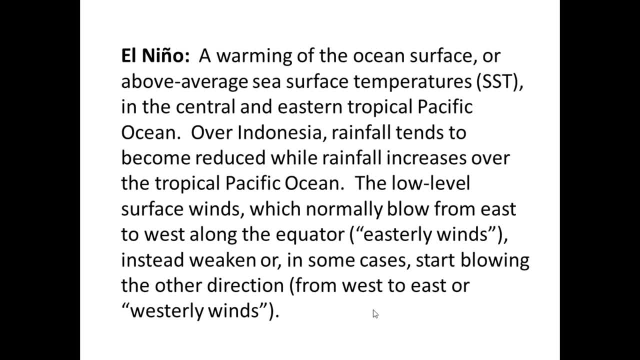 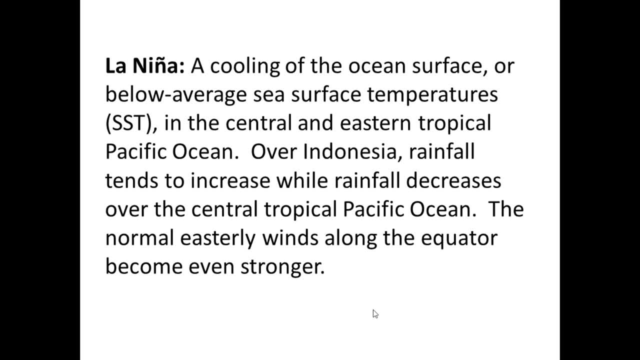 It's a measure of a fluid's internal friction, So La Nina is a cooling of the ocean surface or below average sea surface temperatures in the central and eastern tropical Pacific, Over Indonesia rainfall tends to increase, while rainfall decreases over the central tropical Pacific Ocean. The normal easterly 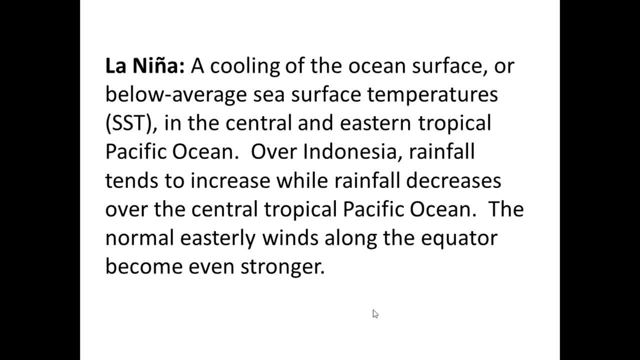 winds along the equator become stronger. So for folks who live, say, in Indonesia, Australia, that area, when La Nina is in place, it's a cooling of the ocean surface or below average sea surface temperatures. So La Nina is in place, you're going to get rained on a lot. 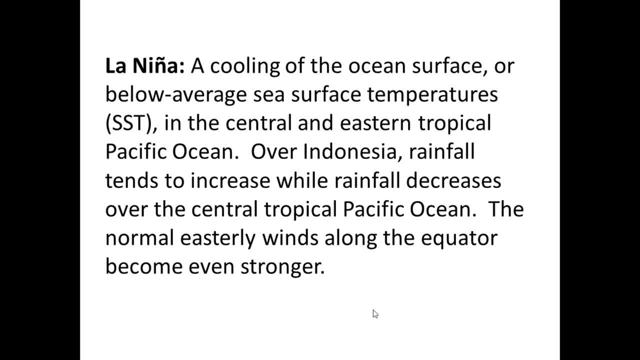 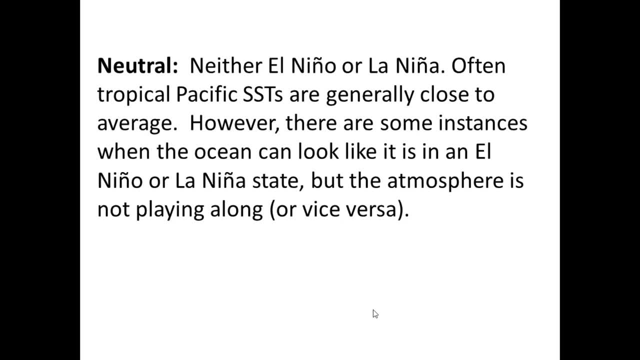 more. When El Nino is in place, you're going to see very little precipitation. You might see some dry and drought conditions, Neutral, Neither, or Often tropical. Pacific SSTs are generally close to average. Some instances it may look like it's in one or the other. 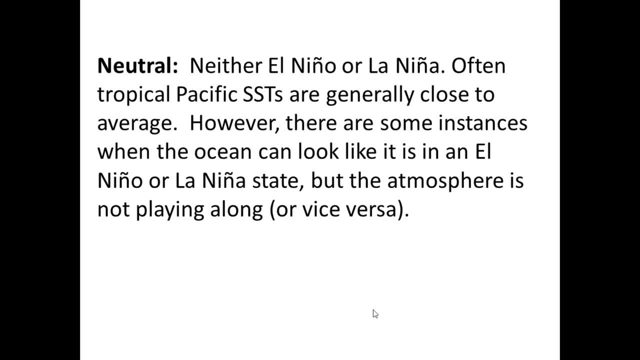 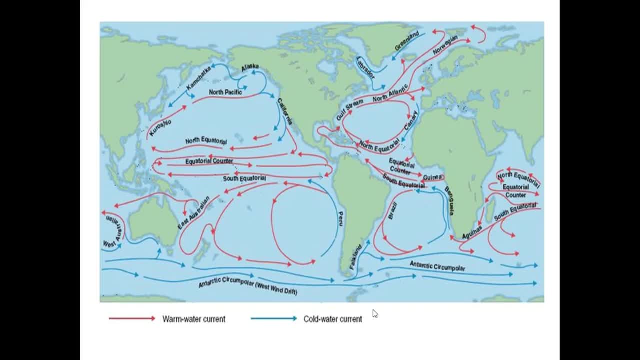 state, but the atmosphere is not playing along. Kind of I'm going to put a little fun on it. Okay, Now this here, this graphic is simply showing the major ocean surface currents on the planet. Okay, And you know, for example, here's the Gulf Stream, right Becoming the 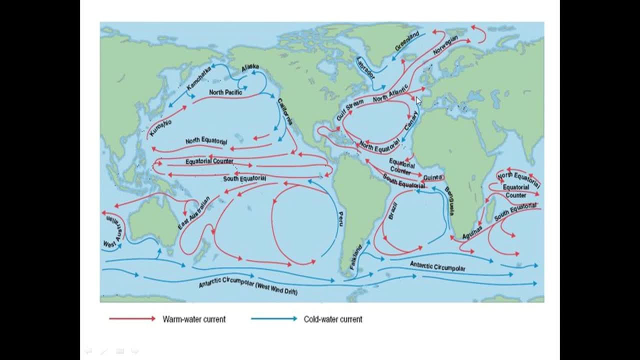 northward drift, right North Atlantic drift. Then we have, you know, the Canary Return Island. So this is a nice gyra system here. You have a north equatorial current in the Atlantic side, Then you have a counter current which goes against, And then you have similar things. 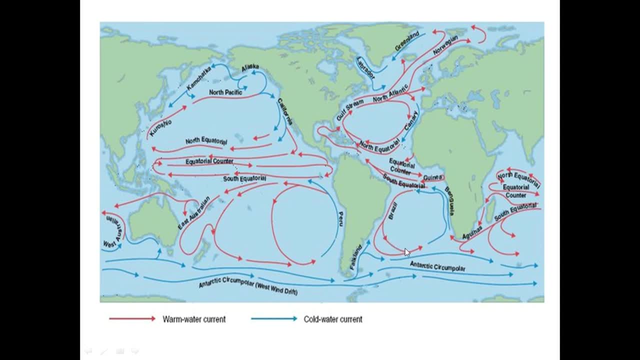 in the South Atlantic. The arrows indicate the direction of flow. The fuchsia or magenta colored are warm water. The blue are cold water currents. Here's the Antarctic Circumpolar, something called the West Wind Drift. This is where it totally rings around Antarctica. 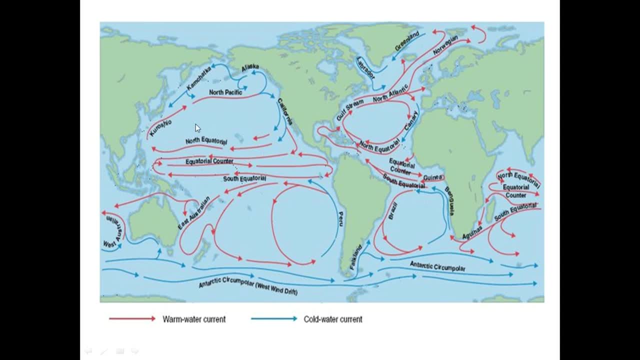 It goes all the way around On the Pacific. here is the nice northern North Pacific gyra. You have a little cold water gyra that rotates in the opposite direction. Little later on I'll be explaining about gyras and cyclones and so forth, But let's. 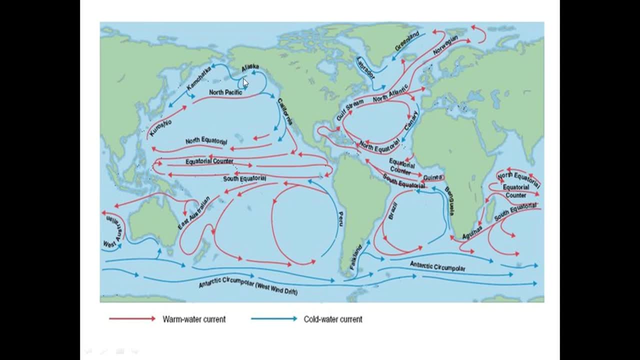 just state for now that because the gyra in the Gulf of Alaska rotates in a counterclockwise manner is a reason why this region is very productive in fisheries, Because you have a nice upwelling in the middle of the ocean. So you have a nice upwelling in the middle. 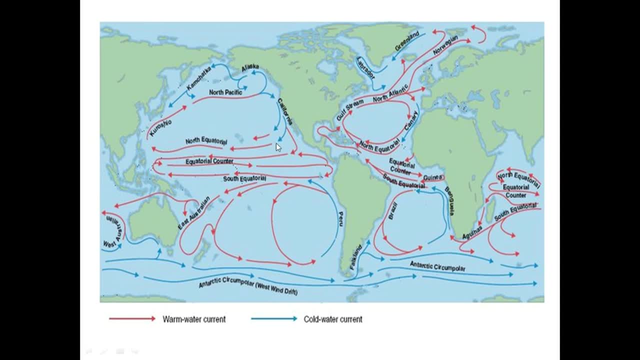 of this bringing loads of nutrients. So here you have the equatorial, the south equatorial current, the north equatorial current. In between is the equatorial counter current. It is these three major currents that, when they go, which way they're blowing, how strong they're flowing, is what ENSO will be affecting. 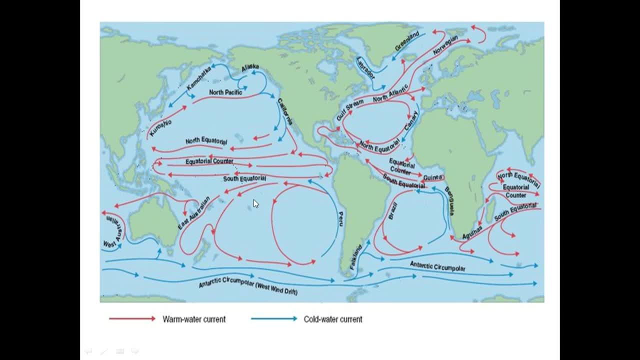 And then we have sort of like a double gyro system in the south Pacific. When the north equatorial hits about the Indonesia region, it actually bifurcates and you have part of what's called the Kuroshio current, which goes alongside Japan, And then you have another current that flows down this way towards the 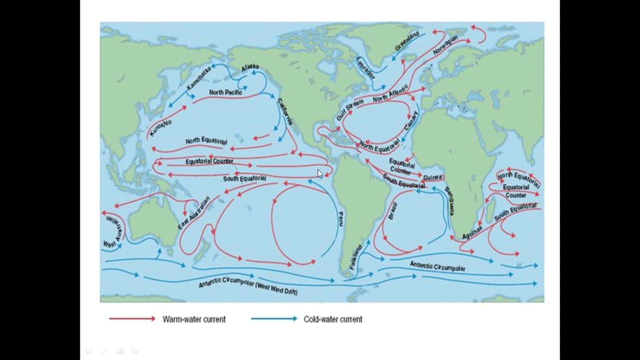 Australia side of things. So I just wanted to point this out. You've got here the major oceanic currents, surface currents, So these are all horizontal flowing. This does not indicate any vertical currents like thermohaline or anything like that. And then you've got 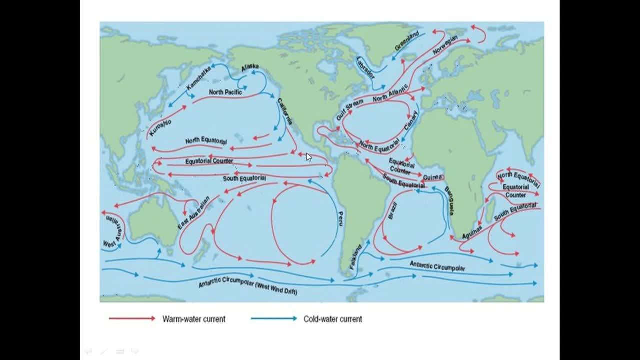 a few in the Indian Ocean, et cetera. So I want to you know, just so you can have an idea of when we start talking about the currents. you can always refer back to this figure to get your bearings. But this is to kind of give you an orientation. So here is from December 1988.. This is a satellite. 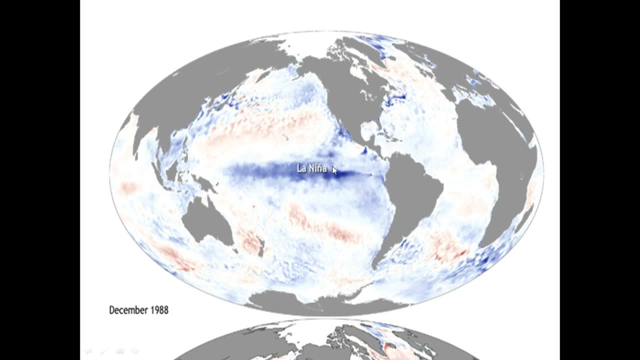 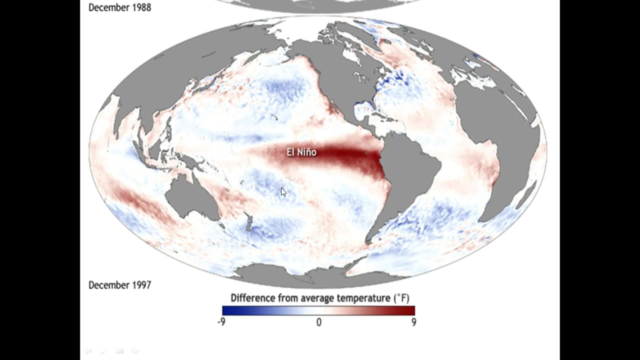 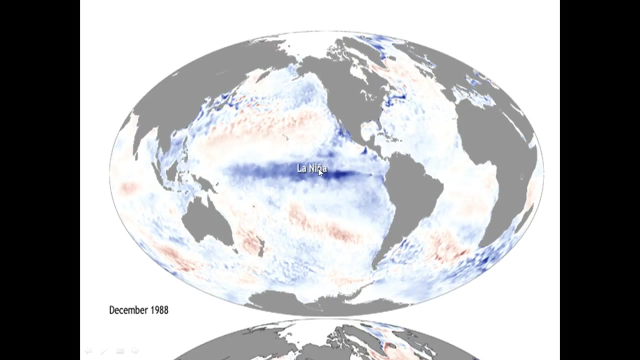 imagery of sea surface temperatures And you can see very cool conditions. in the eastern Pacific equatorial region We have La Niña, And there it is a year before. So this is December 1988.. This is the year before December, Oh, actually the year before. 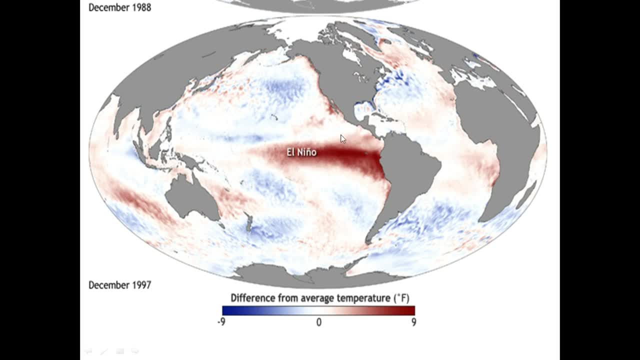 This is 1997.. So nine years later, a very strong El Niño. So what you see here, and just so you understand the temperature scale, this is the difference from average temperature. So when you see white doesn't mean there was no reading, That means that all this is. 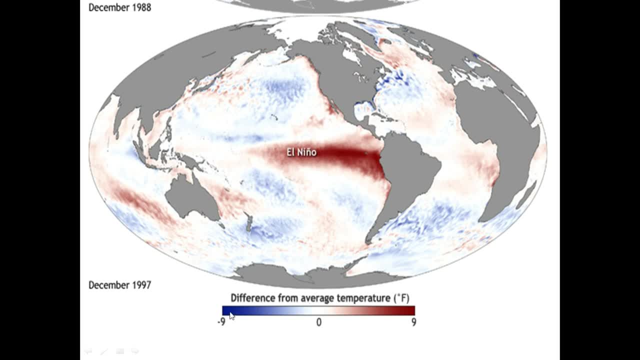 average temperature recorded. The darker blue it is, the colder it is, the more it deviated less than the average. Conversely, the more red it is, the colder it is. So you can see that Say a hot water, a cold water. This is when it deviated less than the average. 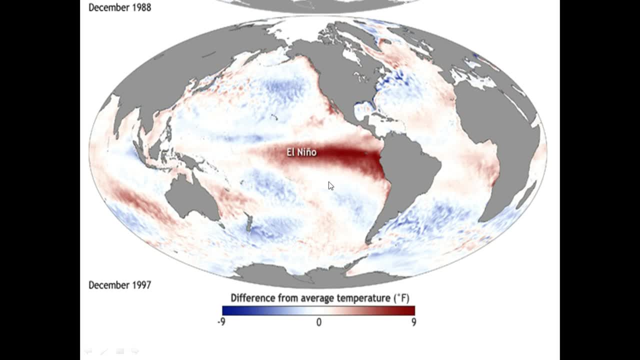 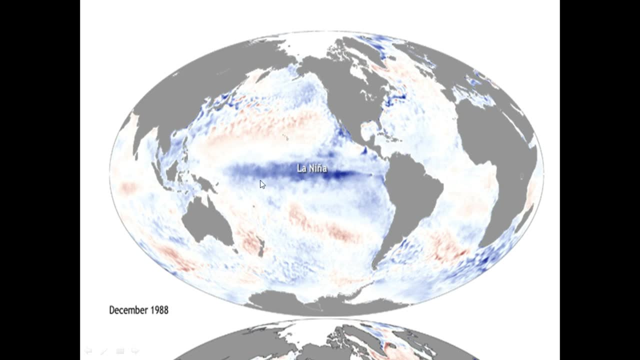 Conversely, the more red it is, the colder it is. So this is the difference. This is the the hotter it deviated from average. so this was really a lot colder than average. not so cold there. not so cold there. and this is really hot. not so hot, say there. i think you get the idea. 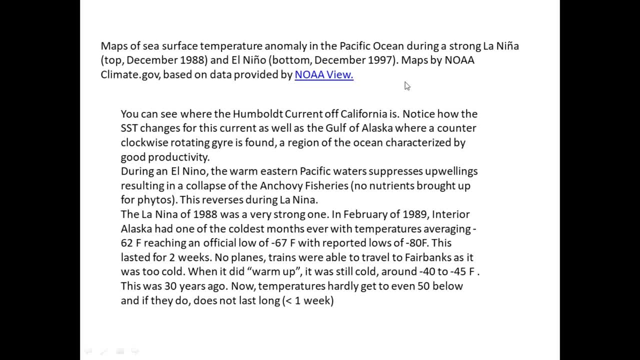 okay, and again that this describes the last two figures. i just showed you maps of sea surface temperature anomaly in the pacific ocean during a strong la nina and then a strong el nino, and i know you can see the humboldt current of california. notice how sea surface changes for 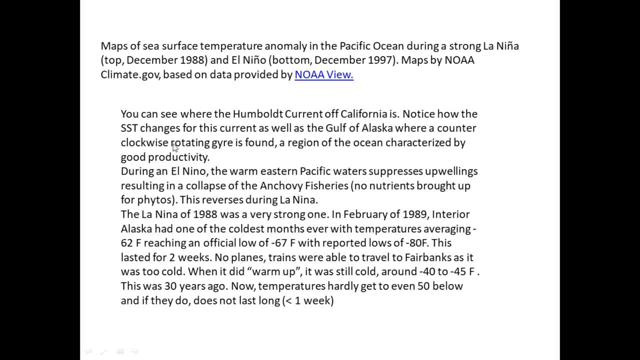 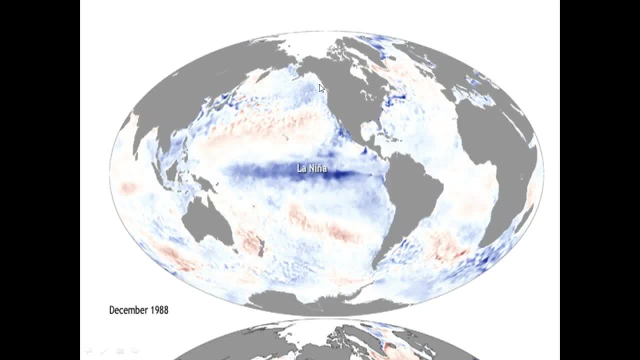 this current, as well as the gulf of alaska, where the counterclockwise rotating gyro is found, the region of the ocean characterized by good productivity. okay, right here, here's the humble current, and right down here here's the atlantic, uh, the alaska, uh, gulf of alaska, gyro, and again. 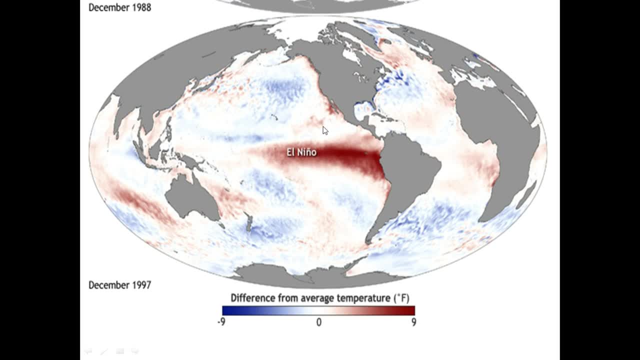 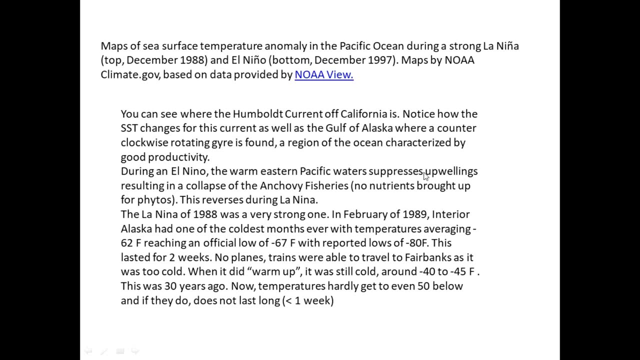 you can still see traces of the humble current coming down during el nino. the warm eastern pacific water suppresses upwelling, resulting in the collapse of the anchovy fisheries. no nutrients brought up. this reverses during la nina. the la nina of ada was a strong one. favor of 89. interior alaska had one of the coldest months ever. 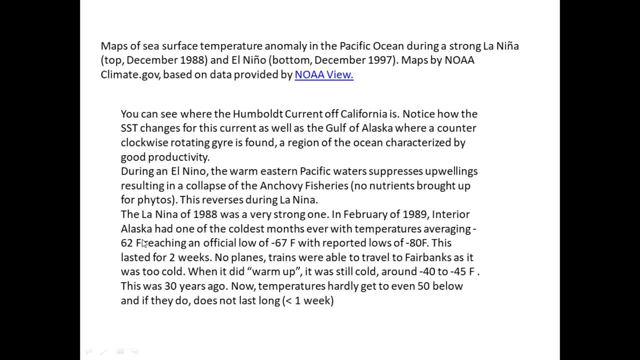 with temperatures averaging minus 62 degrees fahrenheit, reaching an official low of minus 67 fahrenheit, with reported lows of minus 80 fahrenheit. i was there, uh, at where i was living, it was minus 72 fahrenheit. this lasted for two weeks. no plane to trains were able to travel to fairbank. 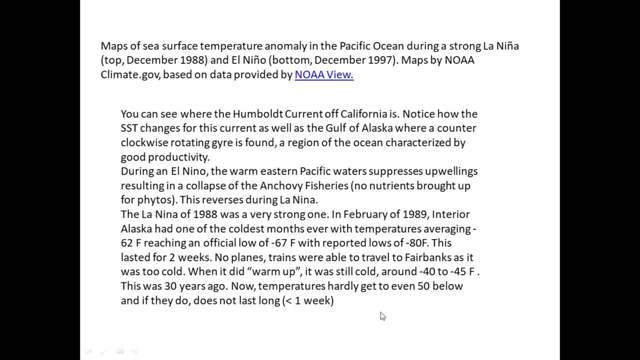 it was too cold. if you had a heating device that required fuel to operate, it didn't happen. basically, those who had wood stoves were very popular, because you can always get a wood stove going and when it did- quote unquote- warm up, it was still around minus 40 to minus 45 degrees fahrenheit. this is 30 years ago now. temperatures: 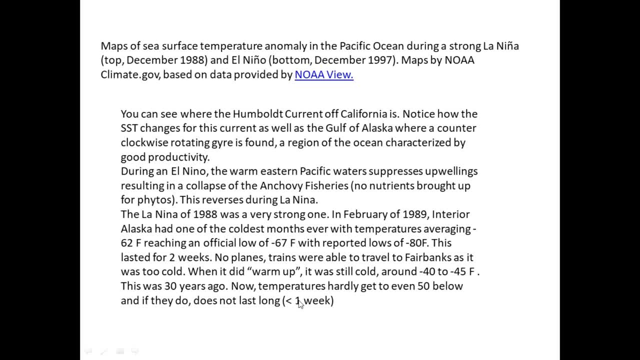 hardly get to even 50 below, and if they do, it does not last long, typically less than a week. this shows you how drastically things have changed here in the arctic due to climate change. but uh, yeah that, la nina, you know that lasted into 89. holy crap, was that cold. there was a brand new. 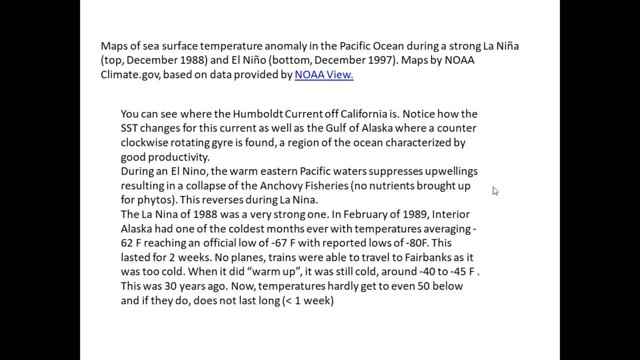 creature that was discovered. it was called the snow snake and it all these, uh, snow snakes were black. basically what it was was it got so cold that if anyone even was stupid enough to try to start their vehicle, the fan belts just snapped. they had contracted so much and gotten so brittle. 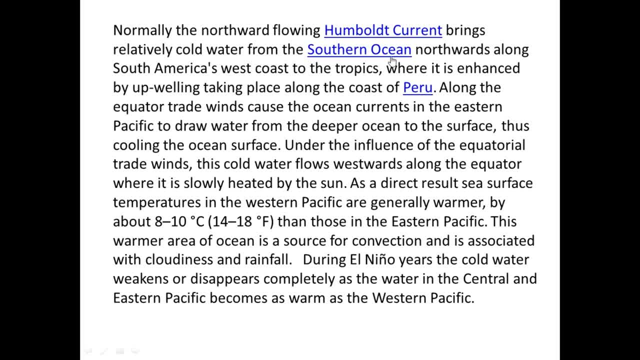 normally the north of flying humble current brings relatively cold water from the southern ocean, north of the long, uh south america's west coast to the tropics. it's kind of confusing. it's a there's a humble current in both the north and the south side, whereas enhanced by an upwelling taking place. 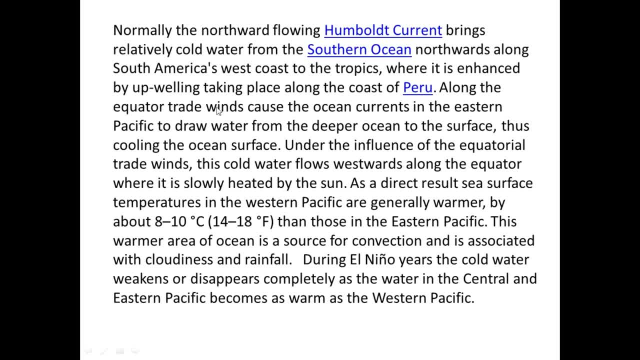 along the coast of peru. along the equator, trade winds cause the ocean currents in the eastern pacific to draw water from the deeper ocean to the surface. it's called a conservation of volume, which is what we call the ocean surface, and this will cool the ocean surface under the influence. 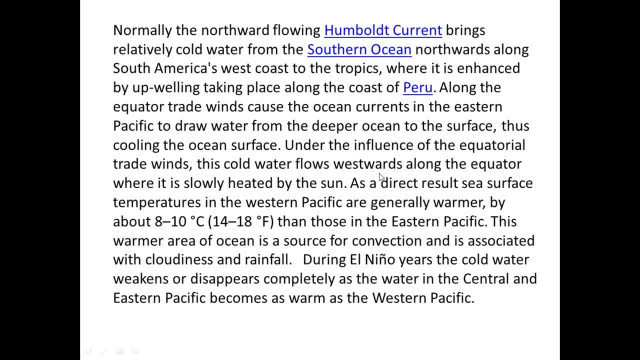 of the equatorial trade winds. as cold water flows westward along the equator, we're slowly heated by the sun. as a direct result, sea surface temperatures in western pacific are generally warmer by about eight to ten degrees c than those in the eastern pacific. this warmer area of ocean is a source for 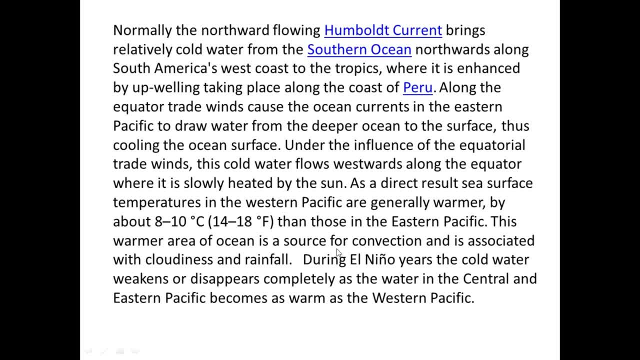 convection, ie atmospheric cells, and associated with cloudiness and rainfall years, the cold water weakens or disappears completely as the water in the central and eastern pacific becomes as warm as the western pacific, and i'll show you graphics on this later. all right, and so it's a nice catch-all acronym for all three states. 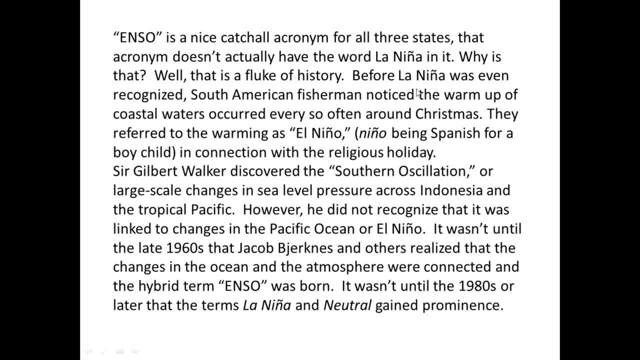 and why doesn't have the la nina in it? uh, that's because la nina was before it was even recognized. this is what i referred to earlier about el nino occurring around the christmas holidays. sir gibble walker discovered the sudden oscillation or large-scale changes in sea level atmospheric pressure across indonesia and the tropical pacific. 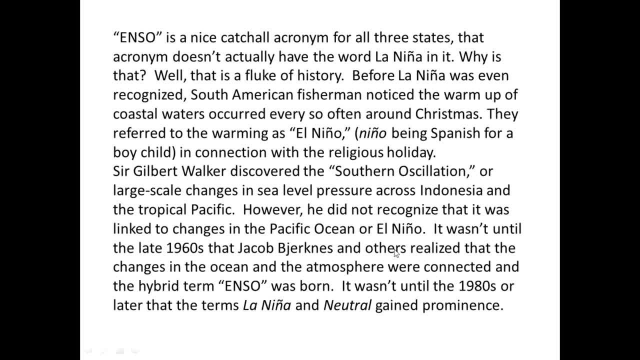 he did not realize that was linked to changes in in the pacific ocean or el nino. it wasn't until the late 1960s that jacob major knees and others uh realized that the changes in the ocean and the atmosphere were connected to the ocean and the atmosphere were connected to the ocean and the 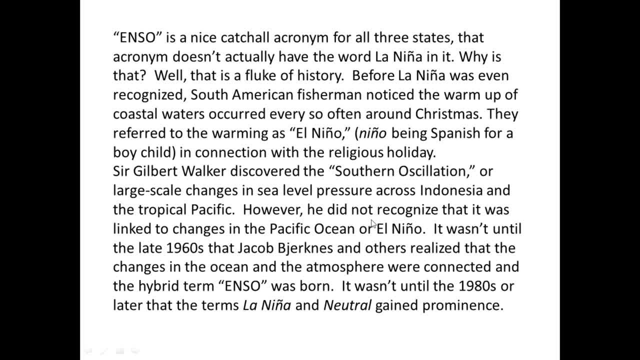 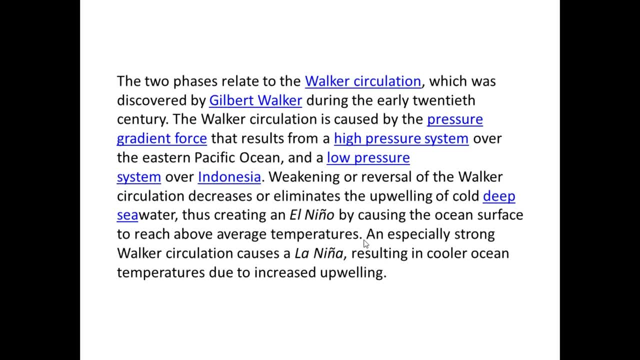 ocean and the atmosphere were connected to the ocean and the atmosphere were connected to the ocean and the atmosphere were connected and we got the and so term. the two phases related to walker circulation is discovered by gilbert walker during the early 20th century. the walk, the. 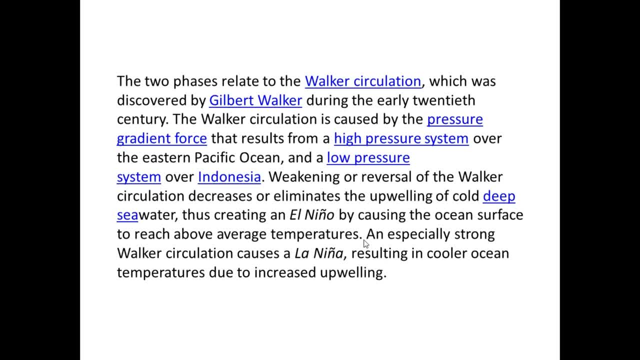 circulation is caused by the pressure gradient force that results from high pressure system over the eastern pacific and a low pressure system over indonesia. okay, what's meant by a gradient? if, if i have one area higher, higher air pressure or higher, let's say, and it's lower in another region, the tendency, you have a difference, so the 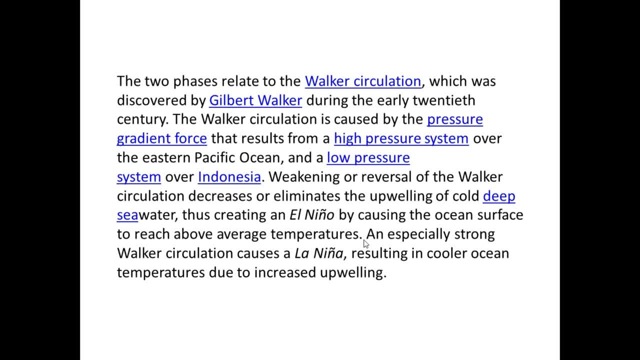 tendency is to flow from high to low and the air is going to move in that direction. think of if i open up a can of rancid whatever and i stick it in the corner of a room, what happens to people at the other corner of the room. you know, at the opposite end of the room, eventually you're going to smell it. 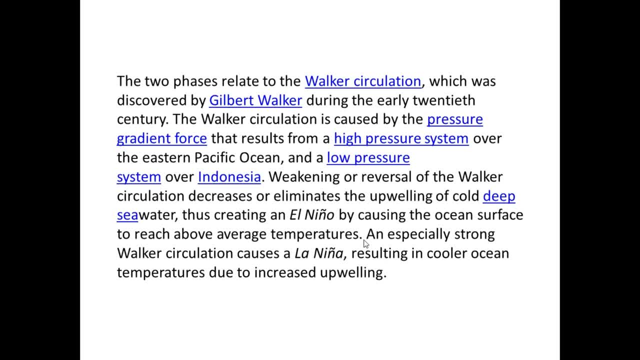 why is that? because the molecules which were high concentration where i opened up the can initially, they start to disperse to the section of the room where the concentration is less. it's that idea, the weakening or reversing a reversal of the water, circulatory decreases, eliminates the upwelling of cold deep sea water, thus creating an alemio, by causing the ocean. 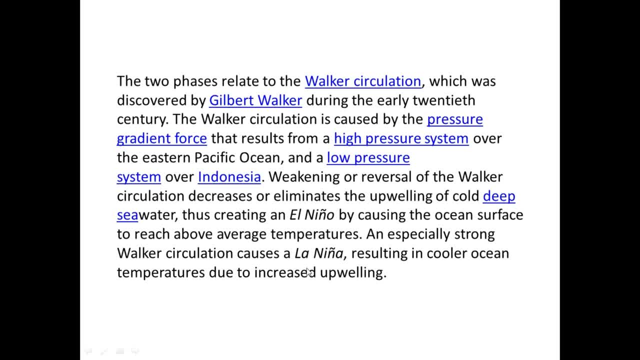 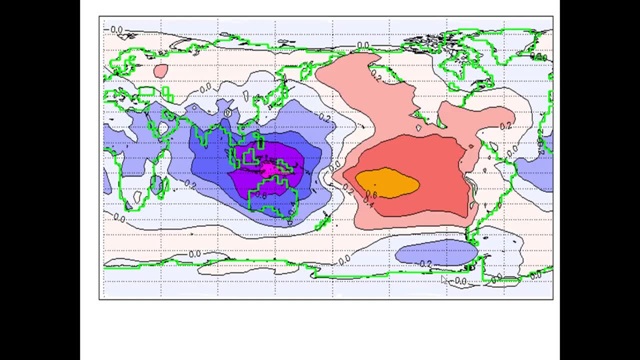 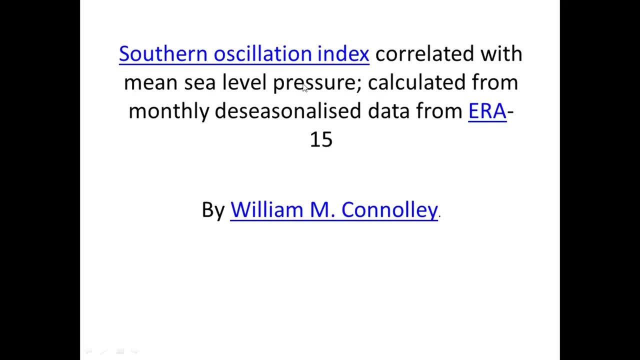 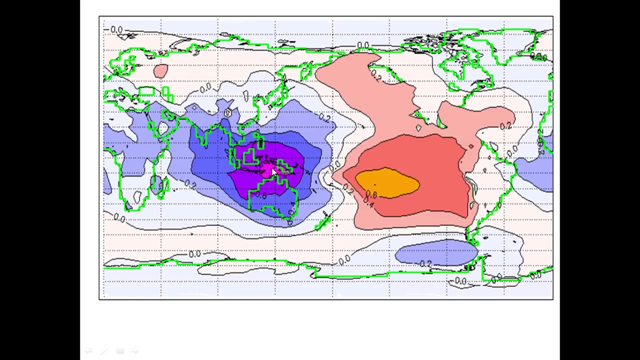 surface to reach above average temperature. strong Walker circulation causes a La Nina, resulting in cooler ocean temperatures due to increased upwelling. so here is and there's the southern Oscillation Index, correlated with mean sea level pressure, calculate from monthly de-seasonalized data. this gentleman here Connolly. so what do we? 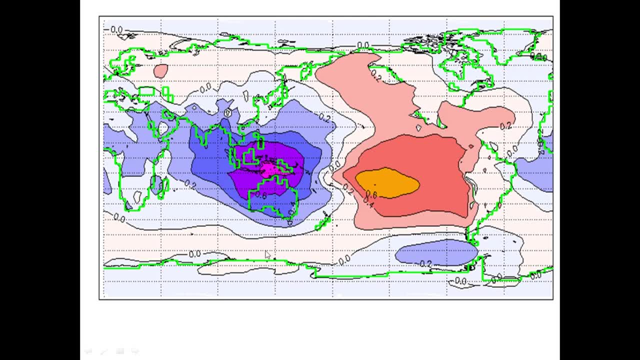 have here again. the white is normal. so you see the the isopleth lines of zero. this is positive 0.2 off of positive 0.6. over here is negative 0.2, down to negative 0.6 or even negative 0.8. so there's higher pressure here, lower. 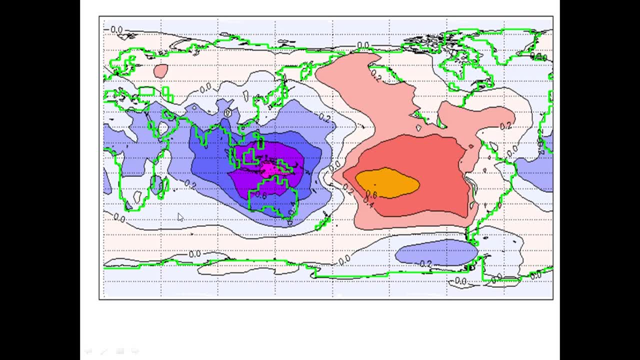 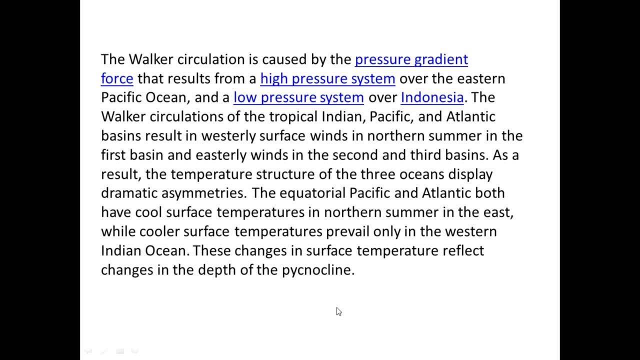 pressure. here you okay. the Walker circulation is caused by the pressure gradient force that results from a high pressure system over the eastern Pacific and a low pressure system over Indonesia. that's what this shows. Walker circulates in the tropical Indian, Pacific and Atlantic basins result in: 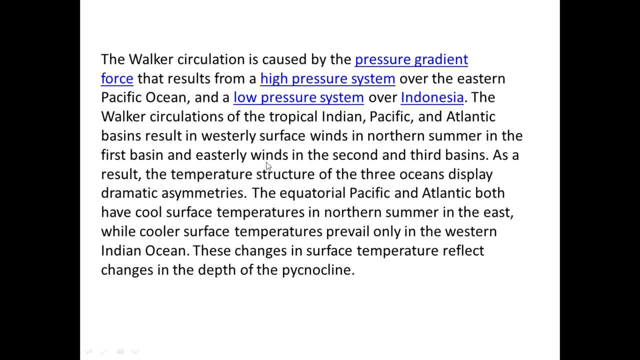 westerly surface winds in northern summer in the first base and easterly winds in the second and third basins. as a result, the temperature structure of the three oceans display dramatic asymmetries. the equatorial Pacific and Atlantic both have cool surface temperatures in. 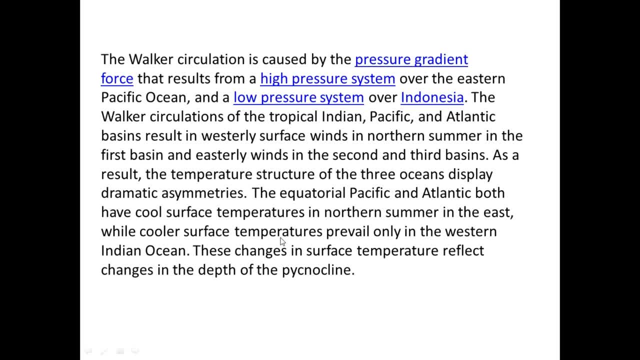 northern summer in the east, while cooler surface temperatures prevail only in the western Indian Ocean. this is related to the Indian Ocean dipole, which, as it turns out, seems to be tied into you guessed it, and so these changes in surface temperature reflect changes in the depth of the picnic line. 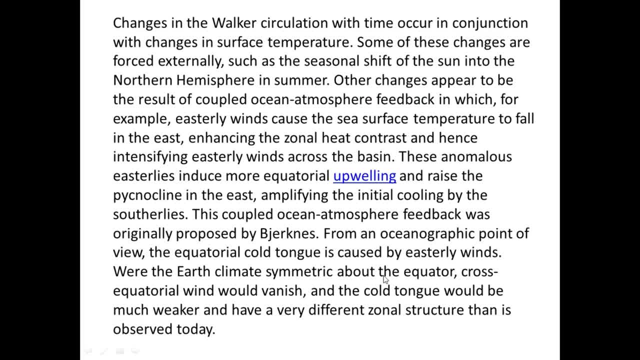 that's the change in density. changes in a walk of circulation with time occur in conjunction with changes in surface temperature. some of these changes are externally force, such as seasonal shift of the Sun into the northern hemisphere in summer. other changes appear to be the result of coupled ocean atmospheric. 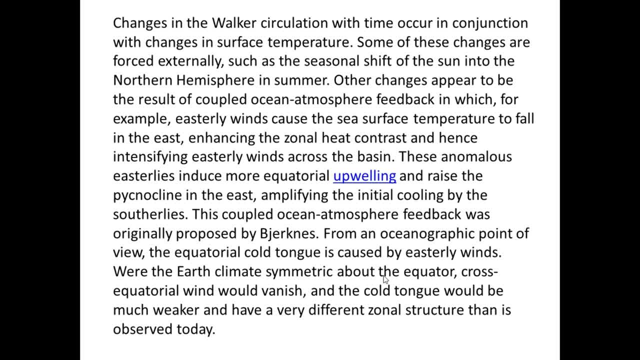 feedback in which, for example, easterly winds cause a sea surface temperature to fall in the east, enhancing the zonal heat contrast and hence intensifying easterly winds a across the basin. These anomalous easterlies induce more equatorial upwelling. 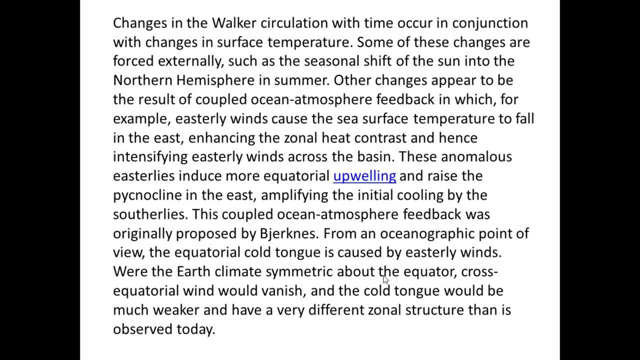 and raise the pycnocline in the east, amplifying the initial cooling by the southerlies. This coupled ocean atmosphere feedback was originally proposed by Bjergnes. From an oceanographic point of view, the equatorial cold tongue is caused by easterly winds. 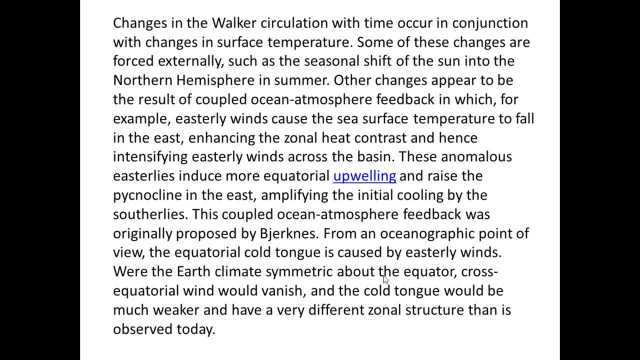 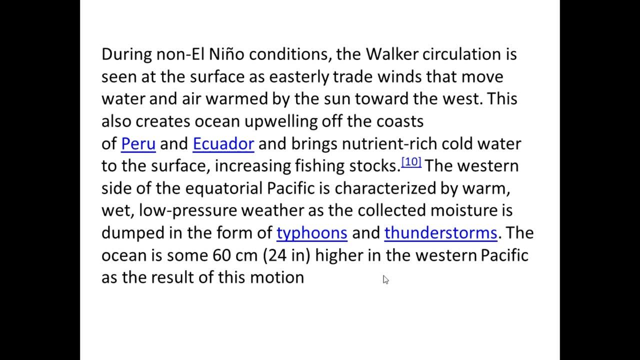 where the Earth climate's symmetric about the equator, cross-equatorial wind would vanish and the cold tongue would be much weaker and have a very different zonal structure than we see observed today. During non-El Nino conditions, the walk of circulation is seen at the surface. 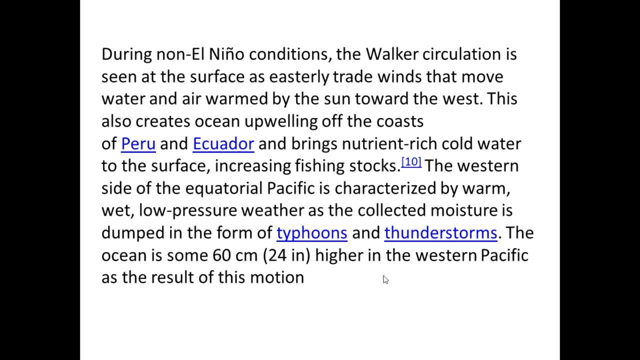 as easterly trade winds that move water and air warmed by the sun toward the west. In that atmosphere, easterly means winds come out of the east, go to the west. In oceanography if we say easterly currents, 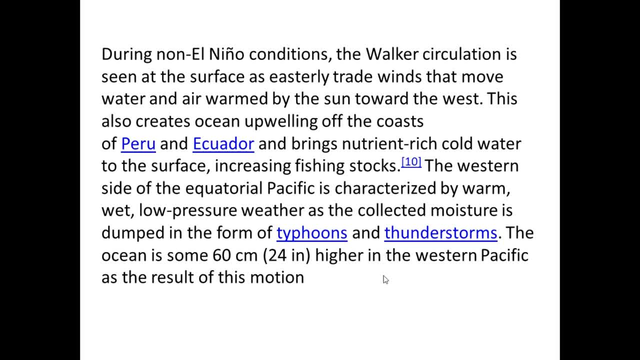 it means it goes towards the east. I know it's confusing. And this movement helps create upwellings off the coast of Peru and Ecuador, brings nutrient-cold-rich water to the surface, increasing fish stock. The western side of the Pacific. 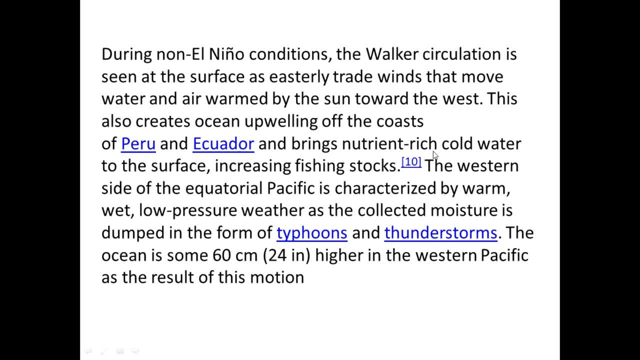 equatorial Pacific is characterized by warm, wet, low-pressure system, as the collected moisture is dumped in the form of typhoons and thunderstorms. And then you get- you know the ocean's sum- 60 centimeters higher in the western Pacific. 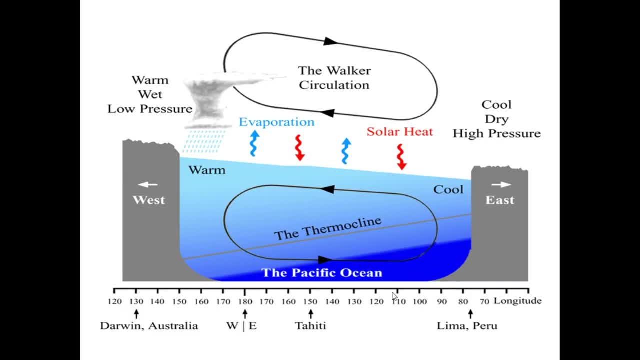 as a result of this motion. So here's a nice little figure showing the walker circulation. So we have solar heat inputting in, we have evaporation. Here's the walker circulation. As you can see, it's atmospheric. So this is the western side. 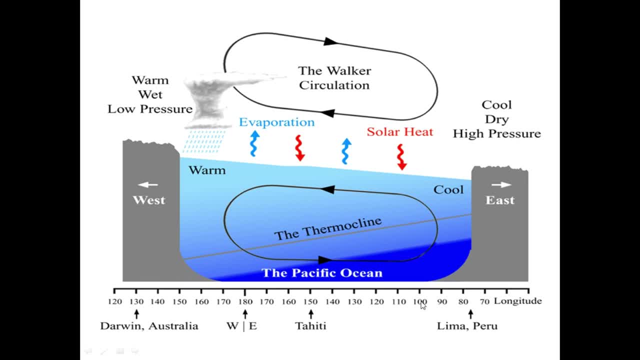 This is the eastern side. This is longitude. okay, Basically, right here is the international date line. Here's Lima, Peru, et cetera. So when you have warm water, remember as I've always described for you guys. 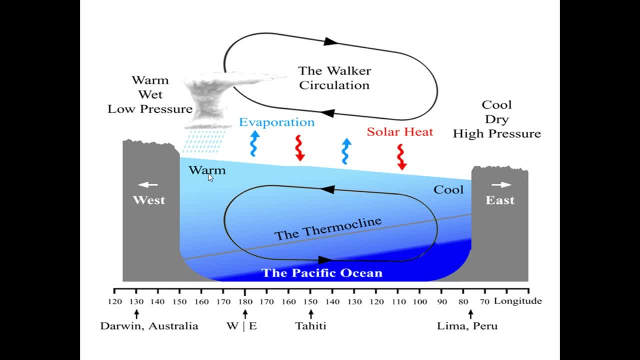 warm water is warmer, so it's going to expand. That's why it shows a little tilt here, This line right here: they're labeling as the thermocline. Technically it's the pycnocline, But let me say this at least: 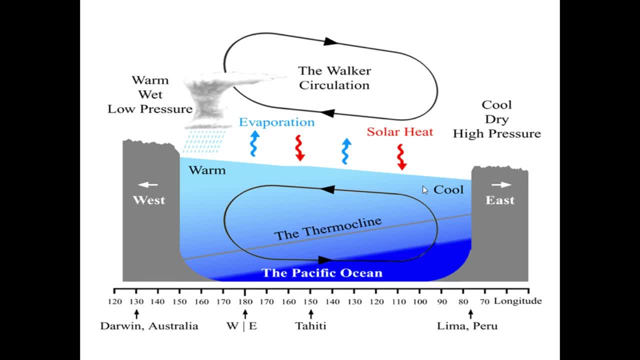 In the equatorial regions of the ocean, changes in density of oceanic water is going to be determined more so by changes in temperature. Salinity does not vary all that much, So temperature is going to be more the varying parameter, and hence it's going to be the more driving of the temperature. So temperature is going to be more the varying parameter and hence it's going to be the more driving of the temperature. So temperature is going to be more the varying parameter and hence it's going to be the more driving of the temperature. 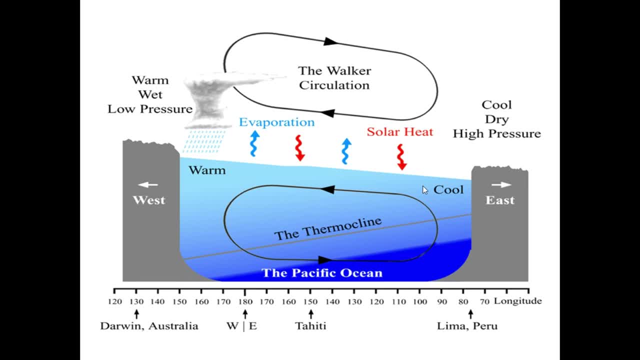 So I understand from that point of view, why they would refer to it as a thermocline, But you still have a salt content there, So I would prefer seeing pycnocline. Unfortunately, and a lot of the graph is going to show you- 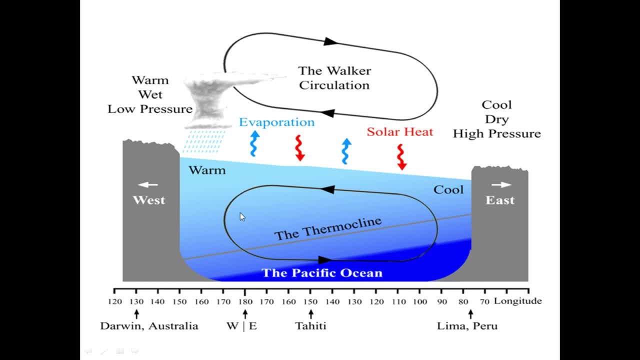 in this video series you're going to see thermocline. When you get the high latitudes, it's the salt content that changes drastically. Water is really cold, So the water temperature is not going to vary that much, but it's the salinity content will. 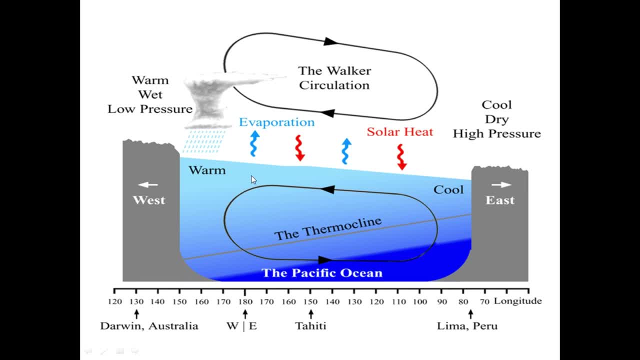 So salinity differences drive the density differences in waters at high latitude, temperature differences at water at equatorial regions. So this is a diagrammatic showing the relationship, the walk of circulation with the air pressures- high pressure, wet pressure- And this low pressure shifts back and forth during ENSO. 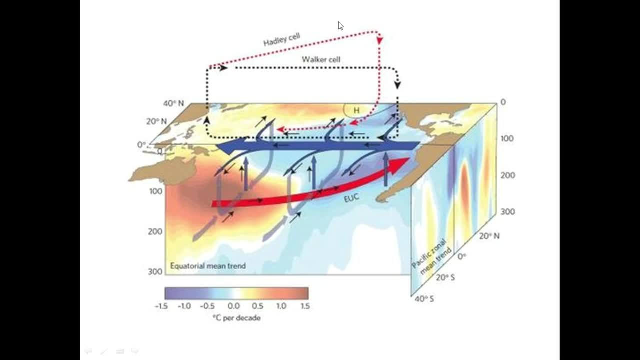 Okay, So we have Hadley cells and atmospheric circulation pattern, as is the Walker cell. Now, if you look here, we're going from zero to 40 degrees north latitude, this showing you a cross section in depth. So here's a little bit of warm water intrusion. 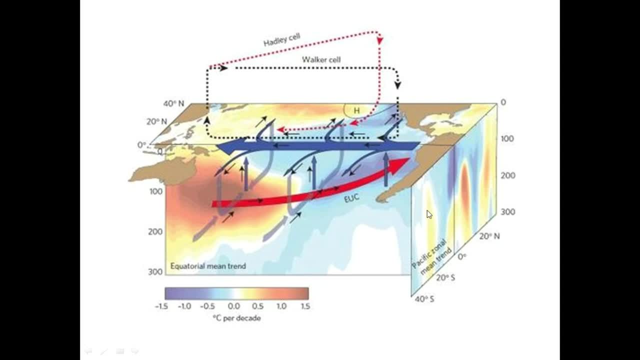 cold water reaching down The EUC is the equatorial undercurrent, So this is a subsurface, It's the surface of flow And, as you can see, we've got warmer waters here. Here's the main forcing have the winds going east to west. 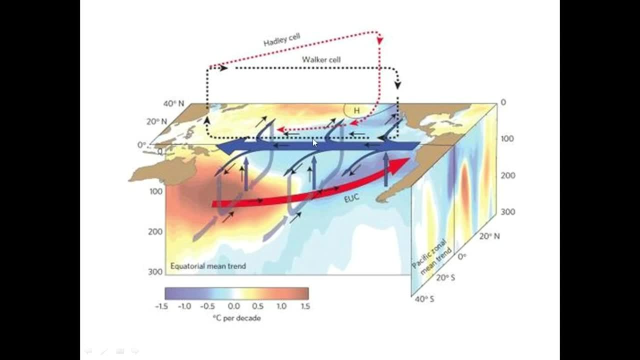 piling up the water this way And we see the atmospheric flow as well, And then what we're seeing here, these are on some vertical flows in the ocean itself. So you've got a little bit of of convective cells, cells going on. that's what all these are. these are all convection cells, you know. 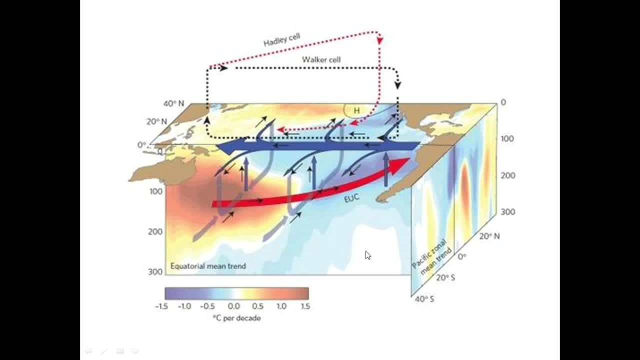 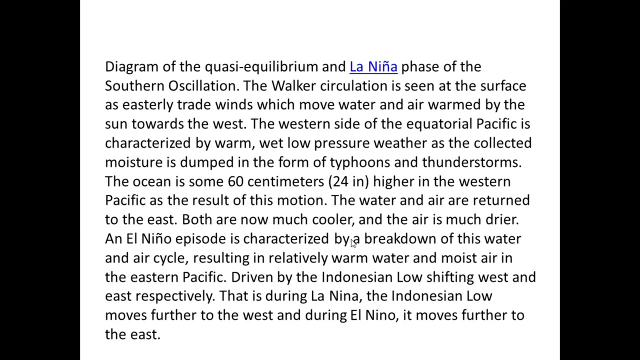 it gets warm, it rises, then cool the sinks, that kind of deal. so, and this brings this, this cool water is coming to the surface, that's the upwelling bringing nutrients, helping the fisheries along this way. so that was diagram to quasi equilibrium in La Nina phase, what the circulation seen at the surface is. 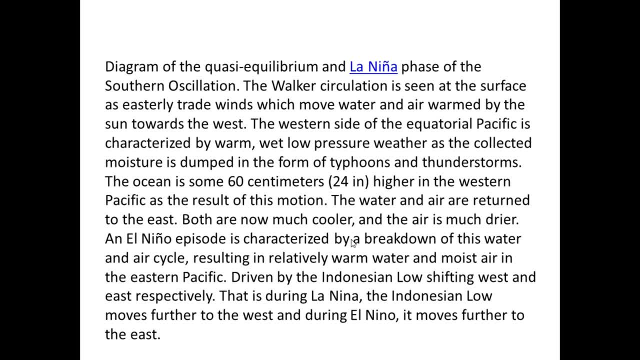 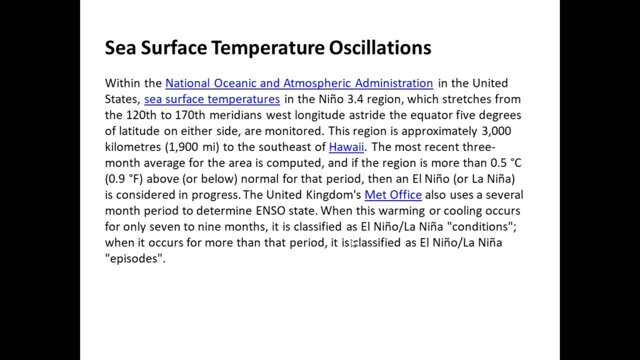 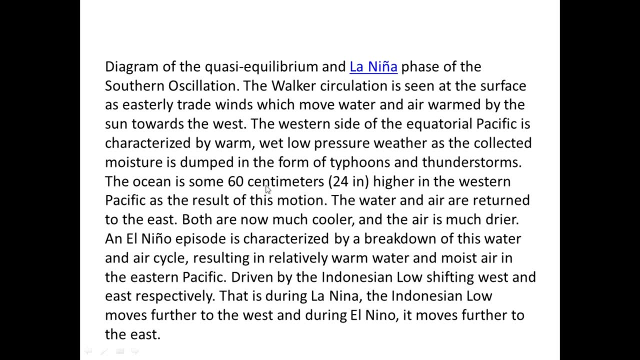 easily trade. wind which move water and warm air- warm by the Sun- towards the west western side is characterized by warm, wet, low pressure, okay, and so on. basically wanted air. or return to the east, because the result of this motion where the water is some 60 centimeters higher in the western, the water and air. 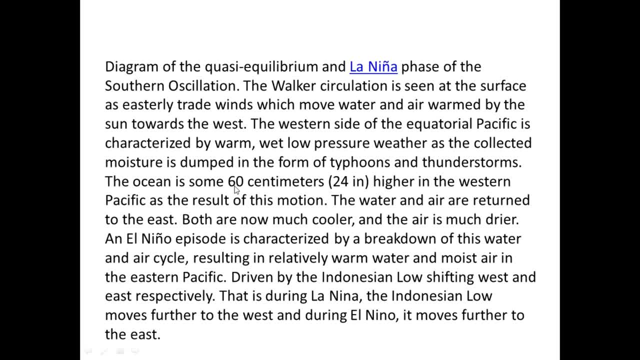 returned to the east, because if I have water that's higher on one location and it's lower in another location- let's assume a flat bottom, that's level- I have a higher pressure where the water is higher. in other words, the pressure exerted on the bottom will be higher because there's a water column is 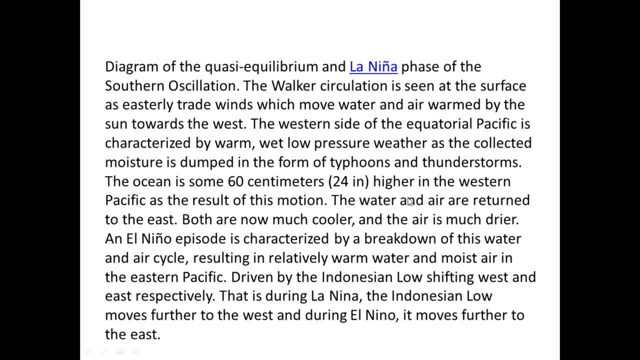 taller. exerting more pressure, it's lower. where the pressure exerted on the bottom is lower because the water level is not as high. guess what? that creates a pressure gradient. water flows down the pressure gradient now because it's occurring at the equator. the flow is in a straight line when you get away from the equator and 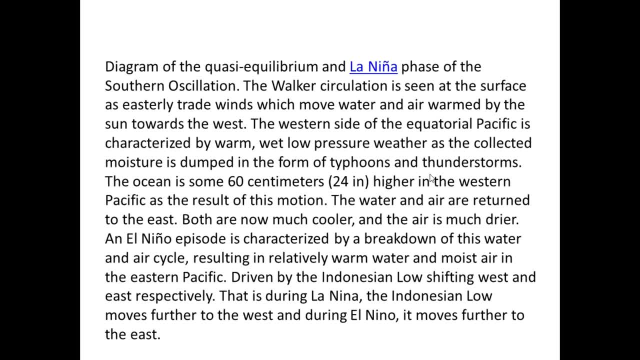 water flows down the pressure gradient, then the Coriolis effect acts upon it, deflecting the motion. in the northern hemisphere it's to the right, southern hemisphere is to the left. that is how you set up oceanic gyros and, and related to that, how you get cyclones and anti cyclones. I will discuss that in a minute. 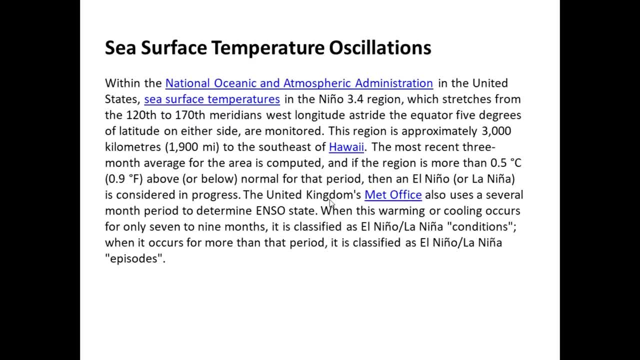 that more so later on. now let's look at sea surface temperature oscillations. okay, NOAA and the us sea turf. sea surface temperatures in the Nino 3.4 region. I have a graphic will show you the bay widow where the stations are to collect. 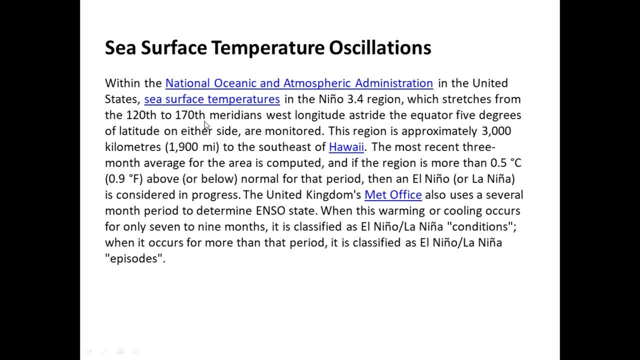 the data and stretches from the 120th to 170 meridians west longitude to stride the equator, 5 degrees of latitude and either side of monitored. this region is probably 3,000 kilometers away from the equator, 5 degrees of latitude and either side of monitored this region is probably 3,000 kilometers. 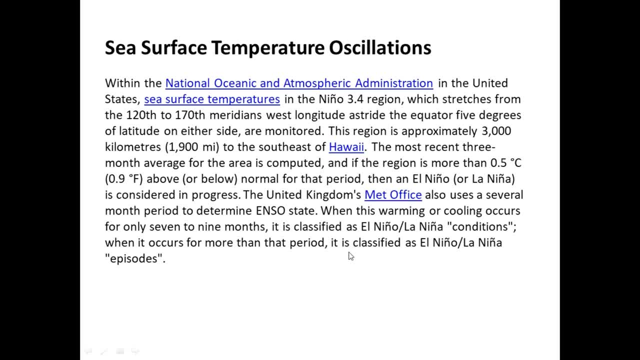 to the southeast of Hawaii and what they do is they calculate the most recent three-month average. they do a running average. the region is more than 0.5 degrees C above or below normal for that period, then El Nino, or line union, is considered in progress. UK's Met Office also uses a several 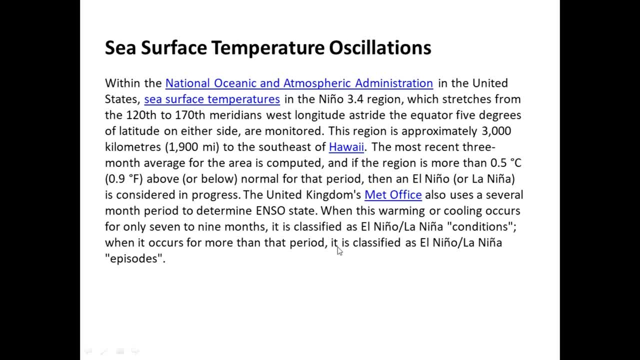 month period to determine and so state when the warming and cooling occurs for only seven to nine months. it's classified as El Nino line unit. can be determined by the temperature variation in the climate and the temperature variation in the climate and the temperature variation in the climate. 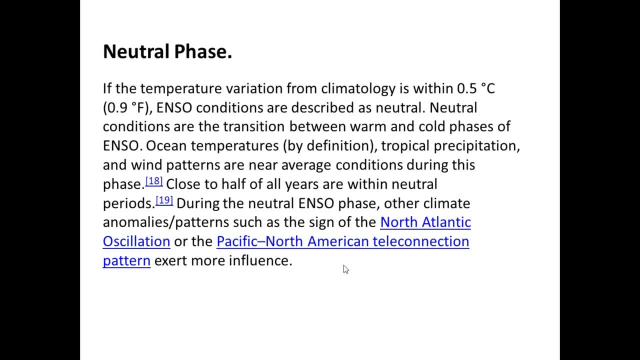 conditions versus episodes. neutral phase temperature variation climatology is within half a degrees, and so conditions described as neutral. neutral conditions are the transition between warm and cold phases of ENSO ocean temperatures. by definition, tropical precipitation wind patterns are near average conditions during this phase. close to half of all years are within neutral periods during the neutral. 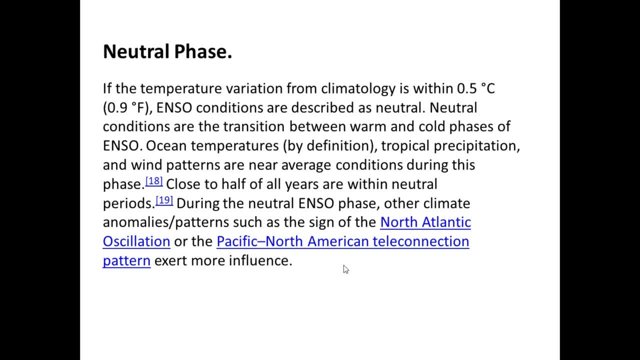 ENSO phase. other climate anomalous patterns, such as the sign of the North Atlantic Oscillation or the Pacific North American teleconnection pattern, exert more influence. what the teleconnection refers to is atmospheric communications across oceanic basins so that, because of what, whatever atmospheric cells are happening, could result in the Atlantic and Pacific. 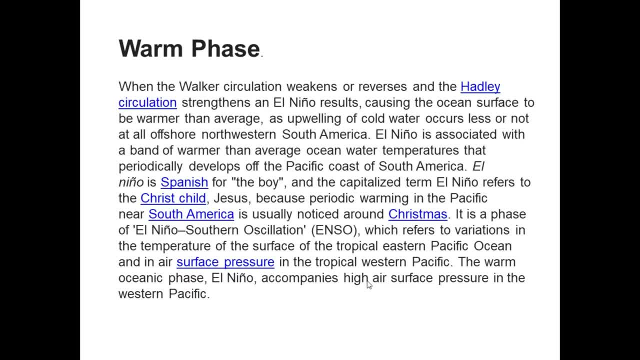 oceans communicating. for example, ocean surface is warmer than average as up well and cold water occurs less or not at all. El Nino associated with a band of warmer than average ocean water temperatures that periodically develops off the Pacific coast of South America. okay, El Nino accompanies high air pressure surface temperature in the 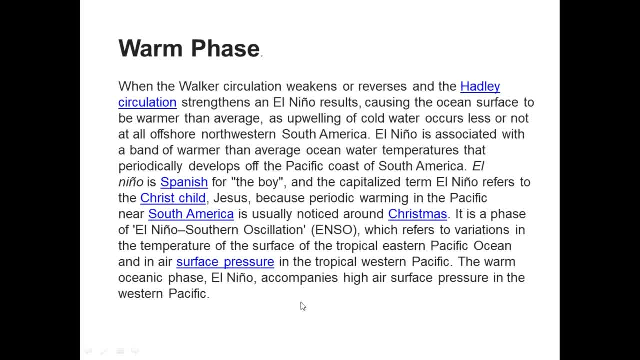 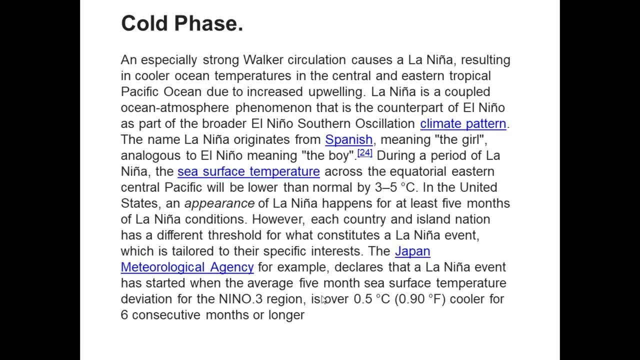 western Pacific. that's the warm oceanic phase and the cold phase. this one we get kind of the opposite. we get the La Nina sea. surface temperatures across the equatorial eastern Pacific will be lower by normal than three to five degrees C. and you know, you got a few of. 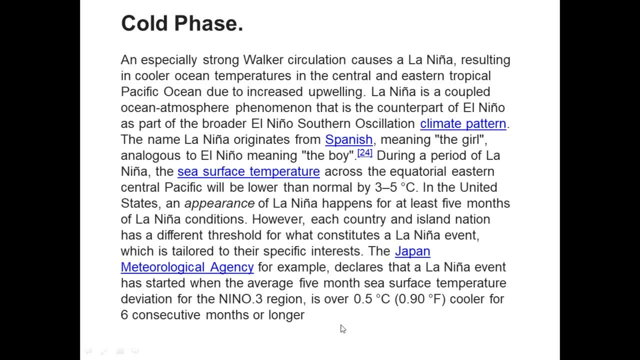 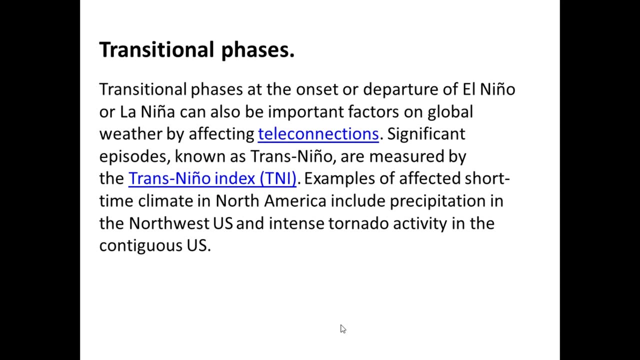 the other little background information. As always, you can always pause the video to you know any time. stop and look at the figures. read the descriptions. Transitional phases At the onset of departure of El Niño or La Niña can be important factors in global weather by affecting teleconnections. 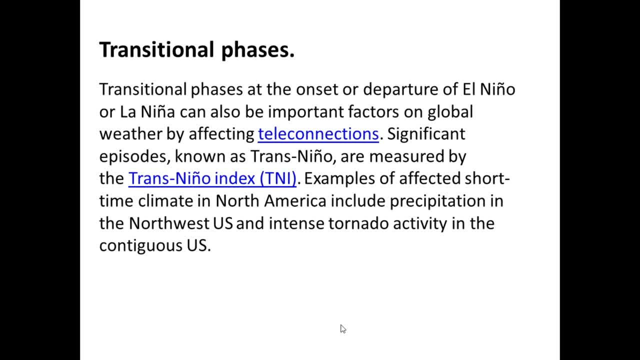 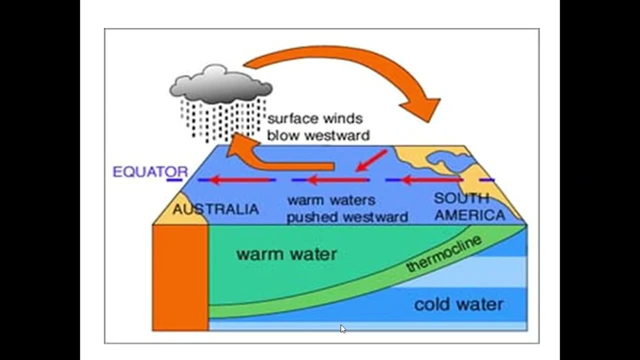 Significant episodes known as Transniño are measured by the Transniño Index, TNI. An example of affected short-time climate in North America include precipitation in the northwest US, intense tornado activity in the contiguous US. Okay, So this is a diagram, maybe a little simplified one from the one I showed you earlier. 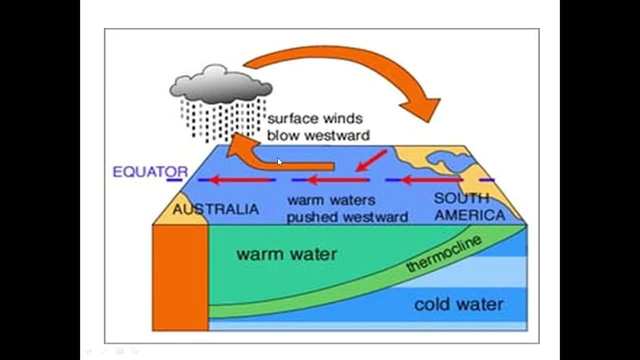 So we have warm waters push westward, surface wind blow westward. So here's a low-pressure system. We've got some precipitation going on here. There might be movement to the east. Here's the warm water, Here's the cold water. 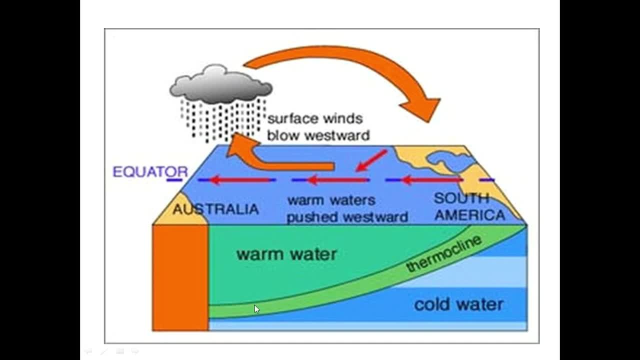 Here's the cold water. Here's the thermal cline. As you can see, the thermal cline is angled up, It's bent, It's not level, And that's because warm water is transitioning gradually to cold water with the abrupt change over the thermal slash pycnocline. 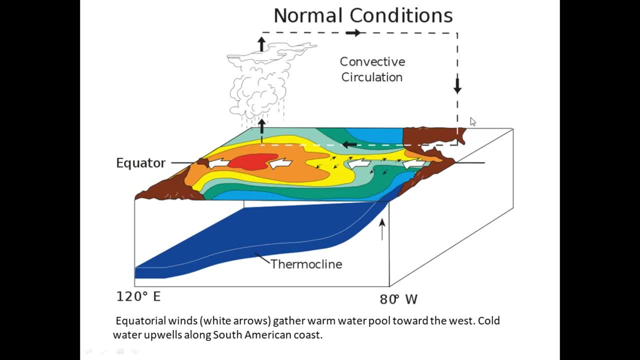 So here's normal conditions, Conductive circulation. Note the position of this low-pressure system. Here's the thermal cline coming up to the surface or near the surface. Here's the thermal cline coming up to the surface or near the surface off the coast of South America. 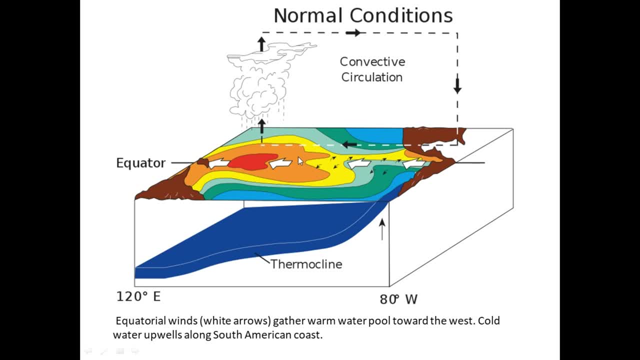 Here's the thermal cline coming up to the surface or near the surface off the coast of South America. Here's the winds pushing the water, piling it up. this way: Warmer surface temperature. this way: Equatorial winds. white arrows gather the warm water pool toward the west. 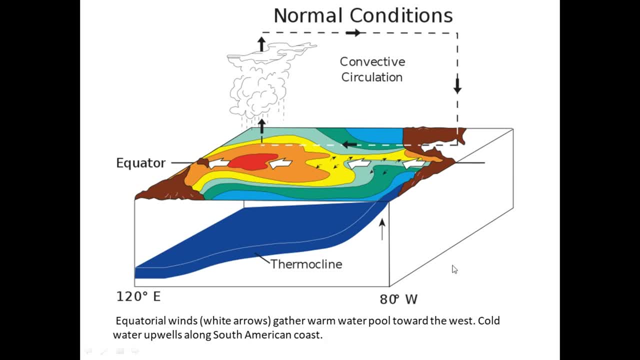 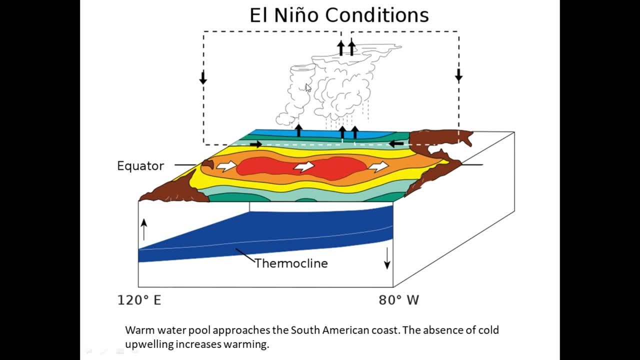 Cold water upwells along the South American coast. This is normal or neutral, if you like. Now look at El Nino. Okay, First of all, see how this pressure system has shifted Right. It's gone to the east, And that creates two convection cells this way and this way, instead of just the one. 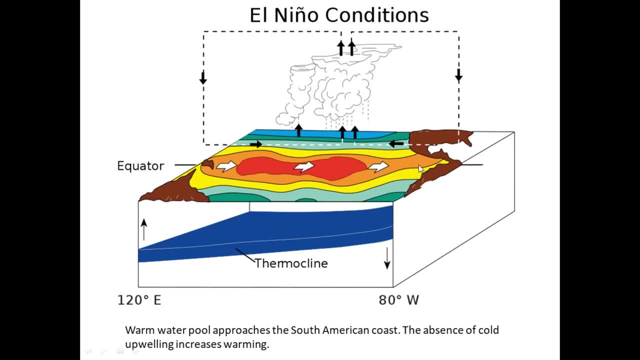 Now you see how the warm water has moved this way. You see how the thermal cline slash pycnocline is now deeper. it's depressed. You're not going to get the upwelling. Now you get this warm water off South America. 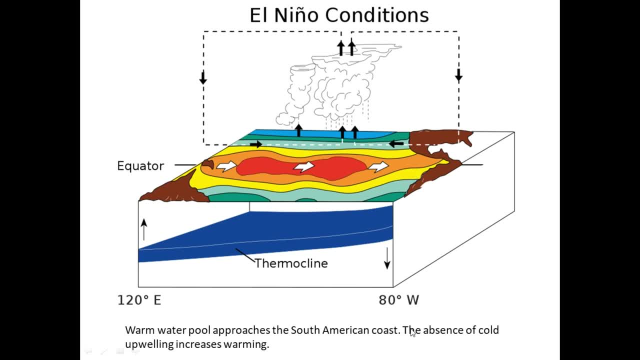 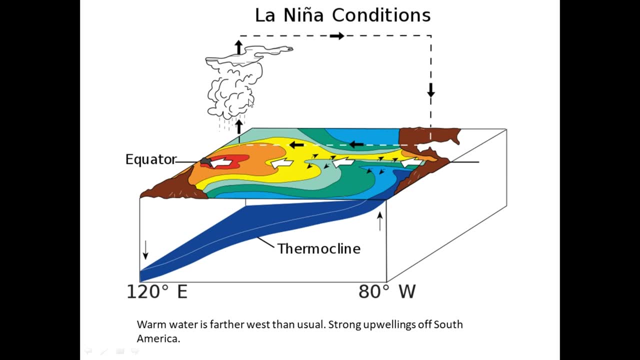 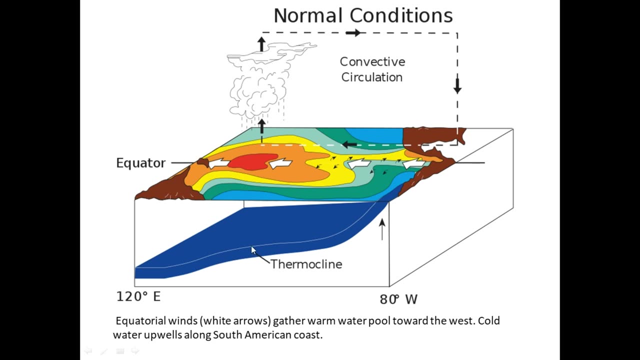 Warm water pool approach the South American coast. The absence of cold upwelling increases warming. And then, La Nina, You'll see how this low pressure system shifted even further west. Right, You see it's, you line it up, It's about that'd be about 105 degrees west latitude. 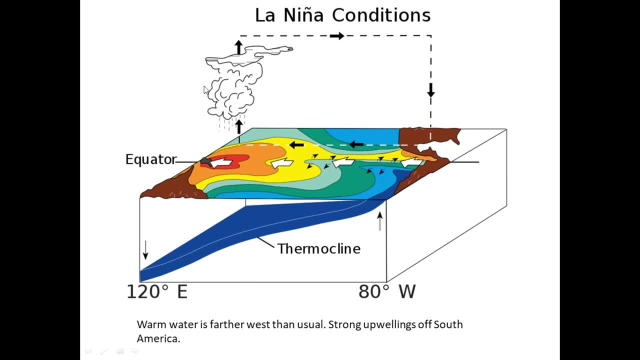 You can see it's gone further. It's like about 110.. You'll notice again, looking at the, that the pool of warmer water is smaller. We have colder water here. We still have the west leaves pushing the water, but not as strongly. 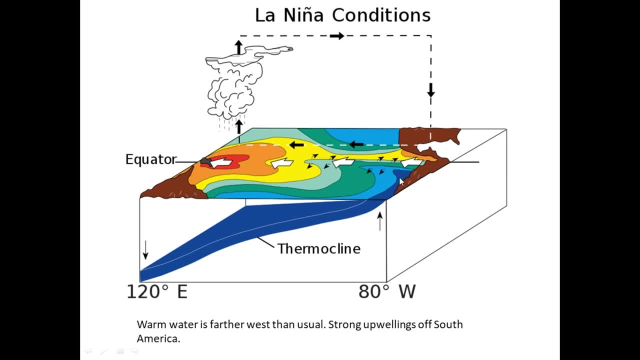 And now the thermal cline, pycnocline, basically reaches all the way to the surface. Warm water is farther west than usual, Strong upwellings off South America. That's kind of diagrammatically what's happening And it's the shifting of what the winds are doing, what the sea surface temperature is doing. 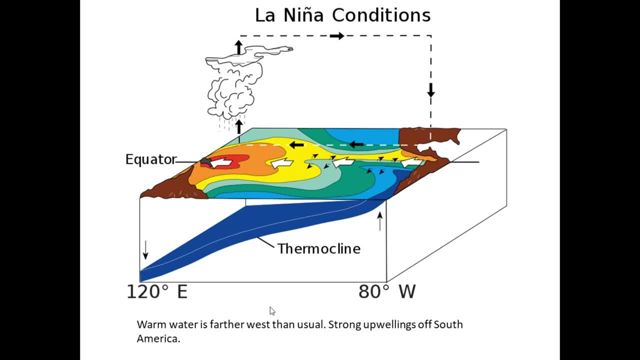 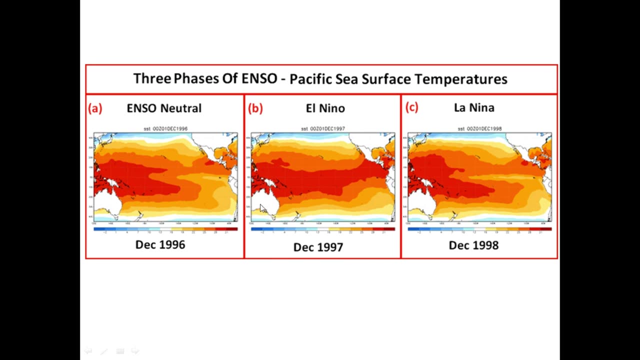 where the low pressure system is is at and all the forcings that come with that And, as it turns out, it's tied into the PDO. So here are taken in December in three consecutive years And so neutral. So this is sea surface temperatures. 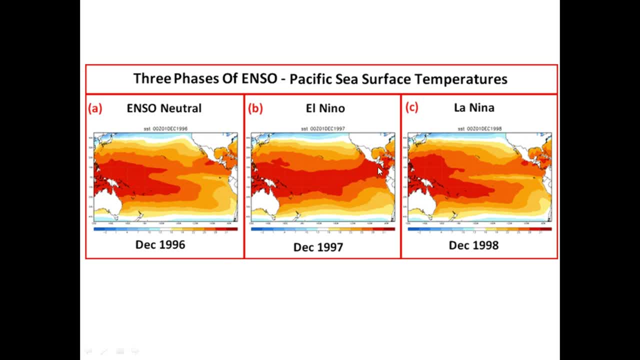 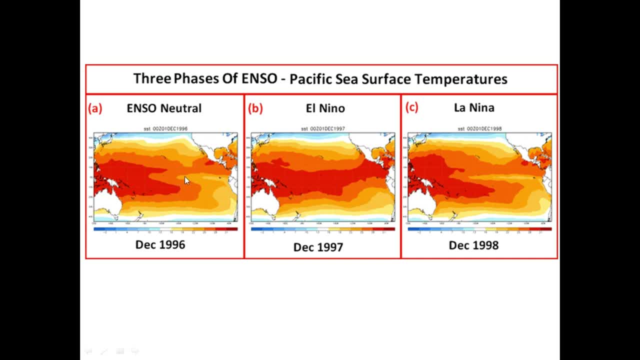 Cetus cool tongue, Cetus cool tongue, Cetus cool tongue. And it stretches further west. See this right there, Right there. This here has gone further to the west. This is actual satellite data. So, again, white is the normal condition. 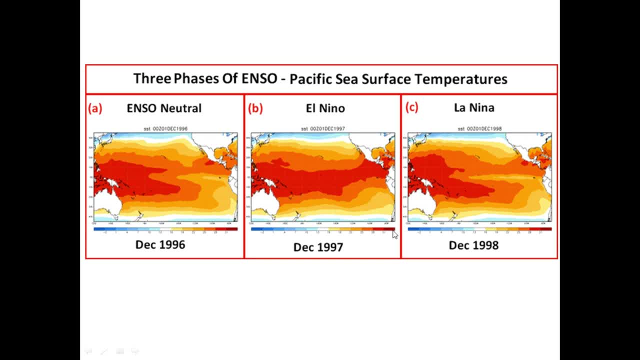 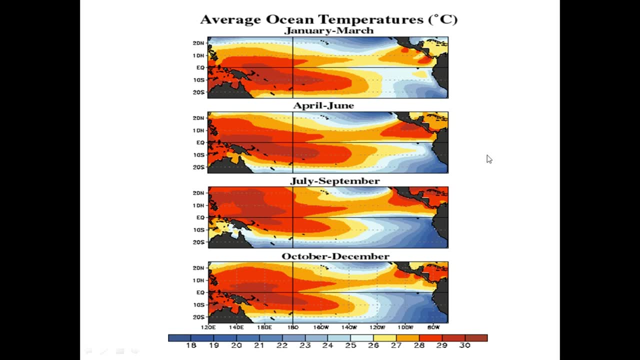 If it gets to blue, it's colder than average. It gets to red, warmer than average. So that's the phases of ENSO And average Average ocean temperature: January to March, April to June, July to September, October to December. 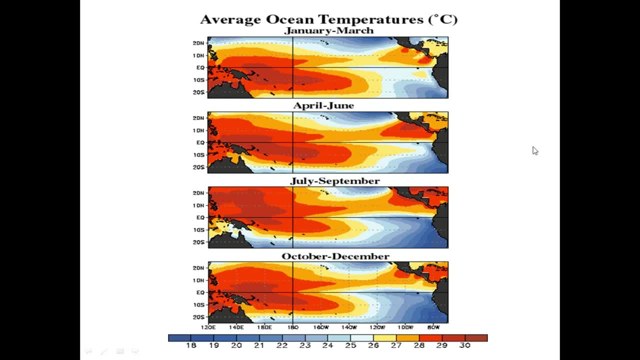 This is over a one-year period And as you look at this, you can see that this is looking like a La Nina situation. Looks like we're transitioning a little bit, And then it didn't quite go all the way, although it still got cold water off Peru and South America. 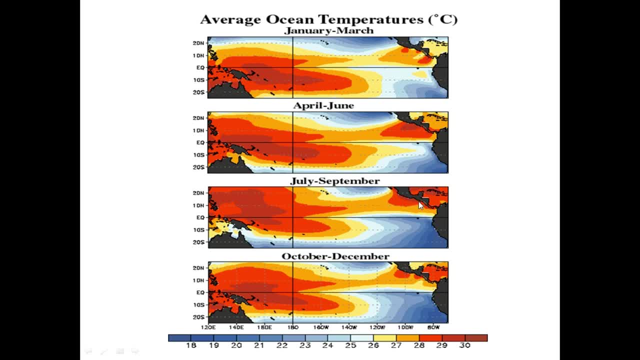 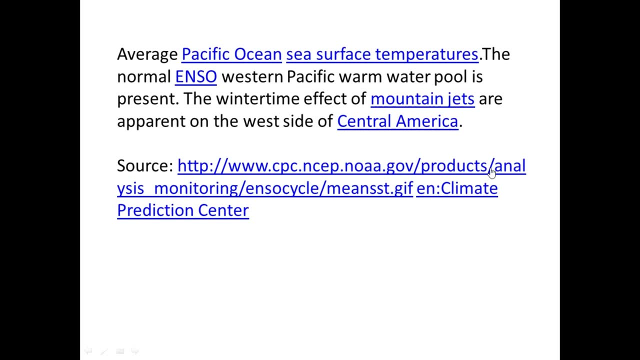 but a little warmer off Central America. It looked like it wanted to go into an El Nino, but it didn't quite. So now we look at- and, by the way, this is a good website. If you want to click on that to explore this in greater detail, go for it. 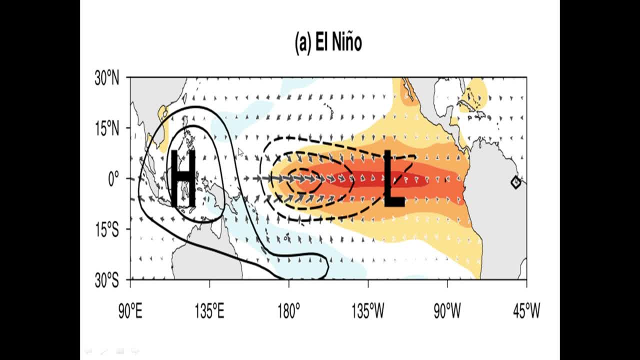 Here's the pressure system When El Nino. You see, these arrows indicate wind forcing, wind direction. The longer and or thicker the arrow, the stronger the winds are. These are called vector fields, by the way, So we've got some very strong winds here, pretty much blowing right along the equator. 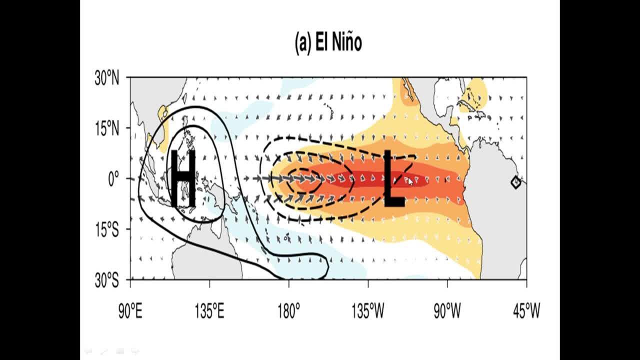 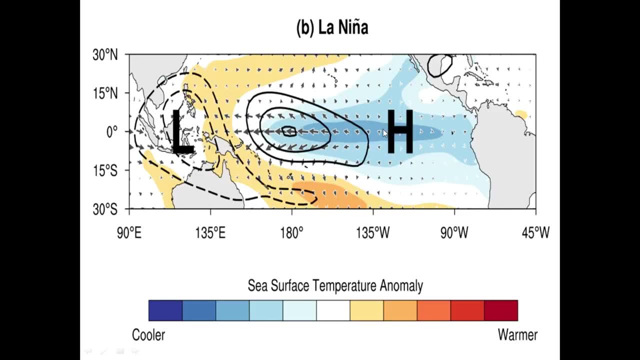 and it's blowing from west to east, So it's pushing the water this way And then, La Nina, We get the reverse. Now the winds are going this way, So this is sea surface temperature anomaly. Let's see that This is separate from this. is the L and the H refer to the atmosphere. 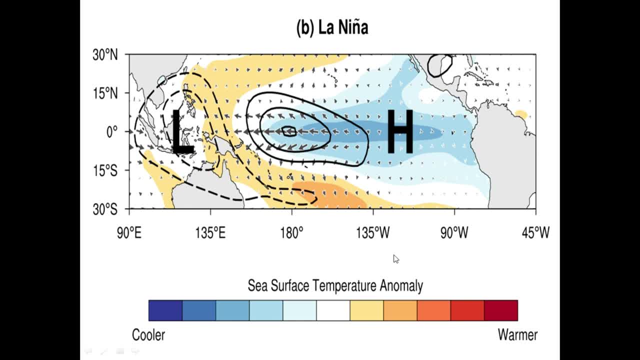 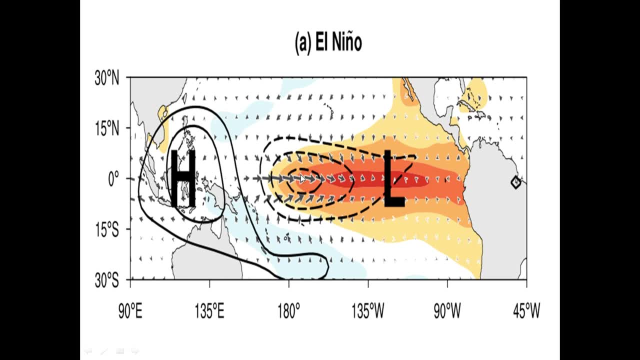 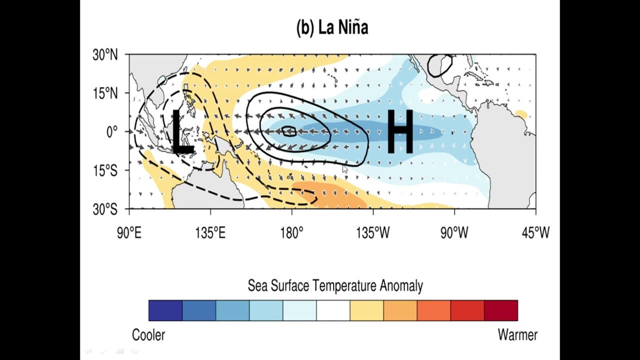 The colors here refer to sea surface temperature, showing the coupling system. So it's a little cooler here. You can see it's a lot warmer here And you can see that the direction of the winds have changed. You can see that. So basically, you can see the flip-flop in these conditions. 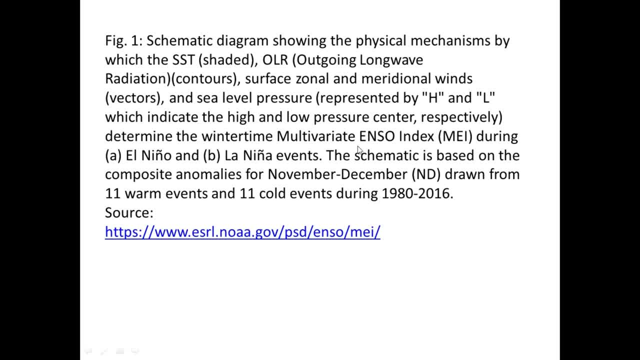 OLR is outgoing long wave radiation. Okay, I'm not, don't worry about that. Sea level pressure, represented by high and low High and low pressure center, also tied into the atmosphere. And then we have the multivariate ENSO index. 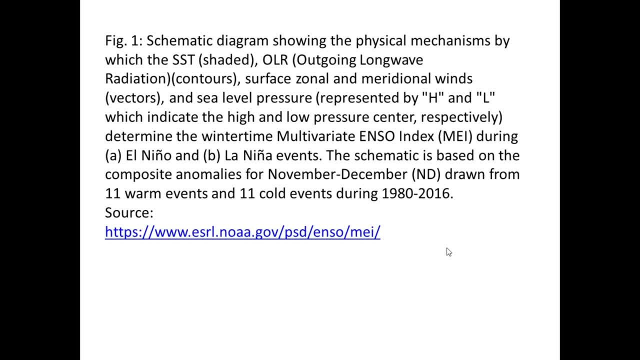 Now, when you calculate the ENSO index, what you're calculating, the parameters you're looking at, are sea surface temperature, sea surface heights, which gives you sea surface pressure, atmospheric pressure- You're looking at. precipitation You're looking at. those are the main parameters. 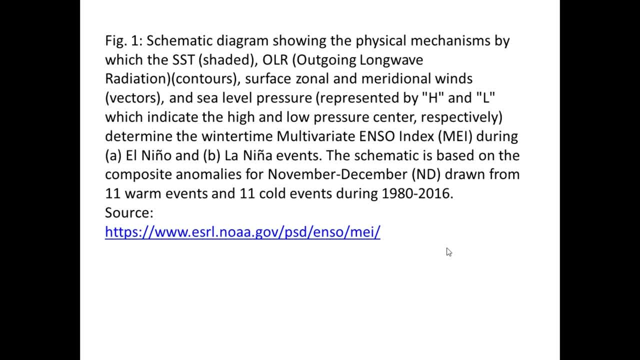 There are some other parameters, but those are the ones that I looked at And then they're calculated And you'll note I'm including a lot of the where you can find this information If you want to do further exploration in detail. 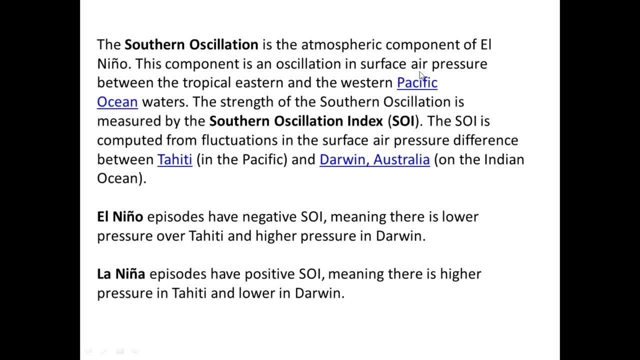 Southern Oscillation is the atmospheric component And this is an oscillation of surface air pressure And it's called the strength, It's called the SOI- Southern Oscillation Index. El Nino episodes have negative SOI, meaning there's lower pressure. 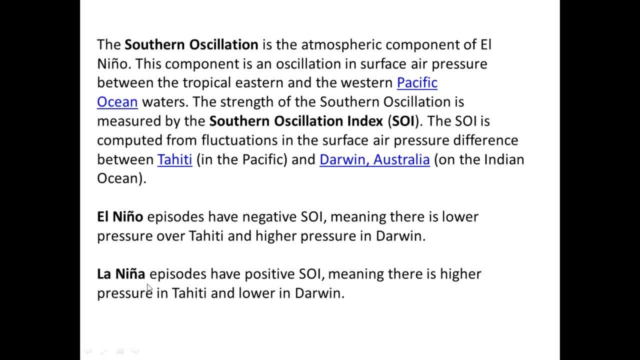 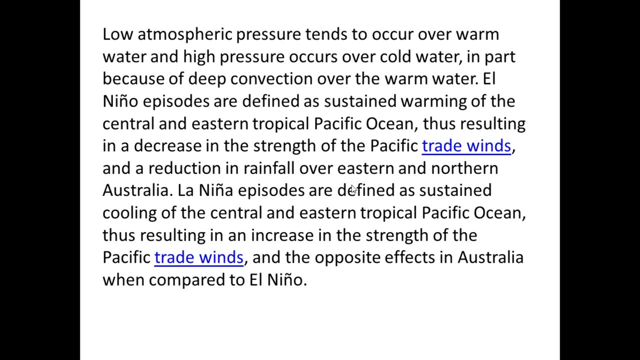 over Tahiti and higher pressure in Darwin. La Nina episodes is the reverse. So they're basing on air pressure difference between Tahiti and Darwin, Australia, on the Indian Ocean side, So they're kind of looking at a small distance. Low atmospheric pressure tends to occur over warm water, high pressure over cold water. 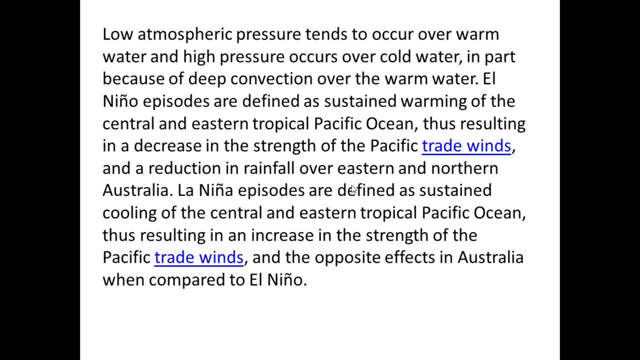 Warm water is also where you know you got warm. you're going to have more evaporation leading to, so you're going to have a thermal rising, And one of the features of a a low pressure system are updrafts. 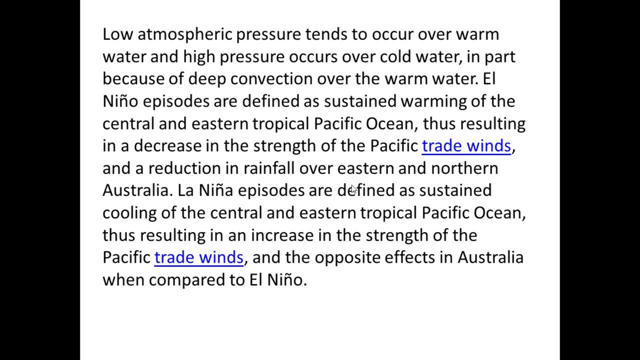 Down drafts are a feature in a high pressure system And when you have high pressure system over the ocean, it's also going to push the ocean surface down, Whereas a warm, a low pressure system, the pressure is reduced. So in addition to the water expanding from thermal expansion. 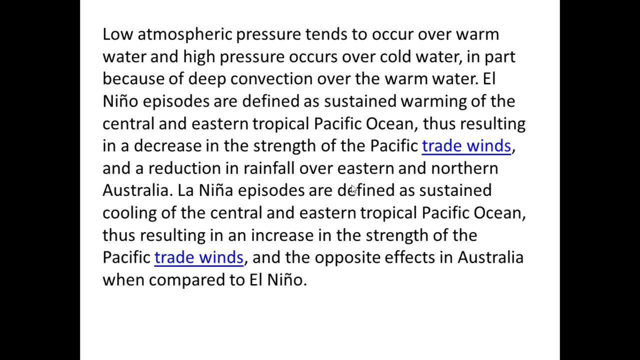 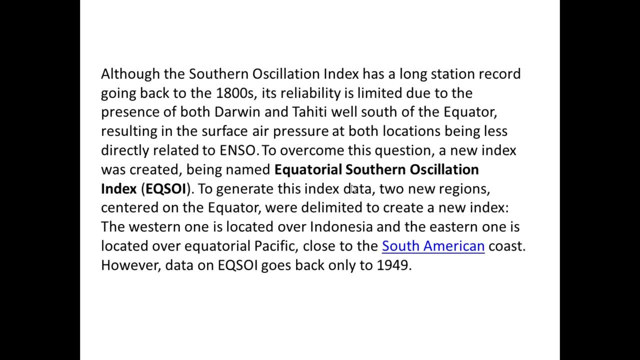 it's going to expand from the fact that it's reduced pressure on it, So it's going to the sea level will also increase as well, And this is just some verbiage about the Equatorial Southern Oscillation Index to help generate a better values and calculations and a better understanding of the mechanisms. 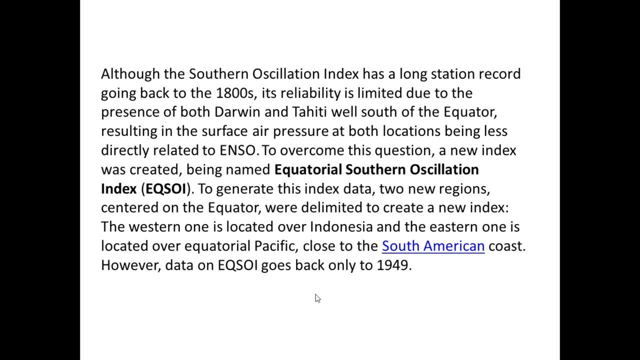 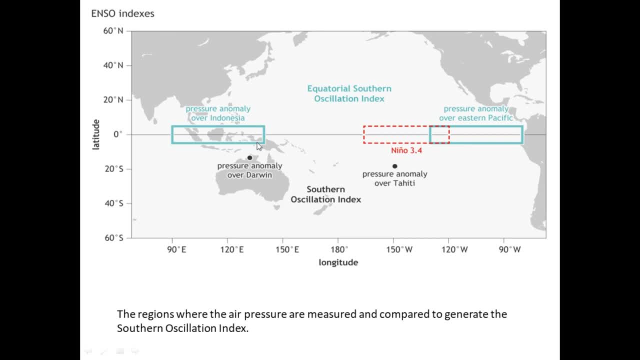 This is the regions where air pressure are measured and compared to generate the SOI. So you got this region here: pressure anomaly over Indonesia. And this is the region where the air pressure is measured and compared to generate the SOI. So you got this region here: pressure anomaly over Indonesia. 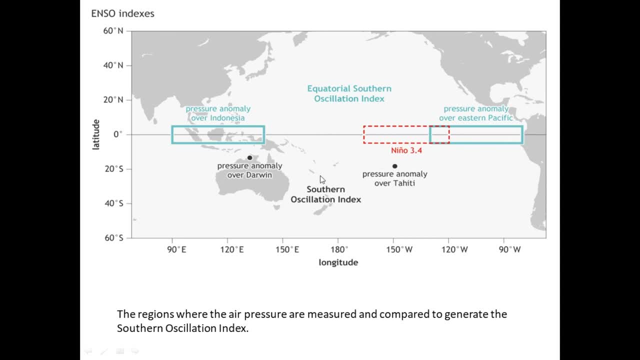 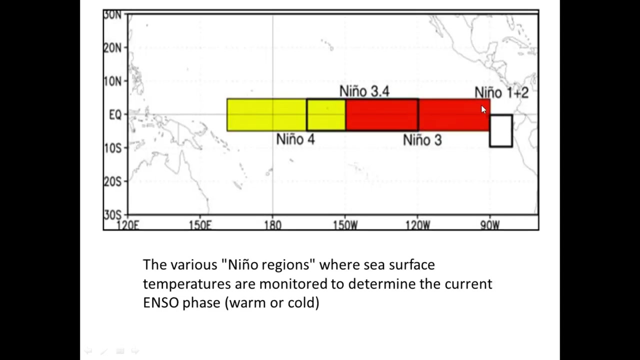 And then here are some of your stations: Tahiti, Darwin, that kind of stuff. This is showing you the location of where to collect the data, And this is just zooming in on this bit here So you can see where they monitor the sea surface temperatures. 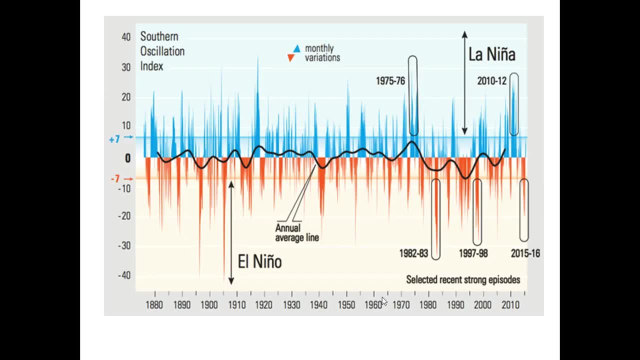 That just gives you an idea of where to get the data from. Okay, here we go. This is the whole ball of wax. Here's the SOI. Negative values have an El Niño, which is a warming situation for the ocean. 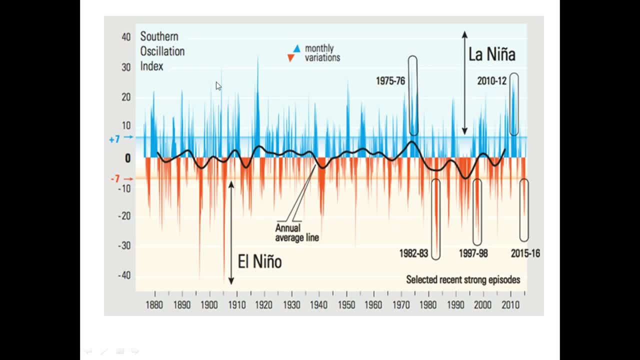 La Niña is a cooling situation and you have positive values. Now you see this horizontal blue line this way. You see this horizontal red line this way. Sounds like a hockey rink right In between. here is considered to be the ocean. 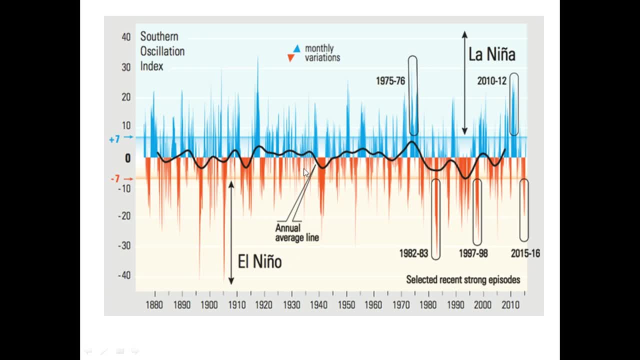 Okay, And then here is considered to be normal or neutral. So when you get to all these peaks this way and this way, this is when you have the episodes. This is a strong La Niña in 75-76.. Here is that La Niña of 88.. 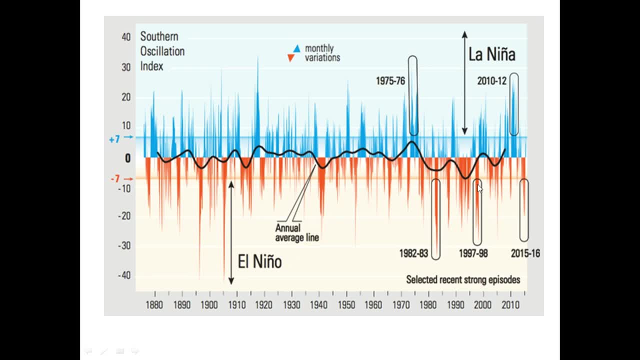 This is a strong El Niño of 82-83, and this is a very strong one, And we have a more recent one, A more recent strong one here, And this was for several years running of an El Niño situation. This is a strong dip down. 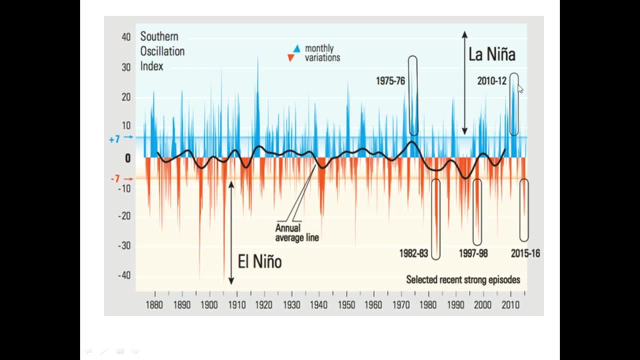 And we're actually coming out of a La Niña recently, Kind of a strong one that way. So in between here is neutral or normal. So you might have a sort of a condition, but not an episode Where the lines go above or below depending which side of the graph. those are your episodes. 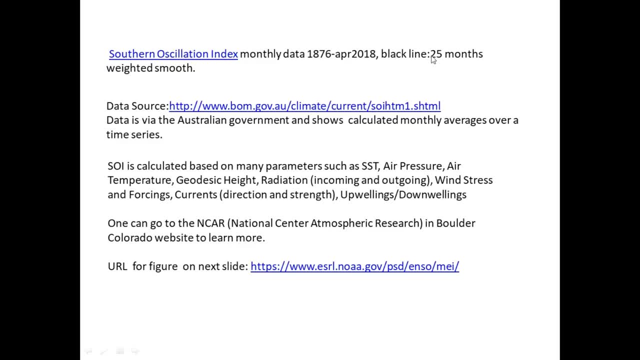 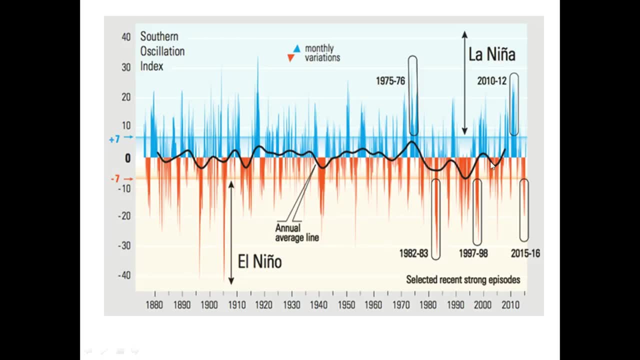 What is the black line? The black line is 25 months, weighted smooth. In other words, you're kind of trying to average out the values here. 25 months, It's over a two-year period. Hence the lag and hence why it stops before. 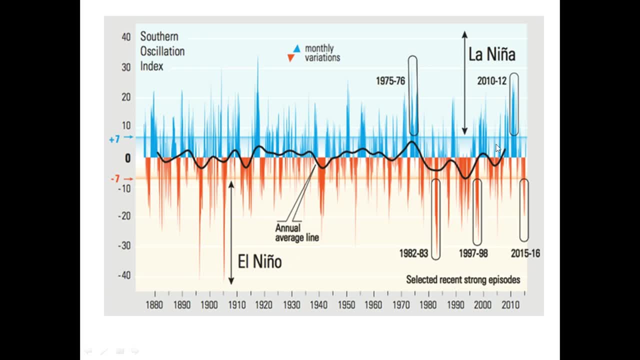 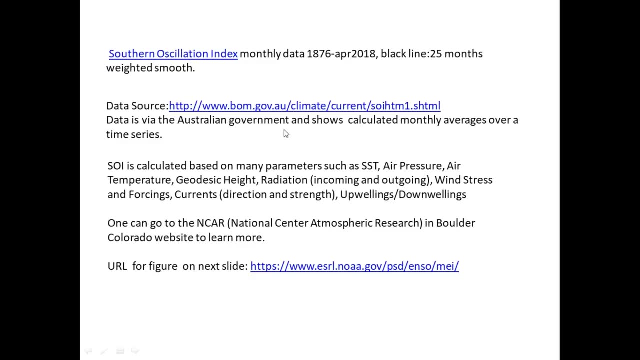 So you can see this shows you a Somewhat cyclical nature to it. And here's the data source. Data's via the Australian government SOI is calculated based on many parameters: Sea surface temperature, air pressure, air temperature, Geodesic height. 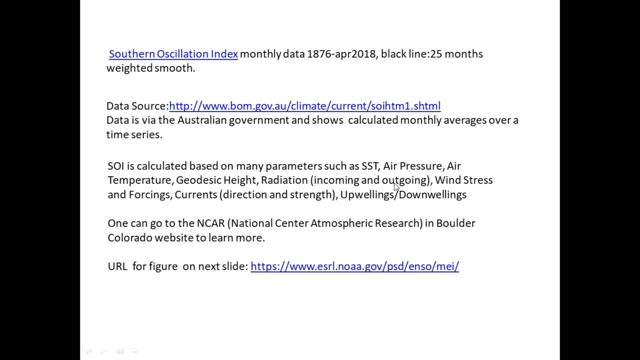 Sea level height. basically Radiation, Incoming and outgoing. Long wave radiation, for example, is outgoing Wind stress, That's the force of the wind on the water, Enforcing the currents, the direction of strain and weather. There's upwellings and downwellings. 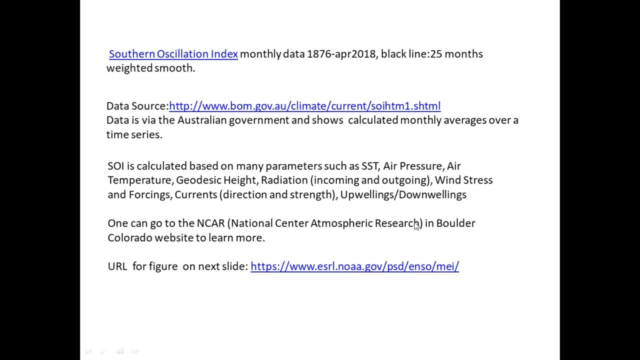 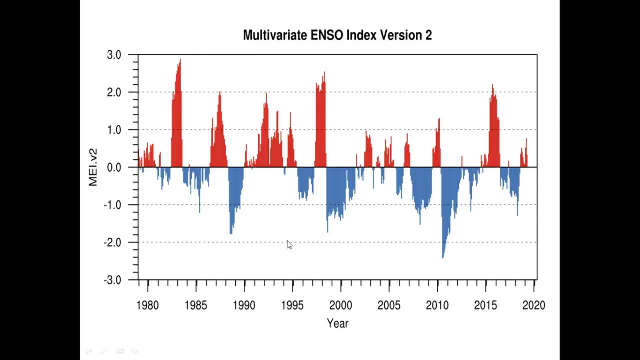 One can go to the NCAR, which is National Center Atmospheric Research in Boulder, Colorado, website to learn more. And then the URL for the figure on the next slide. this one here is basically similar to the first index slide I showed you. 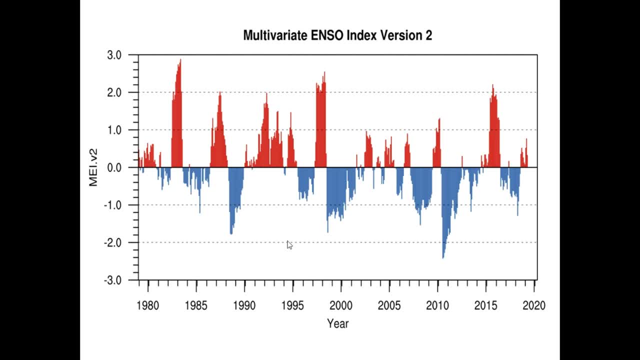 but kind of a little cleaned up so you can see things a little better. Again, here's that nasty 88, 89. A lot of La Nina. Now the. Actually, I just now noticed something: The temperature, The number scales are reversed. 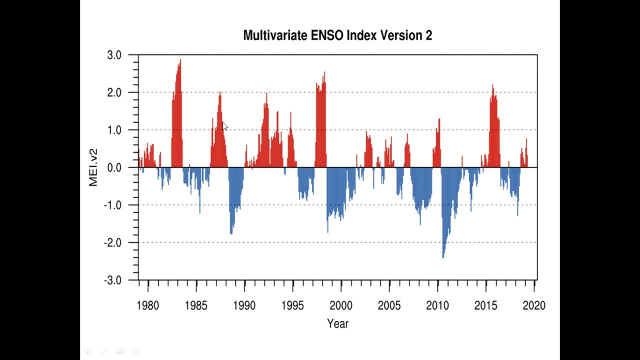 These should be positive values and these should be negative values, because this is El Nino up here, This is La Nina down here, So here's that 2012.. Yeah, so when you look at this, this is minus one minus two minus three. 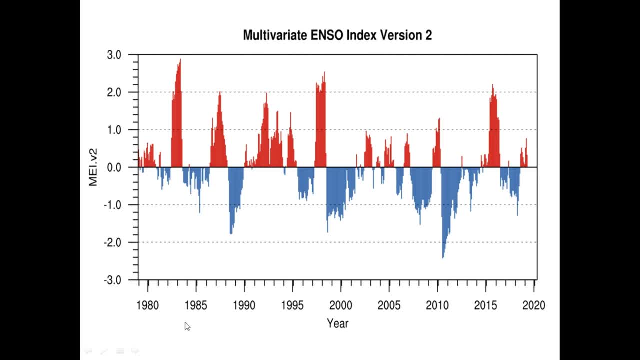 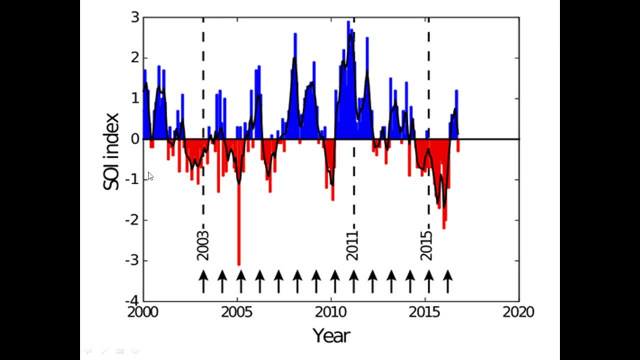 That's Positive one, positive two positive three. I didn't even catch that until just now. See Here's the, Here's La Nina El Nino. See how, Right Now, the numbers are agreeing. So this is looking at a smaller time scale over basically, you know, 17 years or so. 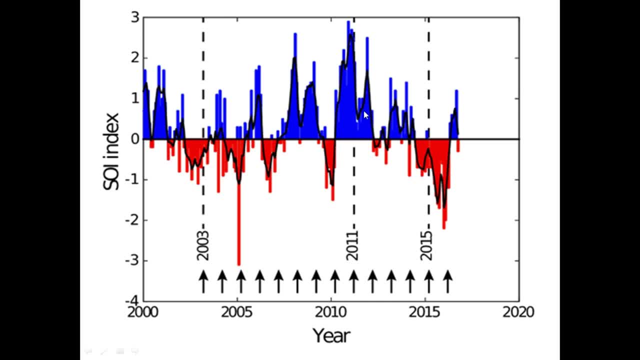 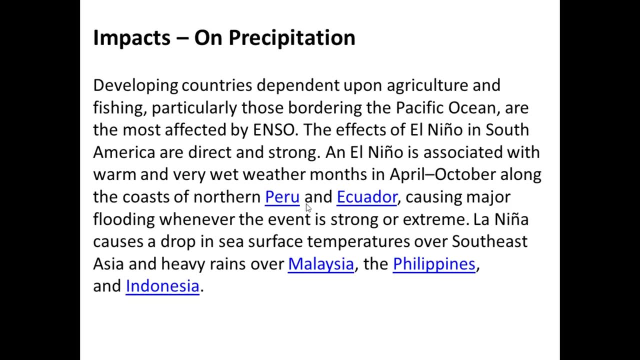 And here's that La Nina coming out of. Here's the El Nino we just had. Here's the El Nino we just had. Impacts on precipitation. Developing countries dependent upon agriculture and fishing, particularly those bordering the Pacific Ocean, are most affected by ENSO. 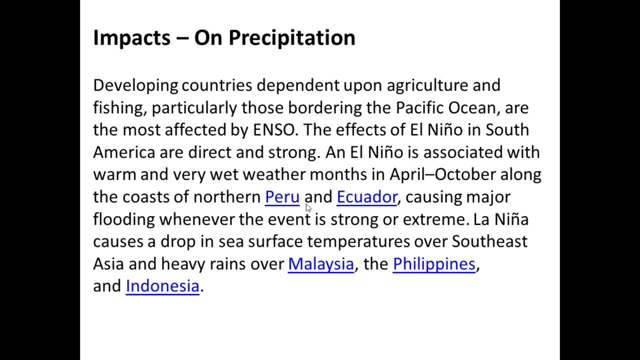 The effects of El Nino in South America are direct and strong. El Nino is associated with warm and wet weather months. in April to October. along the coasts of Peru and Ecuador You get major flooding. La Nina causes a drop in sea surface temperatures over Southeast Asia, heavy rains over Malaysia. 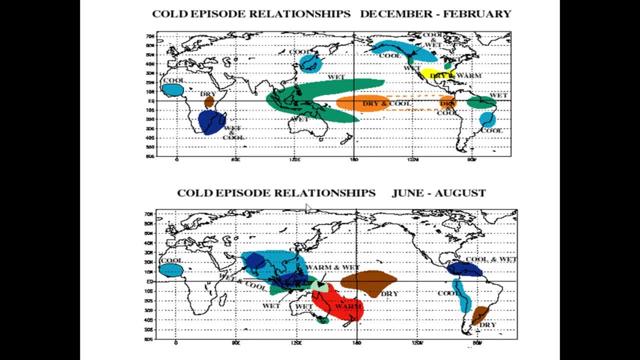 Philippines and Asia, Indonesia. So here we got some cold episode relationships: December to February, June to August And, as you can see, wet, dry, cool. Right, You can wet and cool here. We've got cooler here, cooler here. 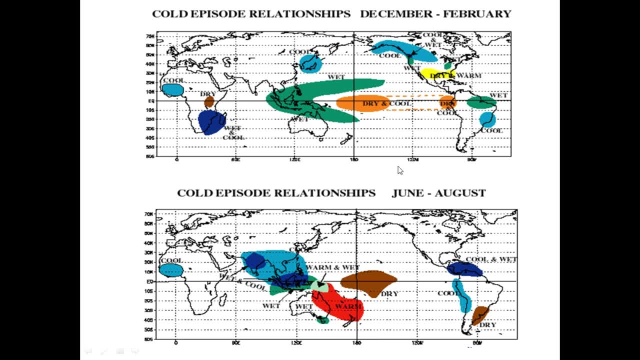 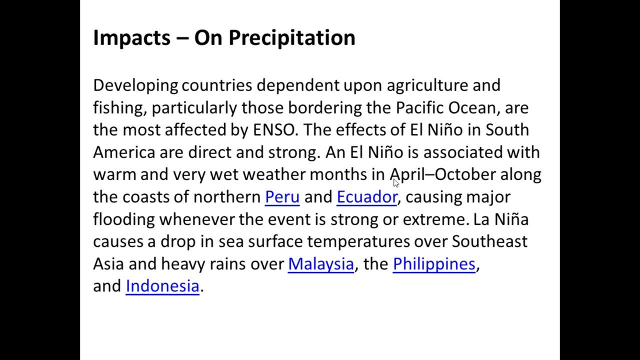 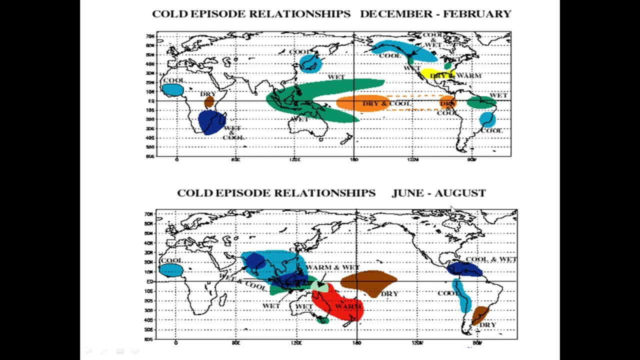 Then in June. Basically, these graphics are describing what was just here. So we've got the warm, very wet months in April to October. April to October- Well, that would include here June, August. So it misses. Don't have April, May. 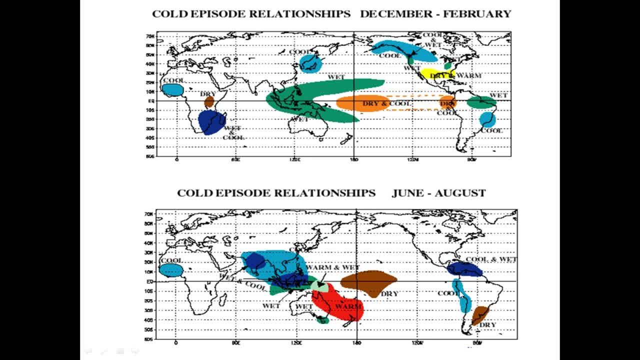 You don't have September, October, But you can see it's cool And it's going to be cool. It's going to be wet. You can see here. So you can see how this is, of course, over a year. 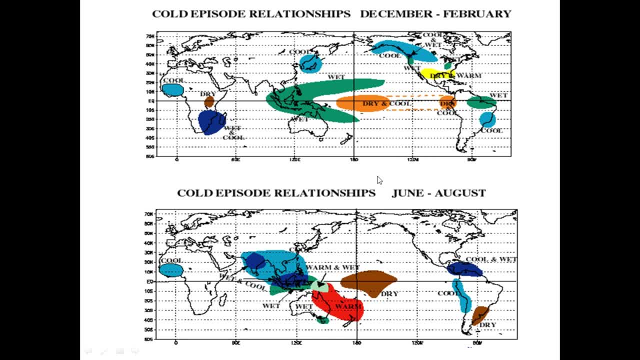 December, January, February. Now along the equator You're not going to have the extreme seasonality that you would in temperate and sub-Arctic latitudes, But still nevertheless it's going to be. the insulation received from the sun will change. 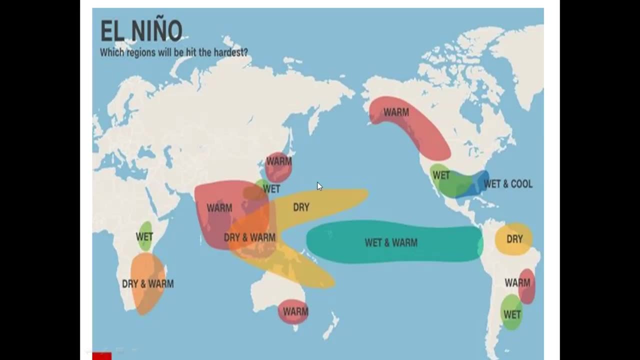 So it will affect things. Okay. So let's look at El Nino. What happens El Nino? Warm, dry, warm dry. It's warm. this way, It's wet and warm. It's warm. over here It becomes warmer, like up into Alaska. 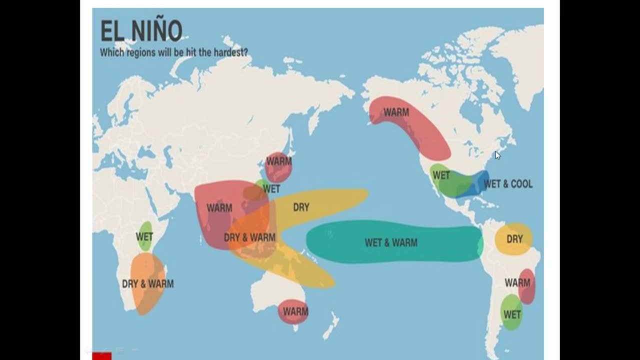 Southwest gets wet, Southeast gets cool. This is wet and cool of the US. Dry, warm, wet, etc. Dry and warm in southeastern Africa. Australia tends to be hit with warm, dry conditions And now, with climate change and the heating becoming more pronounced, they're getting. 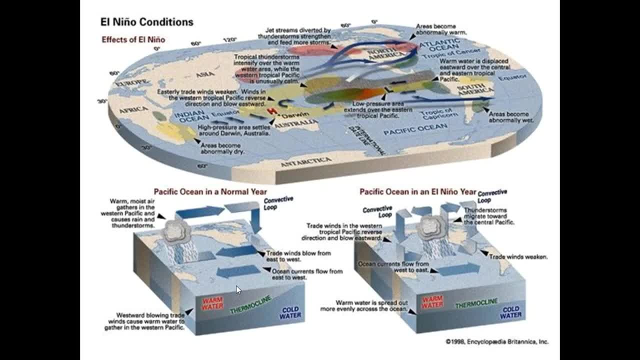 hit with drought conditions. Okay, All right. This is a very detailed map showing graphic, showing you what's going on. Areas become abnormally warm, Jet streams diverted by thunderstorm, Tropical thunderstorms intensify. You got a high pressure here, a low pressure here. 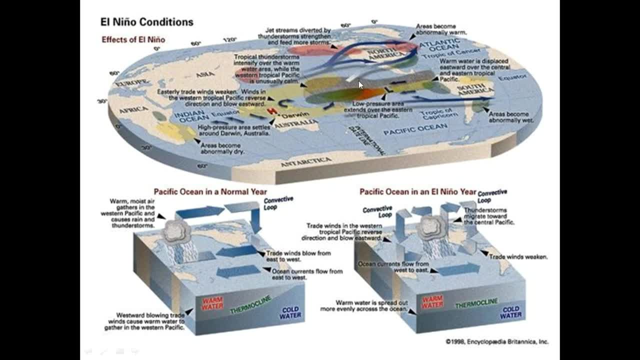 Because, don't forget, the low pressure during El Nino shifts to the east, leaving us with a high pressure here During La Nina, that low pressure system shifts back to the west. I showed you those graphics earlier where the high and lows alternate. 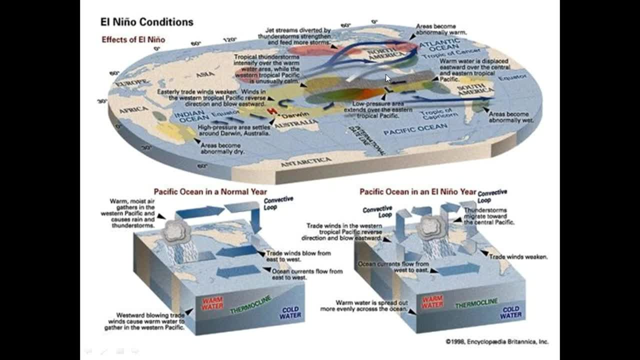 So during El Nino, that low pressure system goes to the east, leaving a high pressure system over this region of the planet, And then the reverse during La Nina. So this is the international date line here. This is the international date line here. 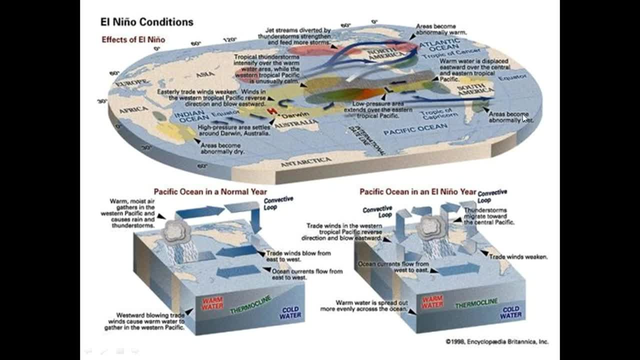 The low pressure area Extends over the eastern tropical Pacific. Air has become abnormally wet. And then we're looking at the convective loops. Thunderstorms migrate to the central Pacific. El Nino warm water Thermal climb is depressed. 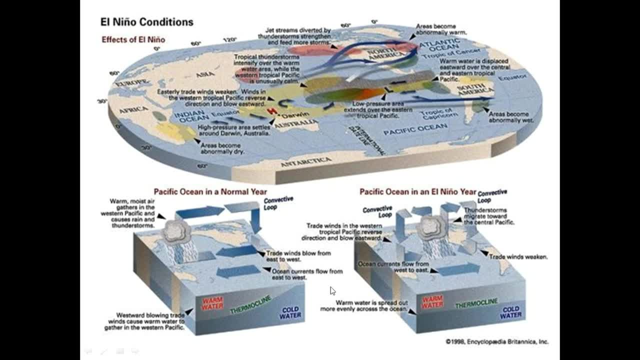 So no upwelling Cold water down below Normal year. we can see the thermal climb slanting upward, bringing cold weather Again. here's that low pressure system. That's to the west, But in El Nino it shifts to the east. 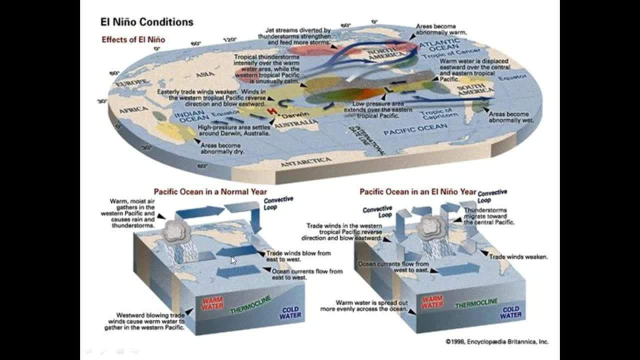 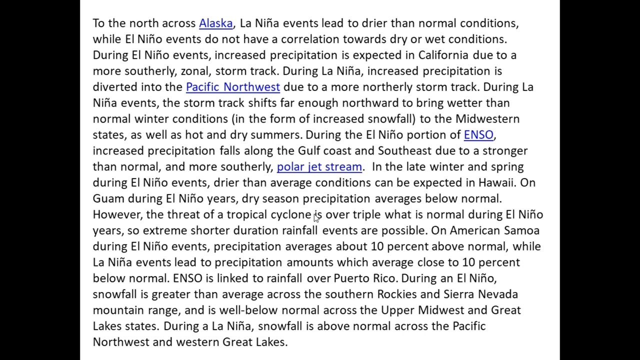 Don't forget. look at the winds. The winds shift in direction as well, Mainly driven by the convection cells, And you can always pause these to ruminate and examine these more closely And, in Alaska, La Nina, eventually to dry to normal condition, but you freeze your ass off. 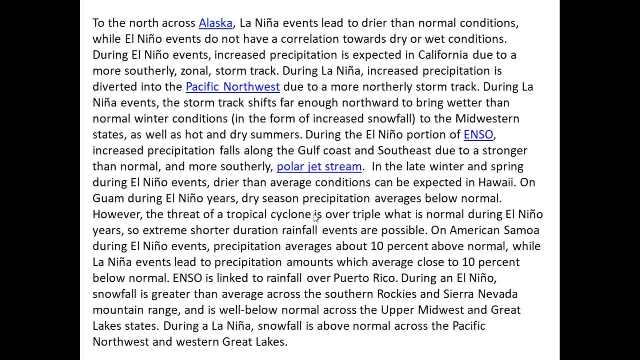 Well, at least it used to. El Nino: events do not have a correlation towards dry or wet conditions, But it does tend to be a little warmer. El Nino: increased precipitation expected in California due to a more southerly zonal storm track. 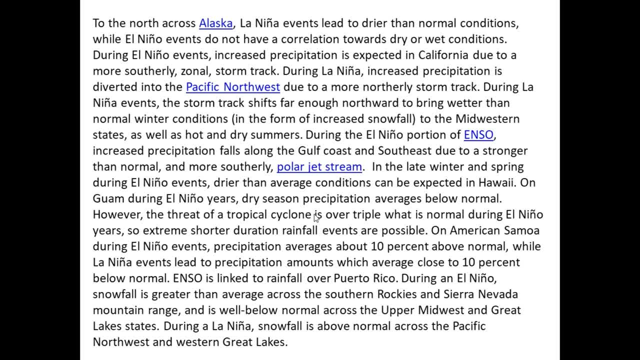 La Nina. increased precipitation is diverted into the Pacific Northwest due to more northerly storm track. La Nina events: the storm track shifts far enough northward to bring wetter than normal condition, ie more snowfall, to Midwestern states. 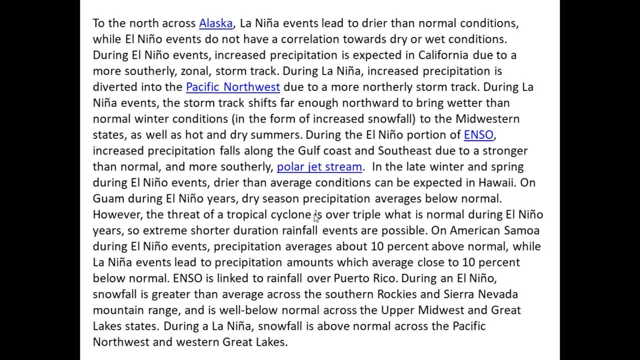 And you get hot and dry summers to go along with that. During El Nino, increased precipitation along the gulf coast and southeast due to a stronger than normal and more subtly polar jet stream Which, as it shows, is tied into the North Atlantic Oscillation. 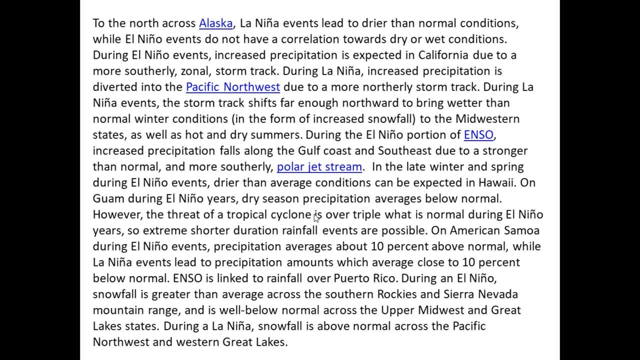 Late winter and spring. during El Nino events. dry and average conditions expected in Hawaii And on Guam during El Nino years. dry season precipitation average is below normal. The threat of tropical cyclone is over triple what is normal during El Nino years. 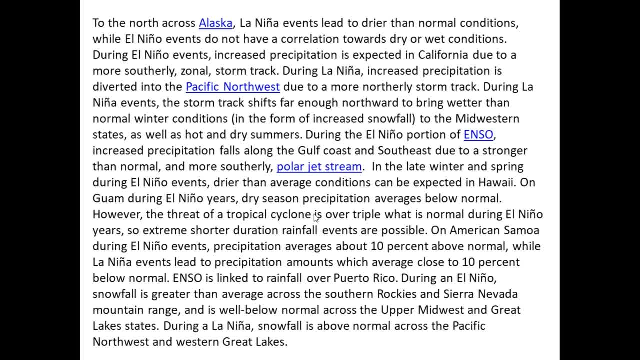 So extreme, short of duration rainfall events are possible, but more severe, And so it's linked to rainfall of Puerto Rico And so El Nino. we have snowfalls greater than average across the Southern Rockies and Sierra Nevada, well below normal across the upper Midwest. 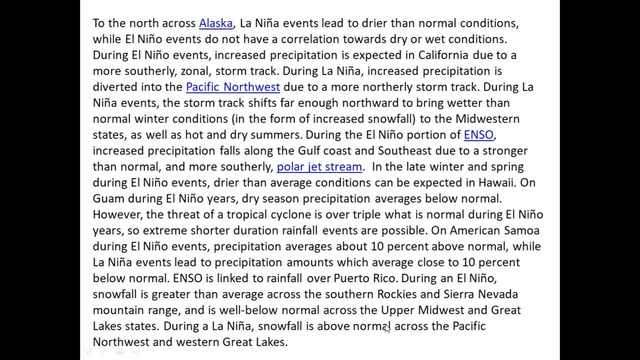 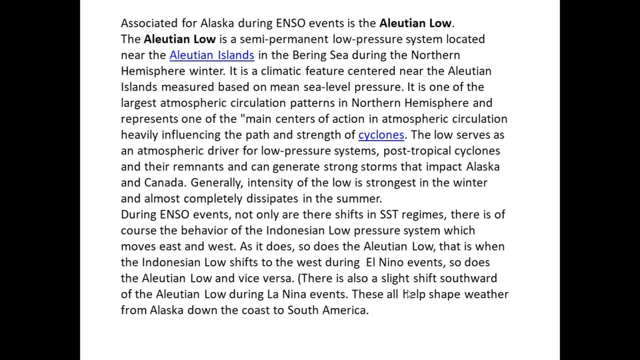 and Great Lakes state. During La Nina, snow falls above normal across the Pacific Northwest and Western Great Lakes. Associated for Alaska during ENSO event is the Aleutian Low, which is associated, as we'll discuss, with the PDO. Aleutian Low is a semi-permanent low pressure system. 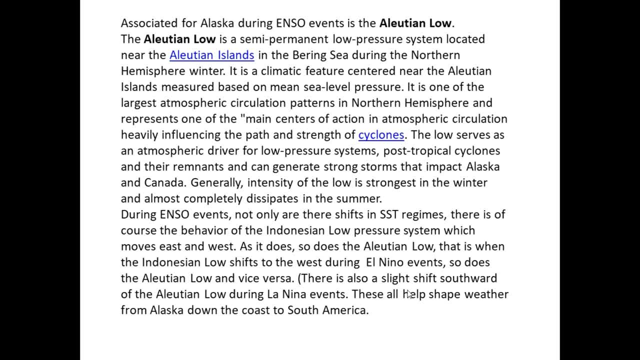 located near the Aleutian Islands, hence the name, in the Bering Sea during the Northern Hemisphere winter. It is a climatic feature centered near the Aleutian Islands, measured based on mean sea level pressure, One of the largest atmospheric circulation patterns. 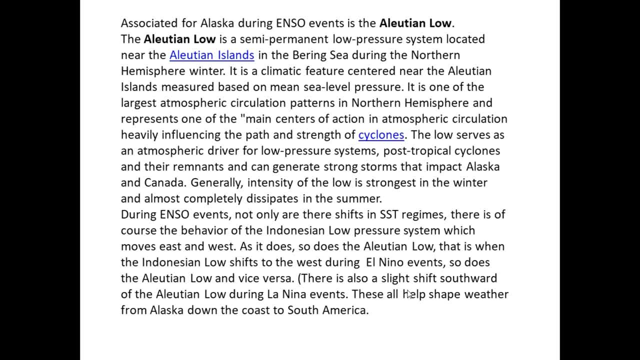 in Northern Hemisphere and represents one of the main- quote unquote- main- centers of action in atmospheric circulation, influencing the path and strength of cyclones. The low serves as an atmospheric driver for low pressure systems, post-tropical cyclones and their remnants, and can generate strong storms. 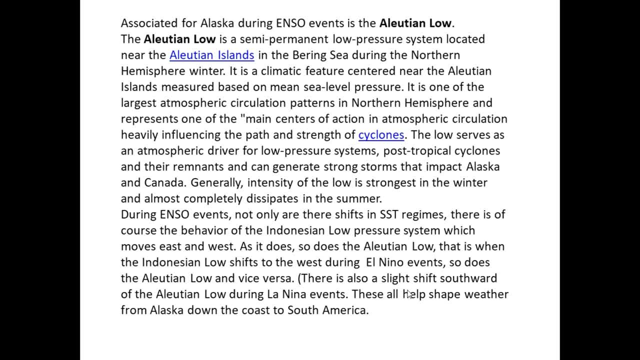 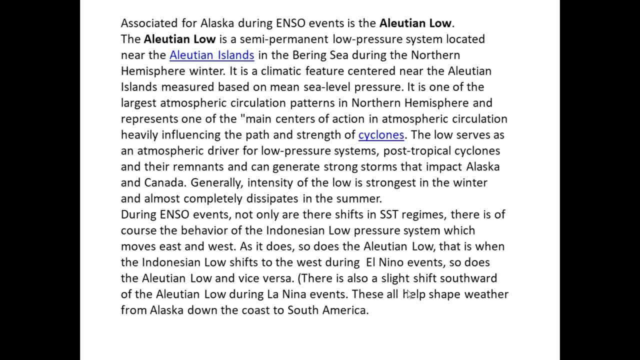 you get the shit kicked out of you. you have nothing but storms there, a whole bloody dime. Generally, intensity of the low is strongest in a winter, almost completely dissipates in the summer. During ENSO event, not only are there shifts, 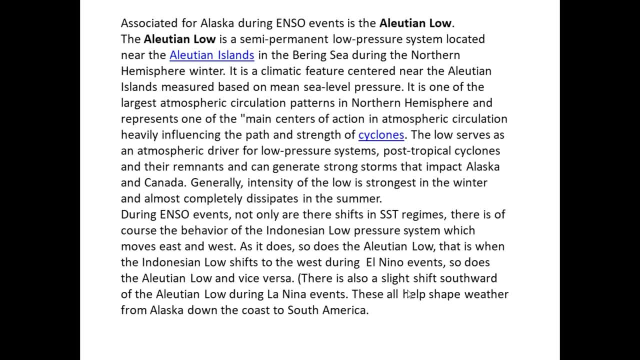 in SST regimes, sea surface temps, there's, of course, the behavior of the Indonesian low pressure system, which moves East and West, that's that the low that was featured on the graph, as it does so does the Aleutian low. so when that Indonesian system, that low, 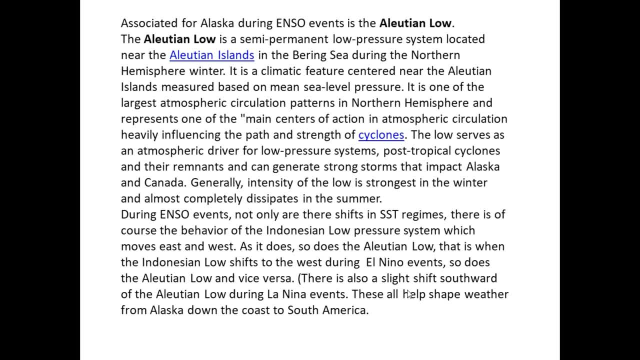 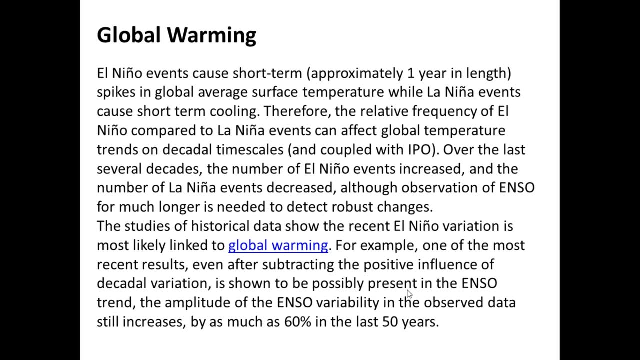 moves to the east, as does during El Nino, it pushes the Aleutian low to the east as well, and vice versa, and of course this shapes the weather. so what about global warming? El Nino events cause short term- about one year in length- spikes in global average surface. 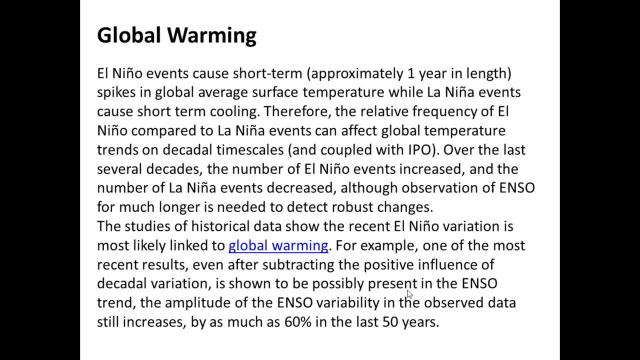 temperature on La Nina events cause short-term cooling. therefore, the relative frequency of El Nino compared to La Nina events can affect global temperature trends. on decadal timescale and coupled with the IPO into Pacific inter decadal Pacific Oscillation over the last several decades, the number of 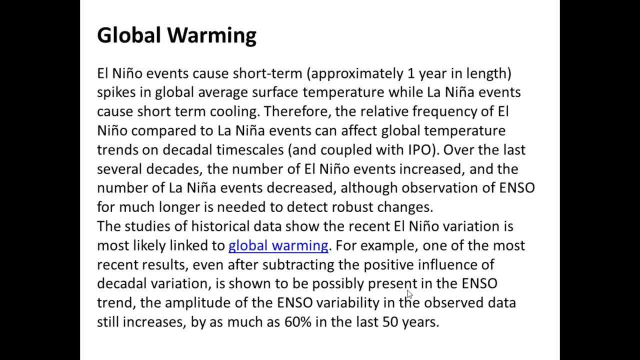 El Nino events increase and number of La Nina events decrease because we're warming the surface and that includes warming the ocean. so historical data showed a recent El Nino variation is most likely linked to global warming. for example, one of most recent results, even after subtracting 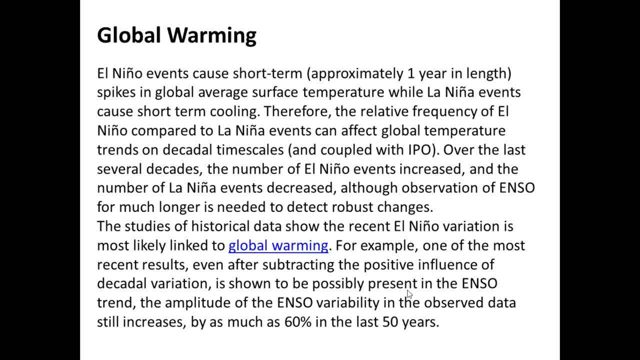 the positive influence of the Kale variation is shown to be possibly present in the n so trend. the amplitude of the n so variability observed data still increases by as much as 60% in the last 50 years. so basically, what the saying here is accounting for. 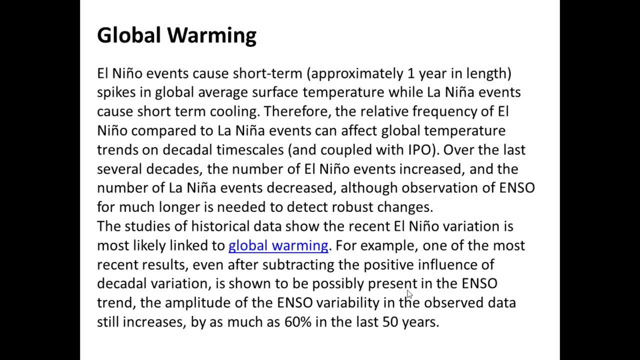 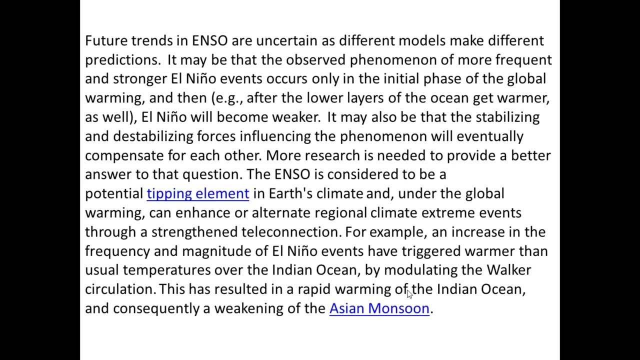 trends and other very normal variations. the resulting increase in an increase El Nino activity is basically due to global warming. that's what they're saying. they have accounted for cyclical normal variation and we're still seeing an upward trend. future trends are uncertain. different models make 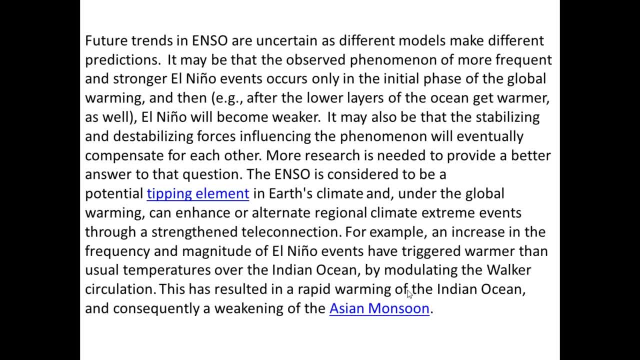 different predictions. it may be observed phenomena more frequent, stronger El Nino events occurs only in the initial phases of the global warming and then, for example after the lower layers of the ocean get warmer as well, El Nino become weaker. it may also be to stabilize and destabilizing forces. 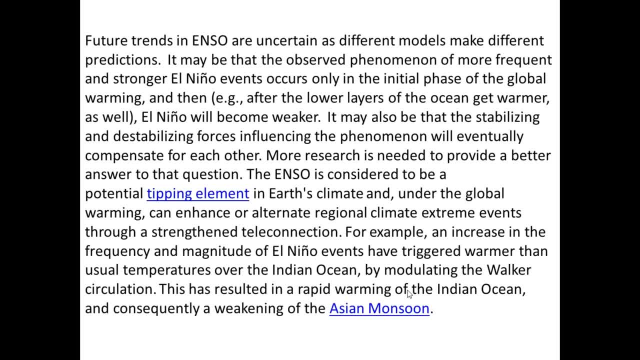 influencing the phenomena will eventually compensate for each other. more research is needed to better get a handle on it. ENSA is considered to be a potential tipping point and Earth's climate and on the global warming can enhance or alternate regional climate extreme event through a strengthened teleconnection, for example. 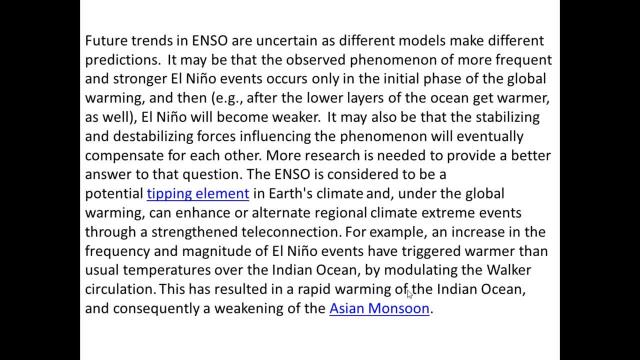 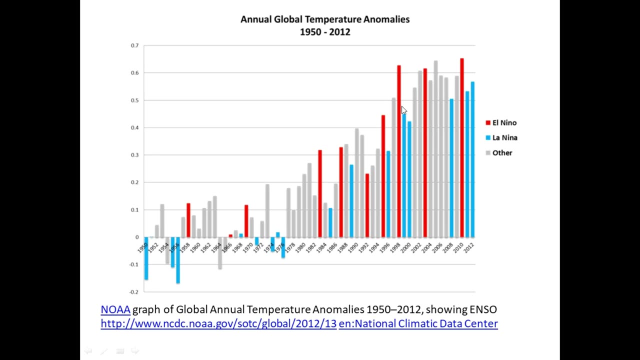 increase in frequency of magnitude. El Nino events have triggered warmer than usual temperatures over the Indian Ocean by modulating the Walker circulation. this has resulted in a rapid warming of the Indian Ocean and, consequently, a weakening of the Asian monsoon. so this is what they're talking about now. so the red bars are El Nino, the blue is La Nina. 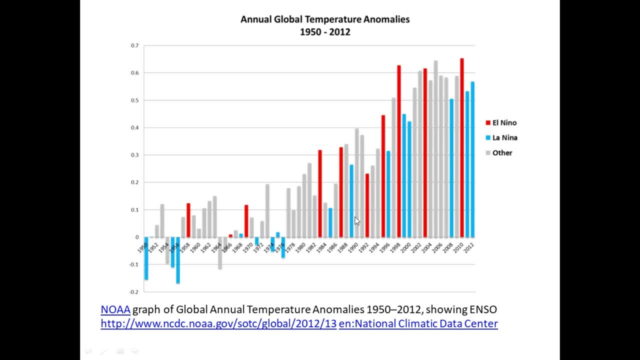 and the gray is other or neutral. this is the graph of global annual temperature anomalies from 1950 to 2012, basically 62 years, and, as you can see, look what's going on, starting from about like 1978. wow, it's just going up and up and up. in other words, 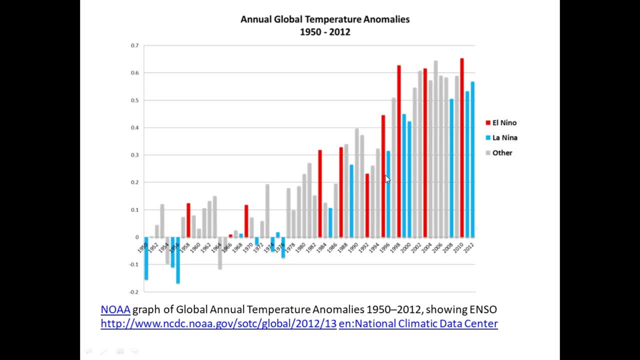 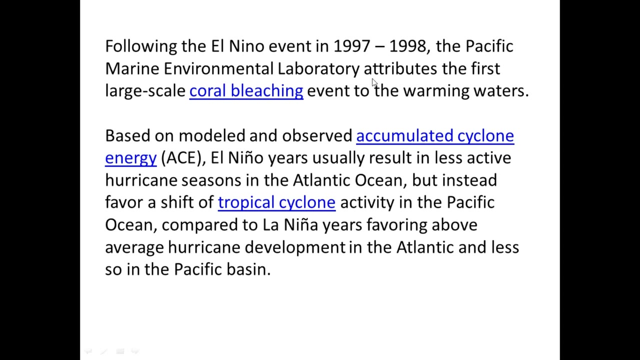 it's getting warmer. yeah, so there you have it. after. that graph is showing: following the El Nino event in 97 98, a Pacific marine environmental laboratory attributes the first large-scale coral bleaching event to the warming water. Coral bleaching is when the coral polyps die. 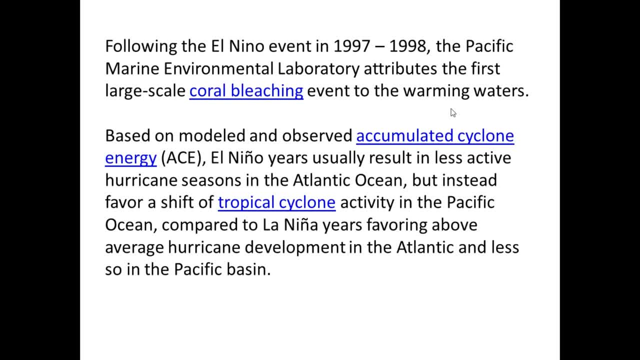 than leaving just the coral themselves, which is simply the secreted deposition of the calcium carbonate from the polyps. Well, there's no more polyps living in there, so calcium carbonate is a white mineral. So when you see white corals, those are dead corals. Based on Model Observed Accumulated Cyclone Energy- ACE. 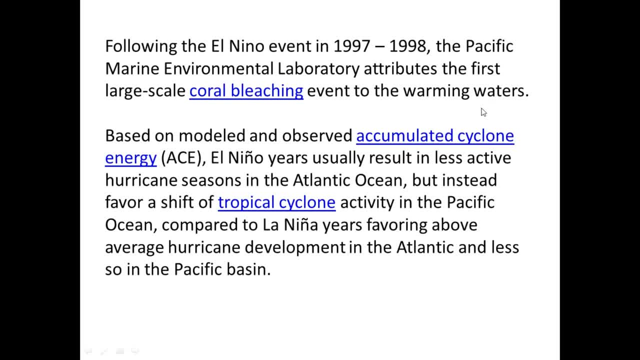 I will not be discussing. if you want me to, I can do the research for you, but it's that's a kind of a different topic altogether. Of course, it's most likely going to be related to what's going on in the atmosphere, in the ocean, but this 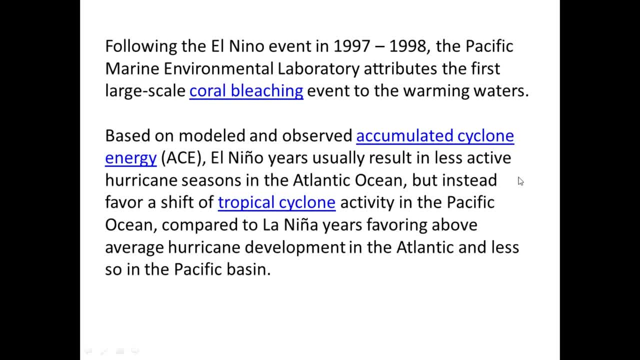 is a different topic altogether and it's really based on what the air and the oceans are doing. El Nino years usually result in less active hurricane season in the Atlantic Ocean, but instead favor shift the tropical cyclone activity in the Pacific, Compared to La Nina years, favoring above average hurricane development in the 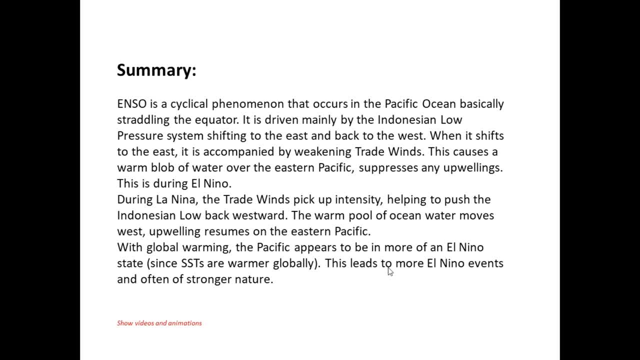 Atlantic and less so in the Pacific. So, summary, Here's a little note myself. ENSO is a cyclical phenomenon that occurs in the Pacific Ocean, basically straddling the equator. It is driven mainly by the Indonesian Lod Thevan moves southwijc into the Pacific, facing the Pacific Ocean. 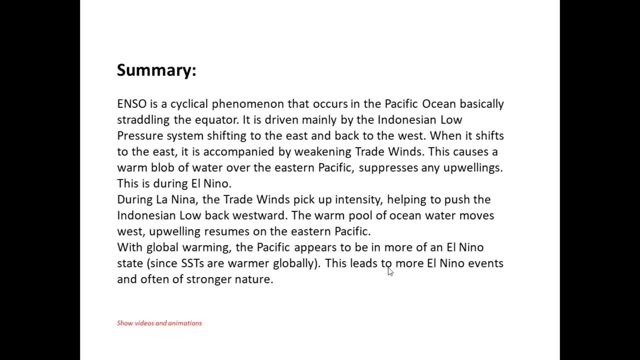 There is a low pressure system shifting to the east and back to the west. When it shifts to the east is accompanied by weakening trade winds. This causes a warm blob- that's a nice technical term- warm blob of water over the eastern Pacific, suppressing 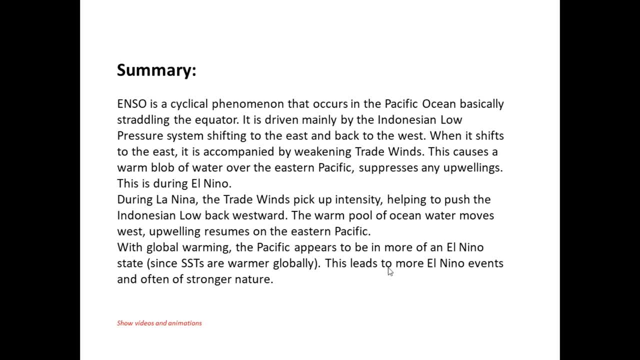 any upwelling, that's during El Nino. During La Nina, the trade winds pick up intensity, pushing the Indonesian Lod back westward. The warm pool of water also moves west, Upwelling Since SSTs are warmer globally. this leads to more El Niño events and often of stronger 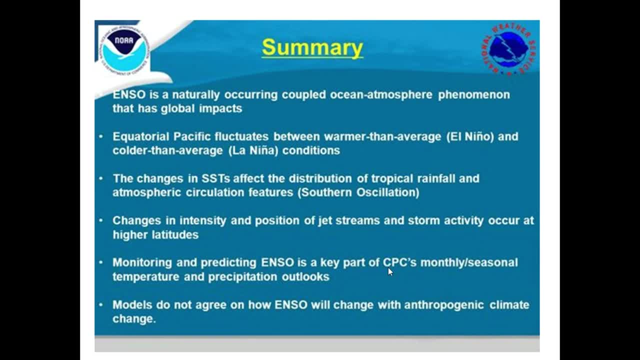 nature. Here is a summary from NOAA. Coupled ocean-atmosphere phenomenon fluctuates between warmer-than-average El Niño, colder-than-average La Niña conditions. The changes in SSTs affect the distribution of tropical rainfall and atmospheric circulation features. Changes in intensity and position of the jet streams, and storm activity occur at higher. 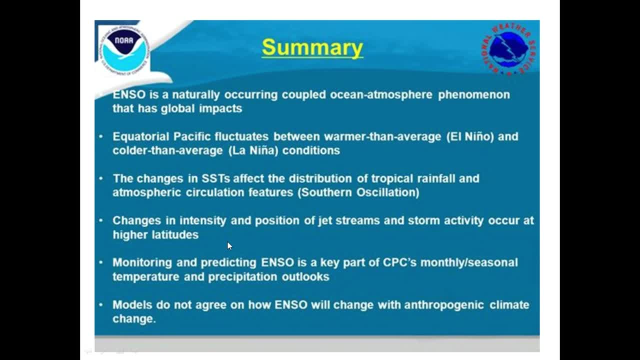 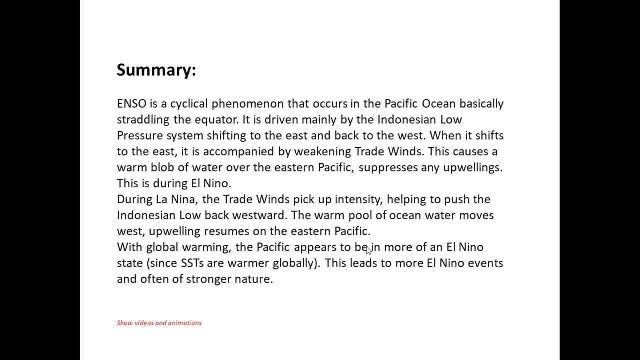 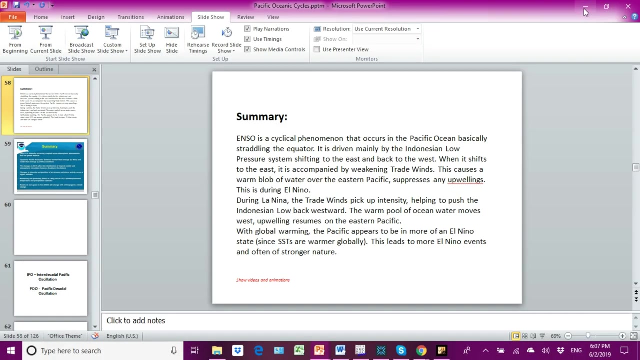 latitudes. Monitoring and predicting ENSO is a key part of the CPC Models. do not agree on how ENSO will change with anthropogenic climate change. Yeah, that's what you call doing research. So let me know. I think I have some little videos queued up here. 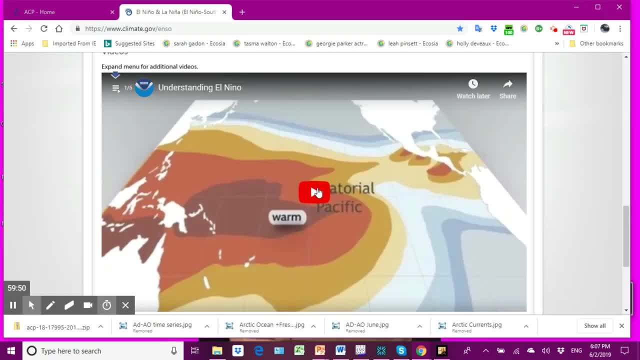 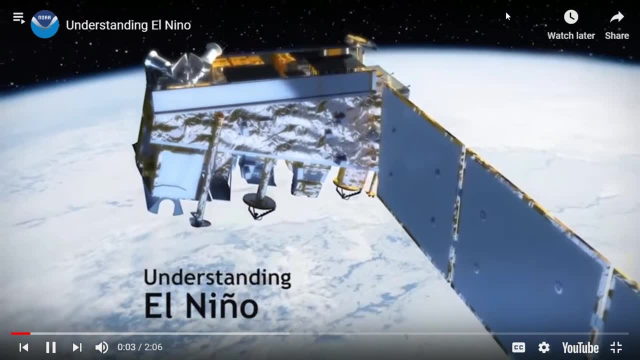 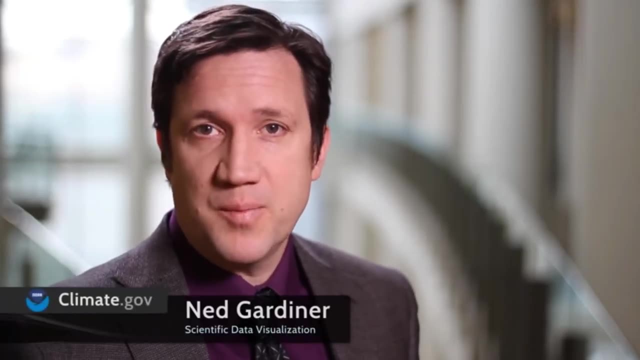 Let me get to that. you know. let's go right here. El Niño is the warm water phase of the El Niño Southern Oscillation, the most influential climate pattern used in seasonal forecasting during El Niño ocean temperatures over the Pacific. 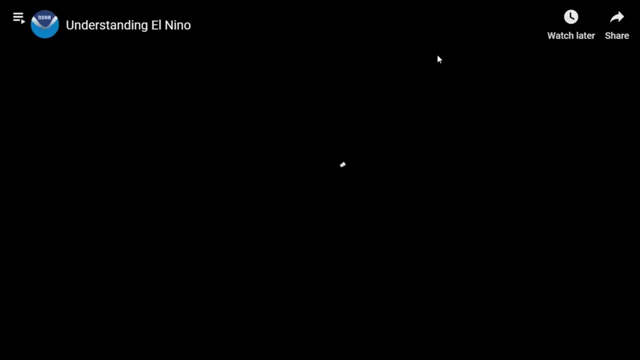 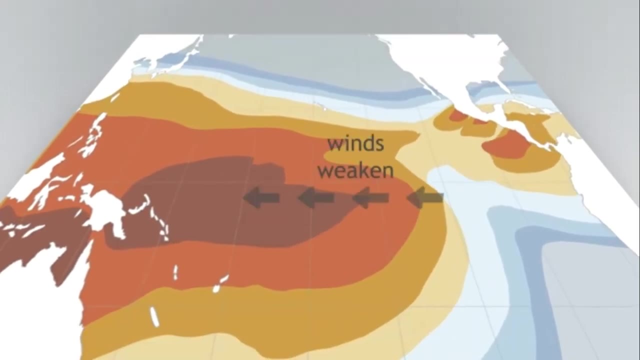 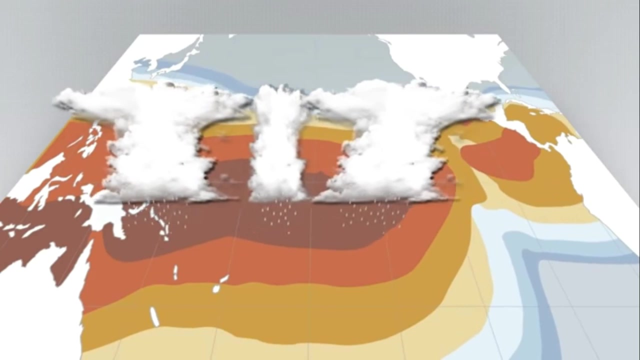 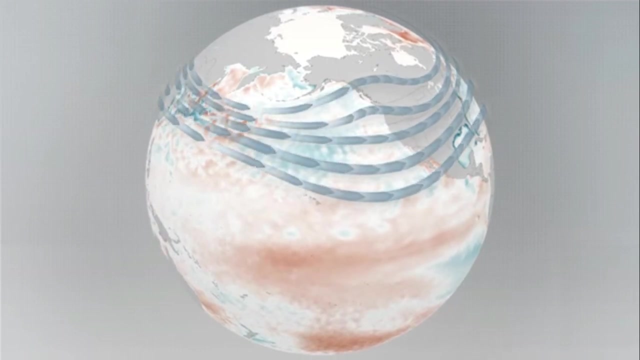 It is the most important time of the year for the Pacific to begin to warm up. Surface winds weaken and rainfall increases over the Central or Eastern Pacific, while decreasing over Indonesia. Warmer oceanic and atmospheric conditions in the Central and Eastern Pacific fuel the 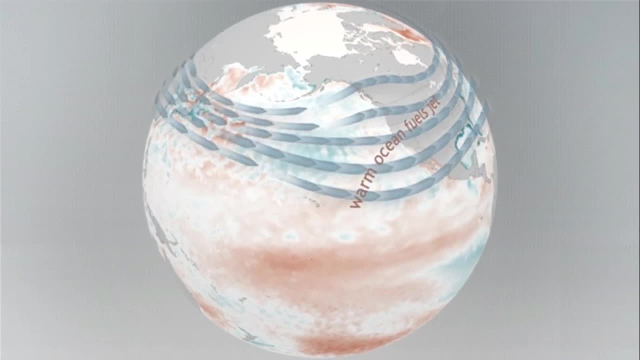 jet stream. Because the Central and Eastern Pacific is warmer than the Central and Eastern Pacific, the jet stream is less likely to be affected. The central and eastern Pacific is warmer than the Central and Eastern Pacific And because the central Pacific is warmer than normal, during an El Niño, the jet shifts. 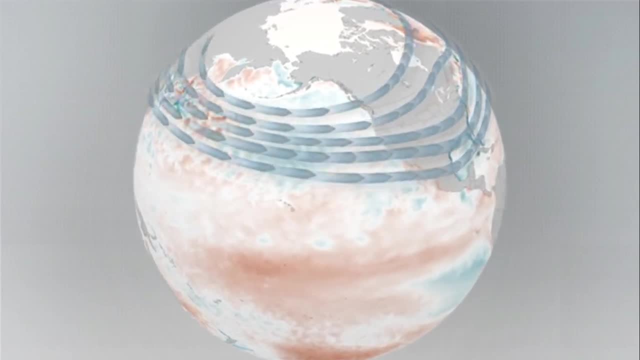 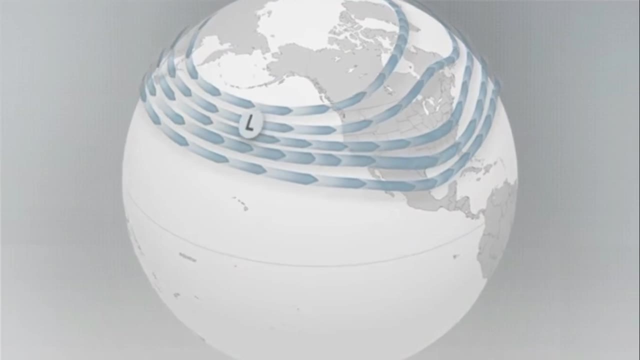 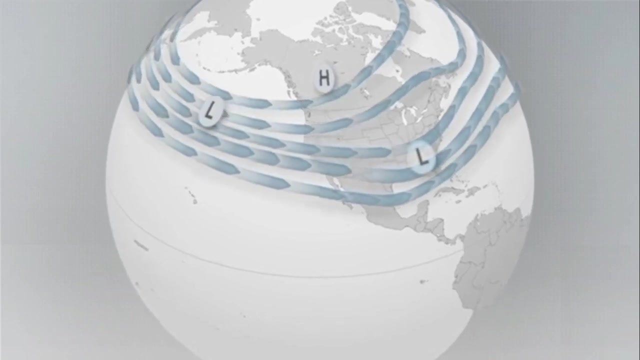 eastward. with this energy source. A stronger eastward shifted jet stream favors low pressure in the Gulf of Alaska, higher pressure over western Canada and lower pressure over the southeastern United States. This type of influence from one region to another over large parts of the globe is referred. 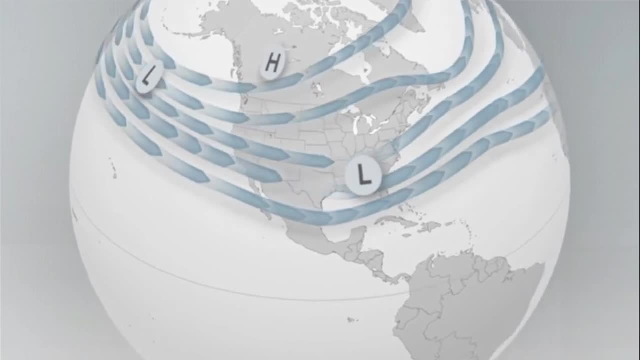 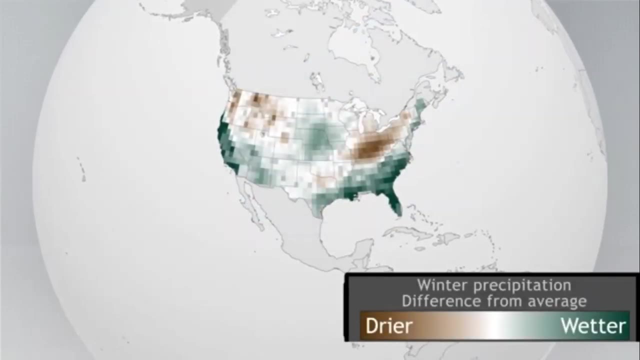 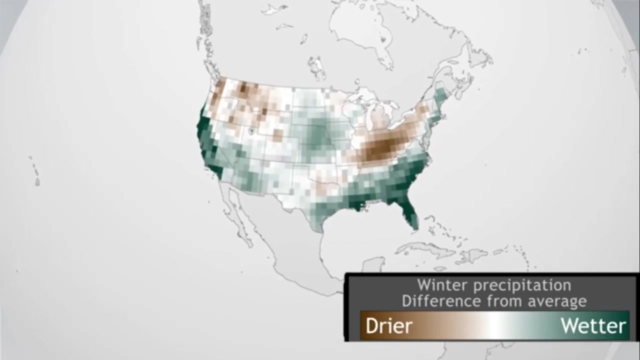 to as a teleconnection. This is the most important thing. During winter, El Niño is generally associated with wetter than average conditions across the southern tier and drier than average conditions in the Pacific Northwest, the Northern Rockies and the Ohio Valley. 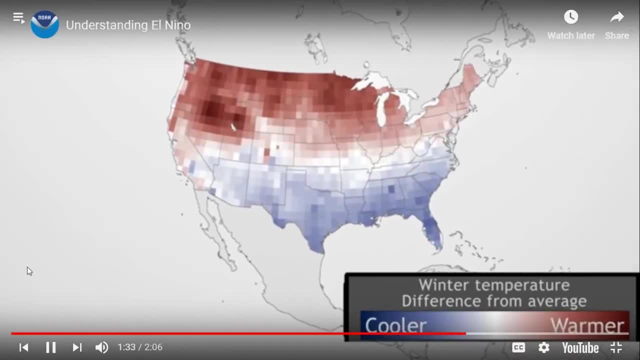 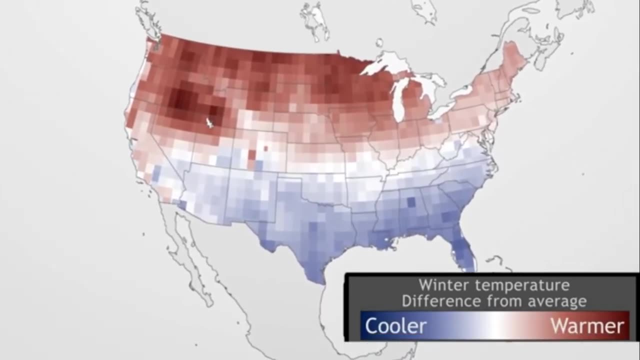 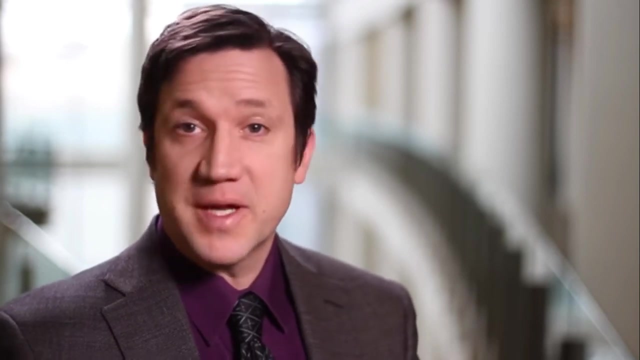 We typically observe below average temperatures across the southeastern United States and warmer than average conditions over the northern part of the country. This is the most important thing. This is the most important thing. Weather is what we experience every day, but remember climate predictions based on. 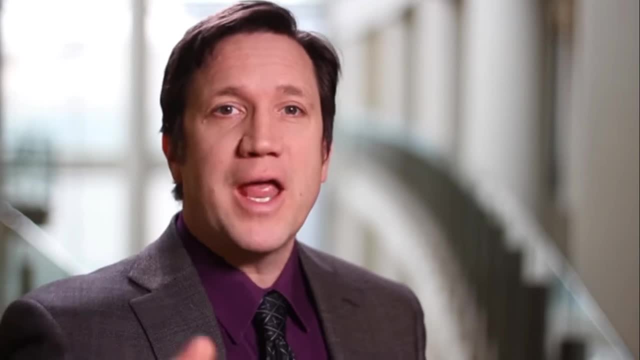 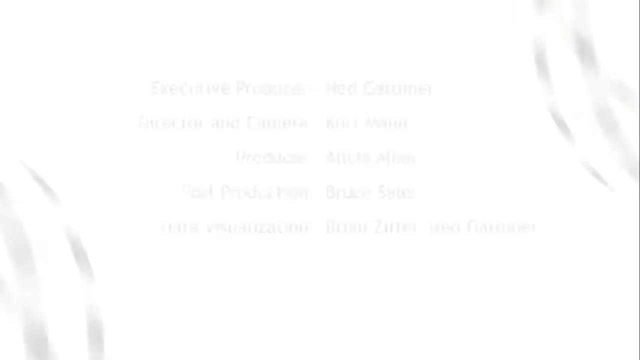 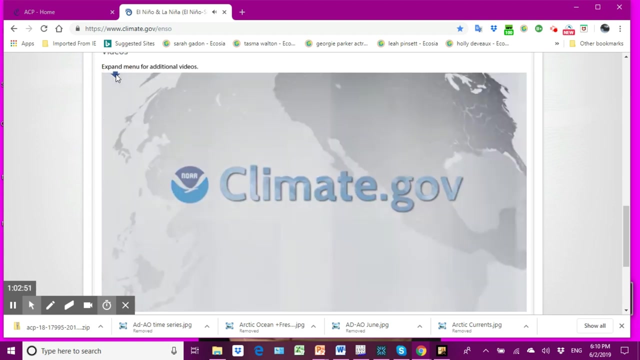 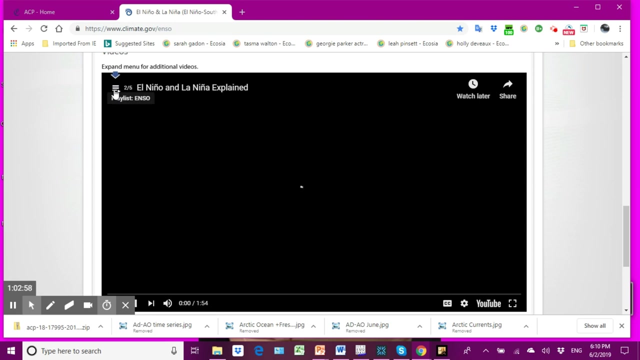 El Niño. tell us what kind of weather to expect, on average and over a long period of time From NOAA's Climate Prediction Center. I'm Ned Gardner. Thanks for watching. I'll see you next time on Climate Prediction Center. Bye for now. 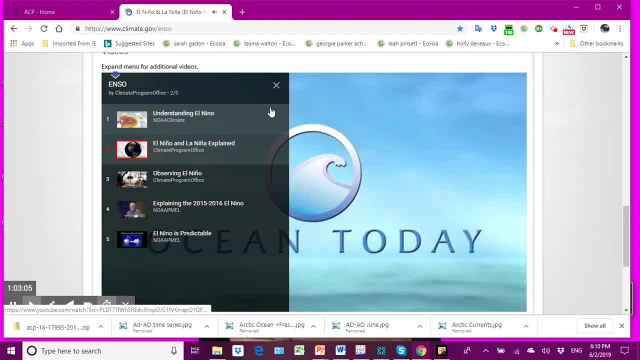 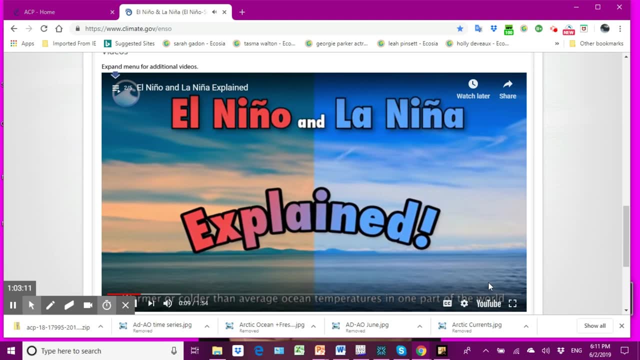 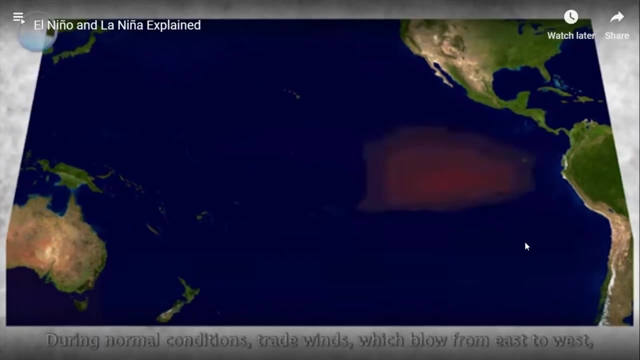 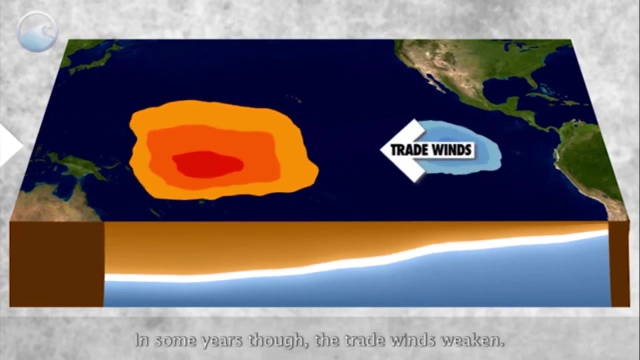 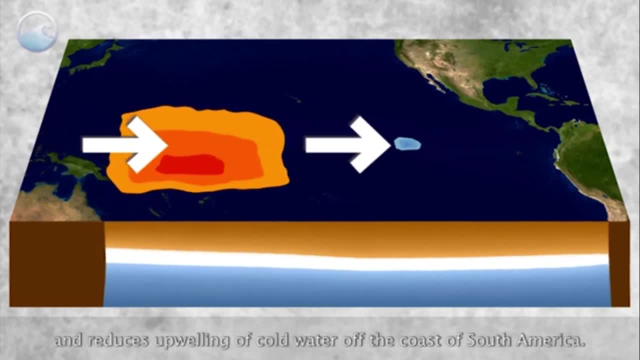 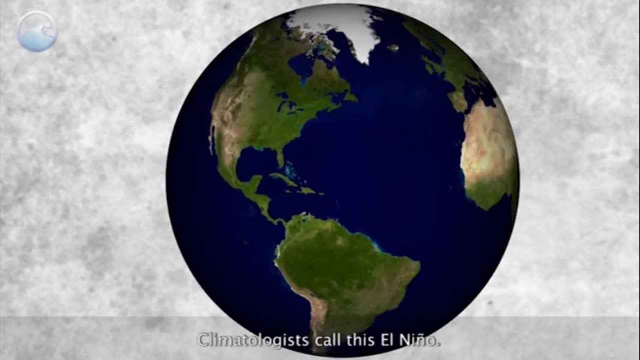 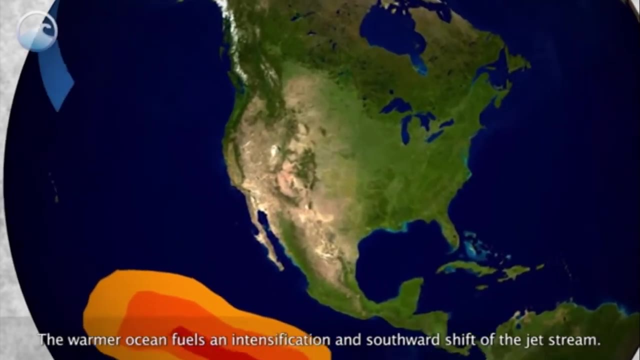 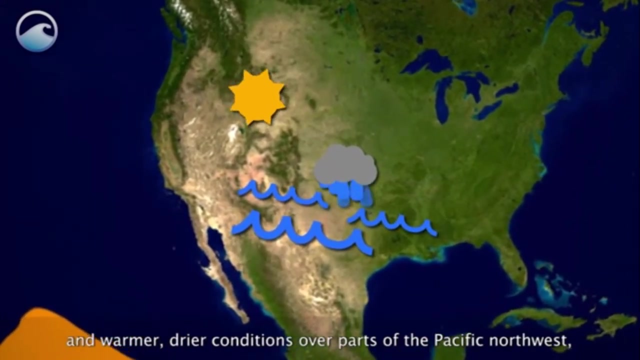 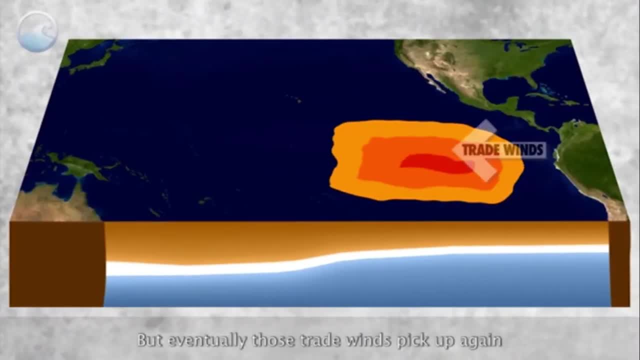 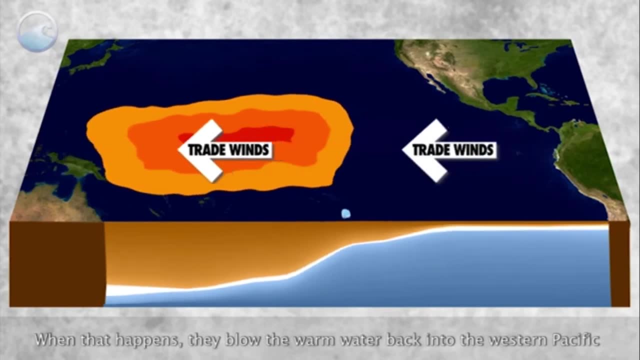 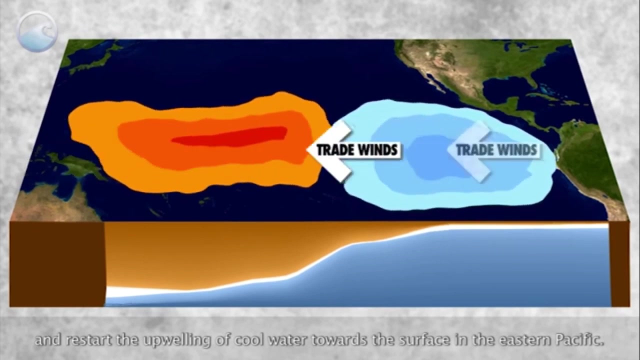 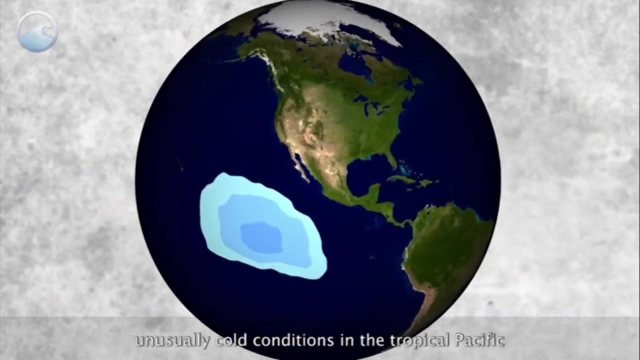 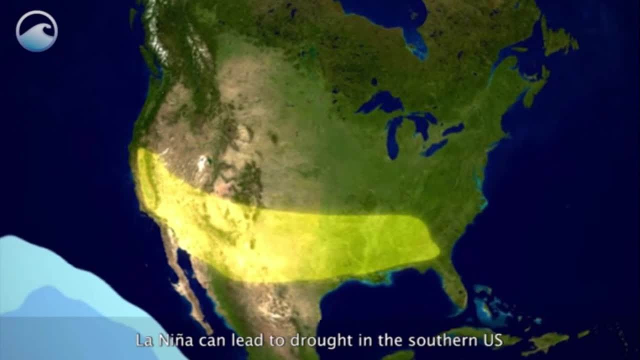 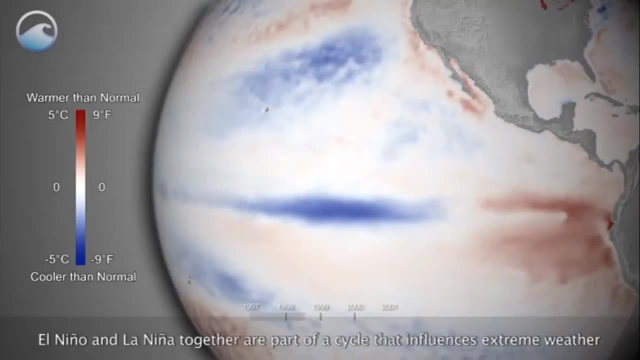 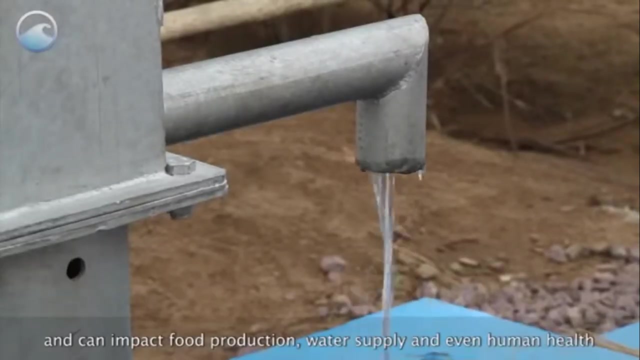 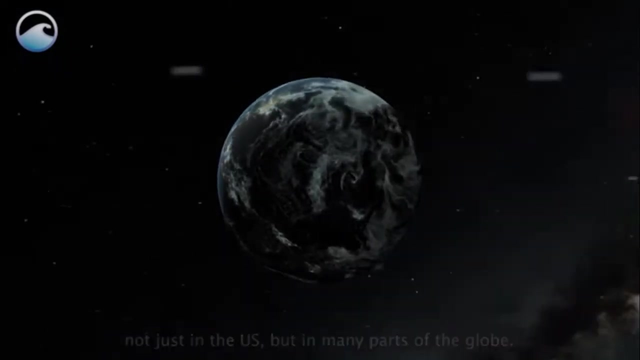 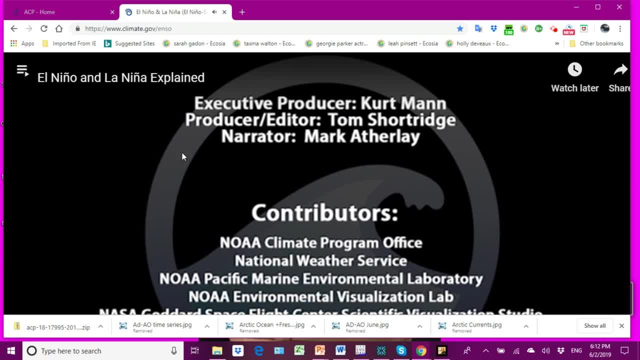 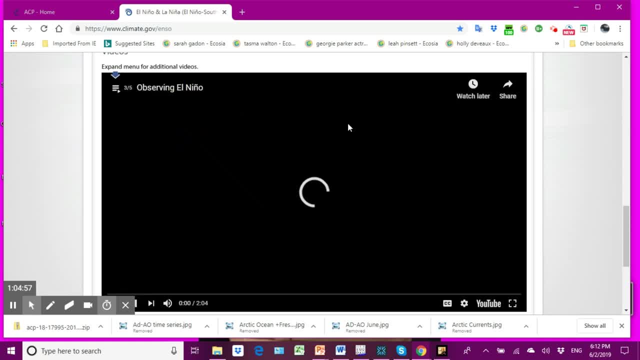 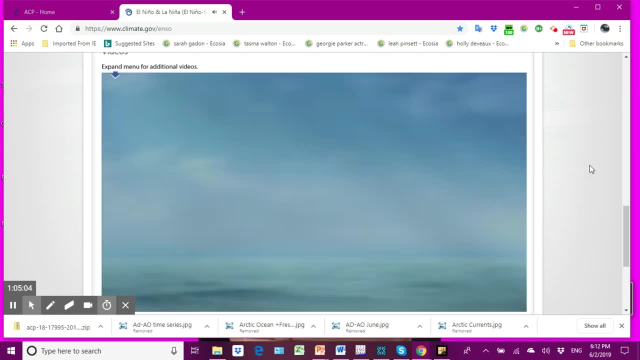 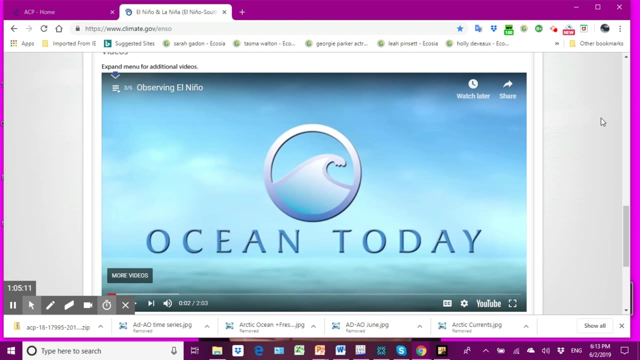 Bye, Bye, Bye, Bye, Bye, Bye, Bye. okay, well, quick, little, quick little videos there. hope you found, hope it helped pull this all together. let's see if I get myself back here. there I am, is this scary, scary sight there? let me. 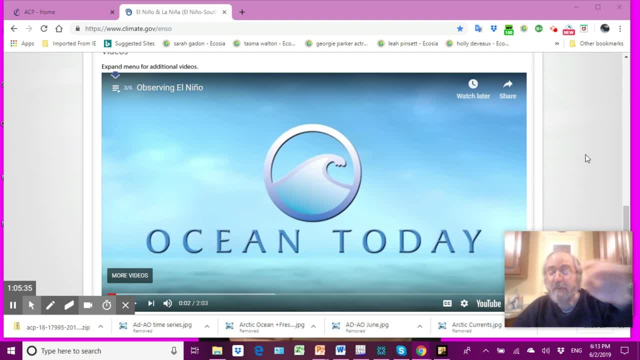 reappear anyway, so I hope you found this video informative. this is the first in a series. you vote, you know, review. watch this video as often as you'd like to. you know. pause it on those on all the graphics that I included in there to study that for the length. pull up the URLs I provided and